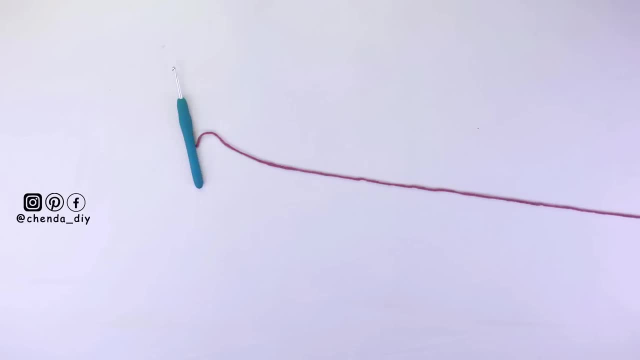 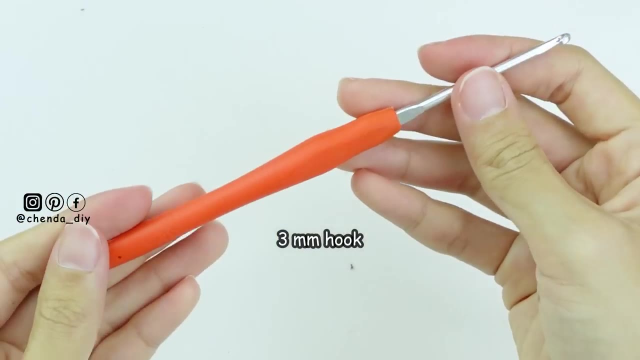 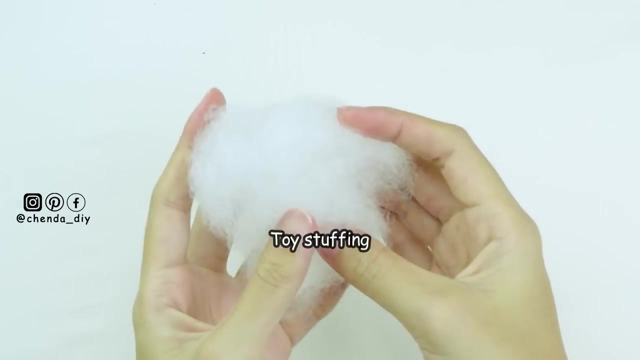 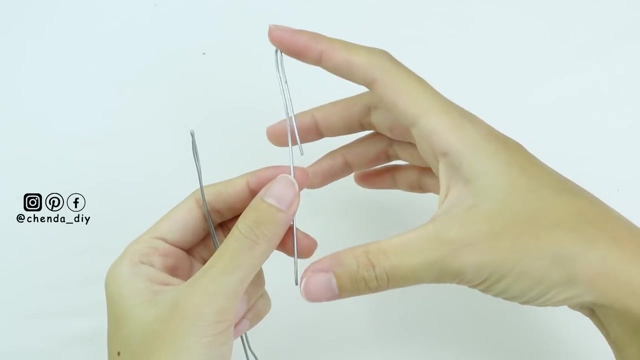 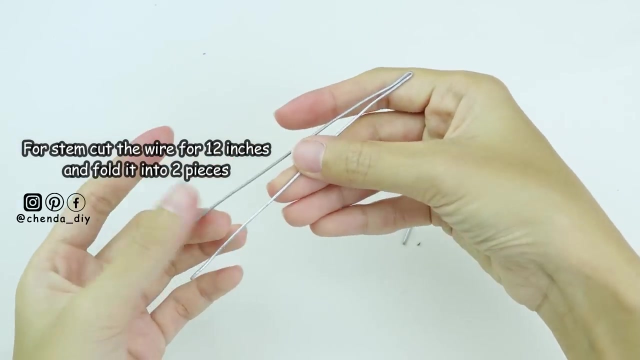 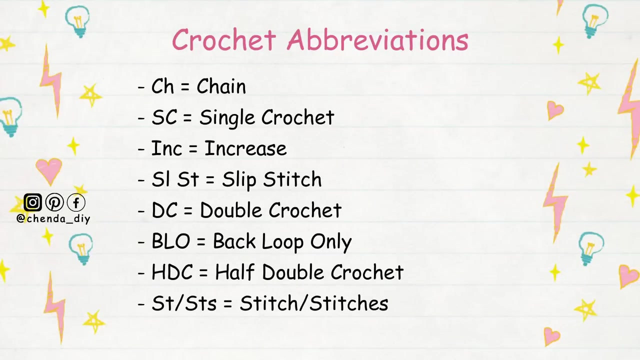 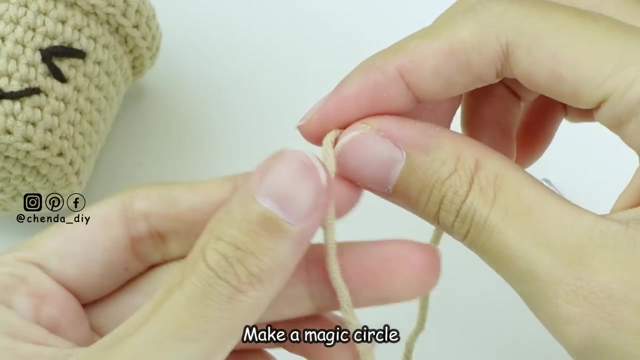 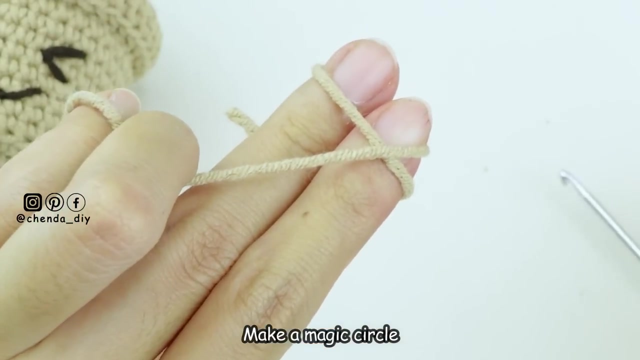 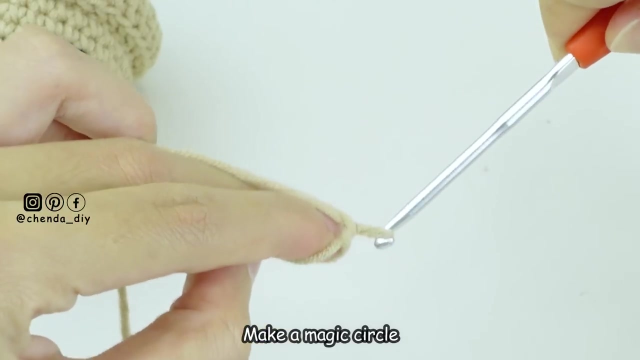 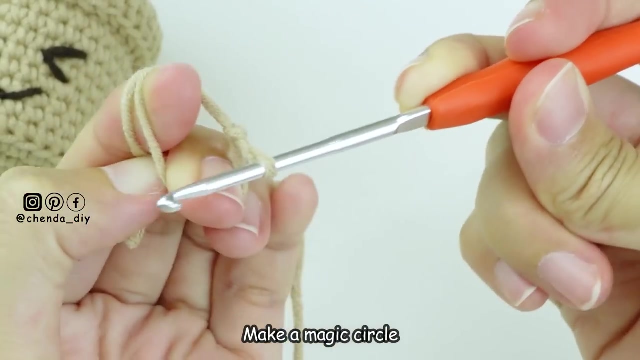 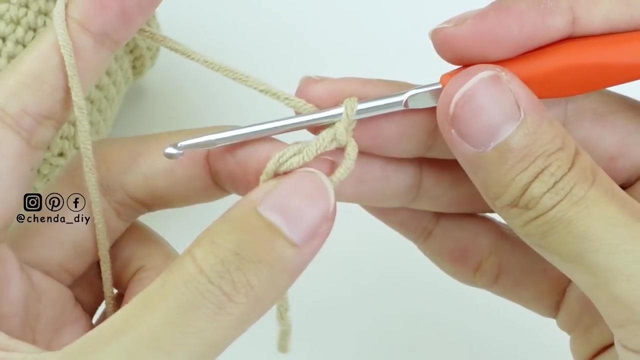 Okay, let's get into the video. Okay, let's get into the video. First thing: first we are going to make the pot To begin make a magic circle, To begin make a magic circle. And next we are going to make single crochet For row one. 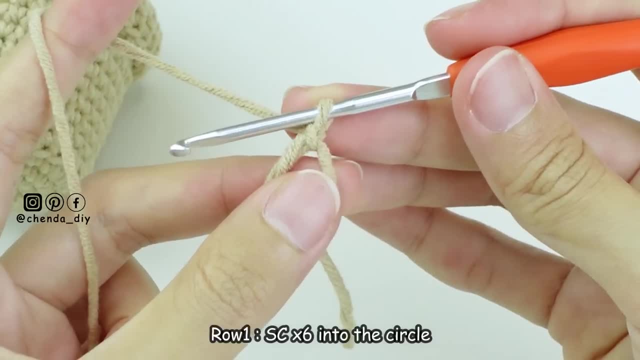 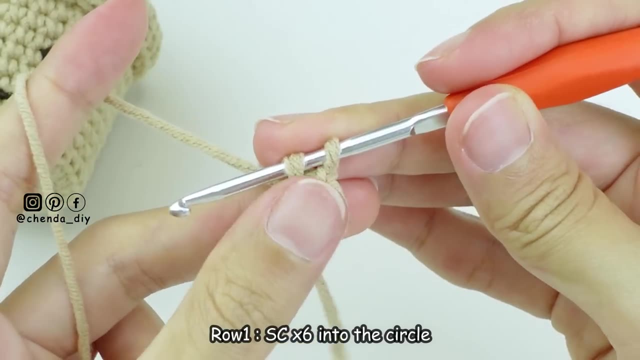 make single crochet into the circle. To make single crochet, insert the hook into the circle, Yarn over and pull up a loop. And now you have two loops on your hook. Yarn over and pull through all two loops. Don't forget to make a magic circle. 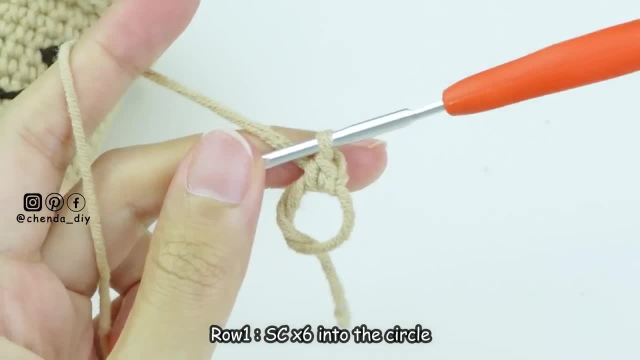 Yarn over and pull through all two loops. Don't forget to make a magic circle. Don't forget to use stitch marker to mark at this first single crochet stitch. It is where we are going to make slip stitch. at the end of the row. 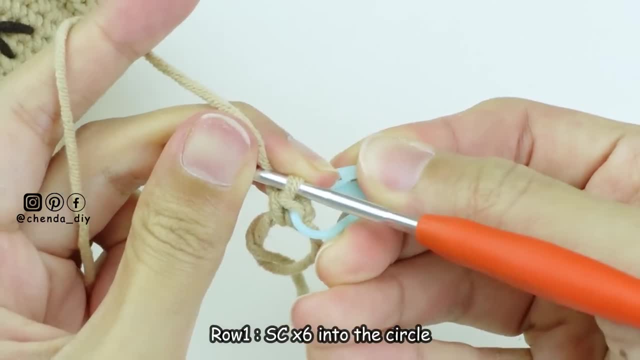 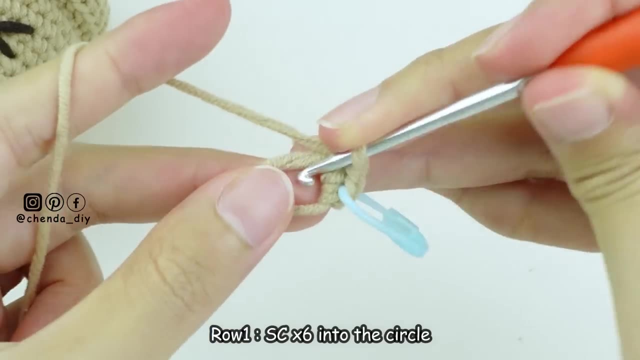 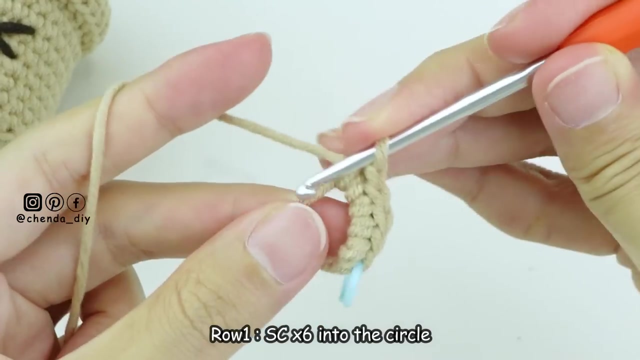 It is where we are going to make slip stitch at the end of the row. It is where we are going to make slip stitch at the end of the row. Keep making single crochet into the circle until you got six stitches of single crochet. Then I will meet you back again. 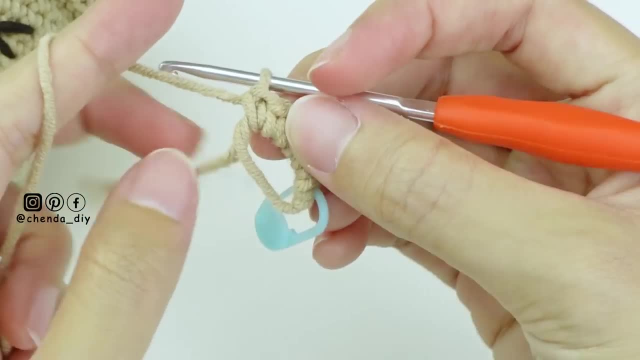 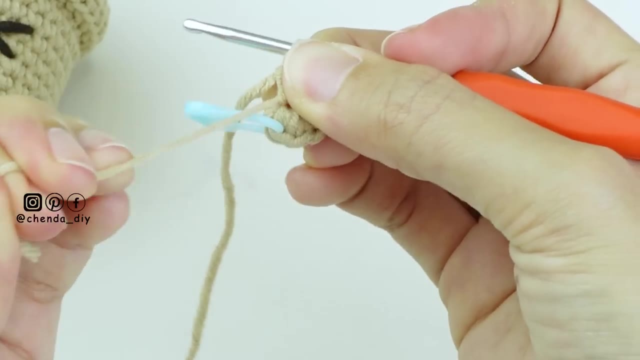 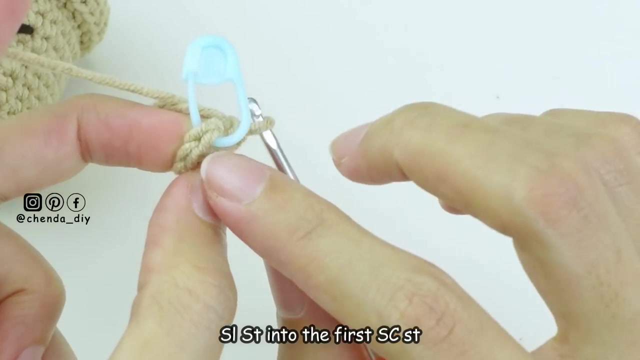 After you got six stitches of single crochet, then pull the short string of yarn tight to close the circle. Then I will meet you back again. And next we are going to make slip stitch into the stitch that we mark. And next we are going to make slip stitch into the stitch that we mark. 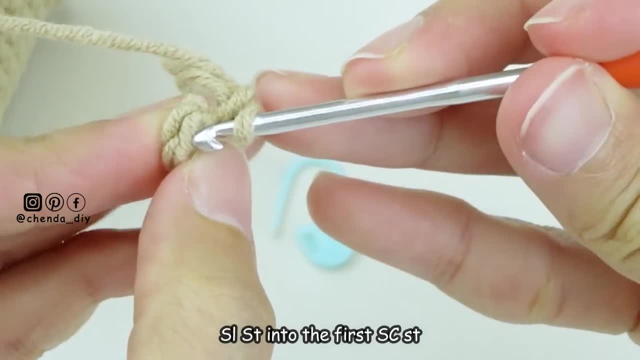 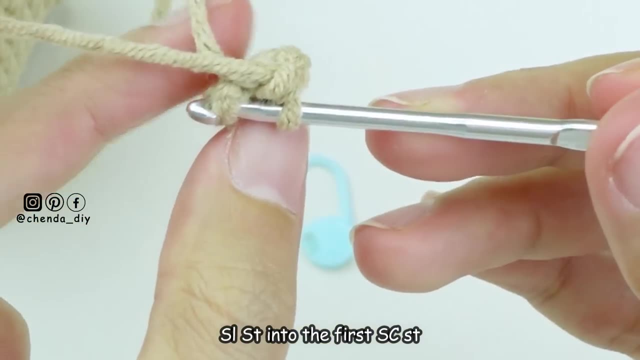 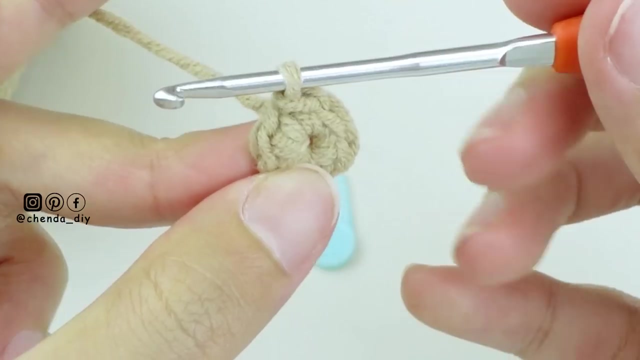 To make slip stitch continue, insert the hook into the loop. To make slip stitch continue. insert the hook into the loop. To make slip stitch continue. insert the hook into the loop. Yarn over and pull through all the loops After you have made slip stitch. next for row 2, chain 1.. 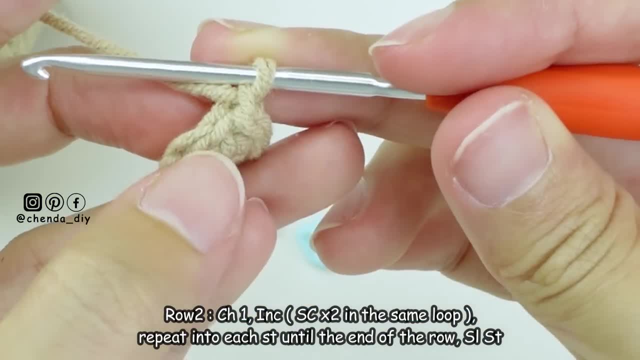 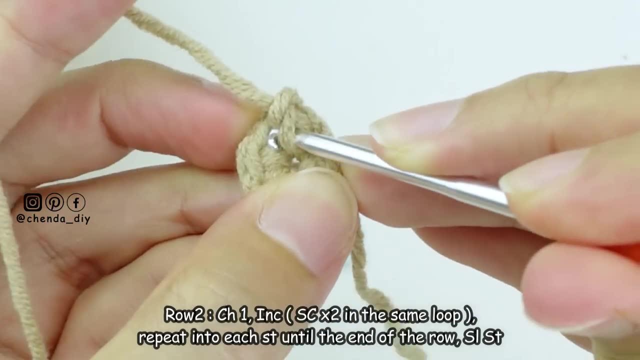 For chain 1, we don't count as a stitch. Next, we are going to make increase by making 2 single crochet into the same loop near chain 1.. Next, we are going to make increase by making 2 single crochet into the same loop near chain 1.. 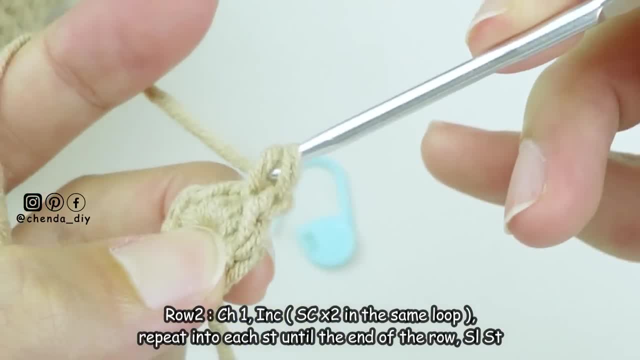 Next we are going to make increase by making 2 single crochet into the same loop near chain 1.. Don't forget to use stitch marker to mark at the first single crochet stitch. Don't forget to use stitch marker to mark at the first single crochet stitch. 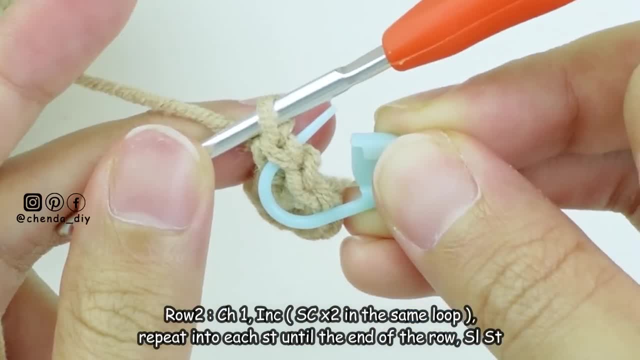 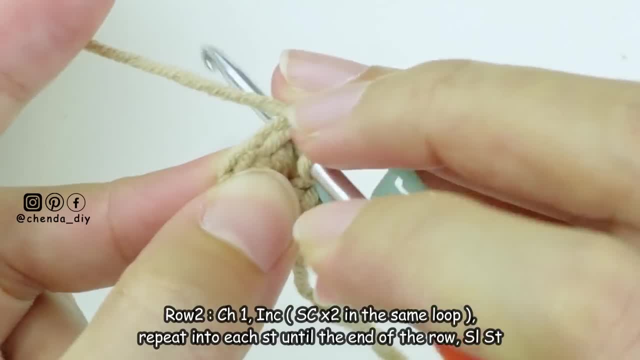 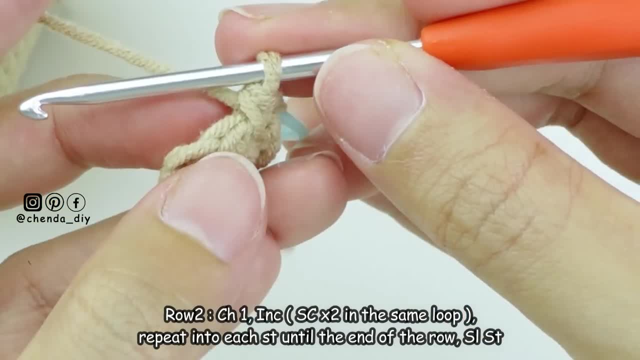 After you got 2 stitches in the same loop, then we are going to repeat the same thing by making 2 single crochet in the same loop. After you got 2 stitches in the same loop, then we are going to repeat the same thing by making 2 single crochet in the same loop. 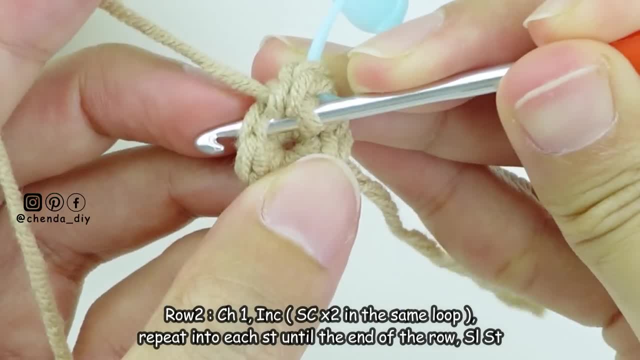 After you got 2 stitches in the same loop, then we are going to repeat the same thing by making 2 single crochet in the same loop. After you got 2 stitches in the same loop, then we are going to repeat the same thing by making 2 single crochet in the same loop. 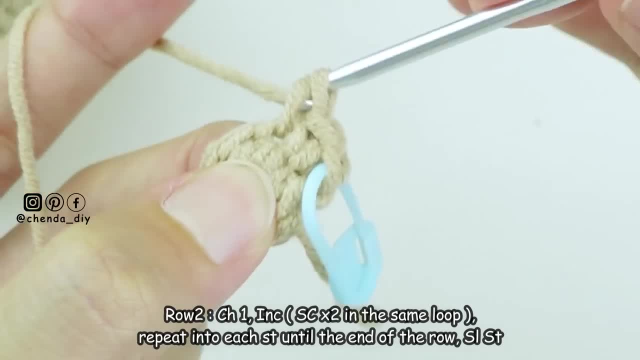 After you got 2 stitches in the same loop, then we are going to repeat the same thing by making 2 single crochet in the same loop. After you got 2 stitches in the same loop, then we are going to repeat the same thing by making 2 single crochet in the same loop. 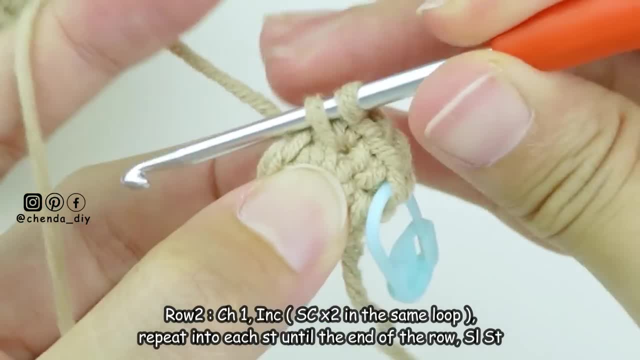 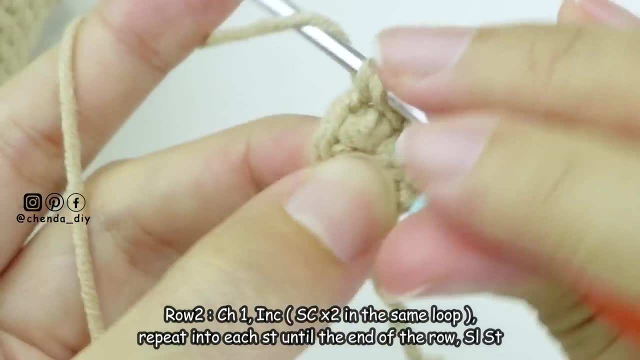 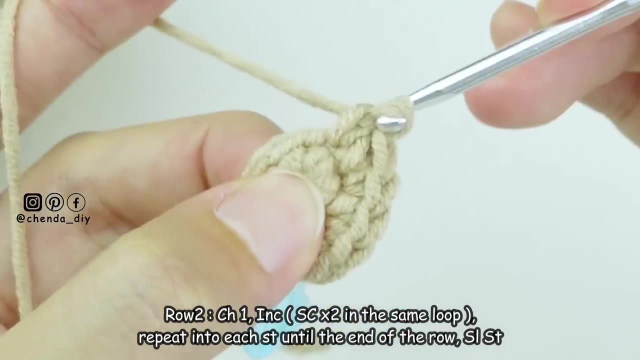 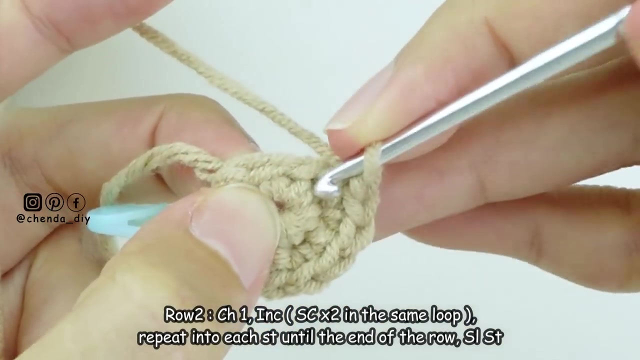 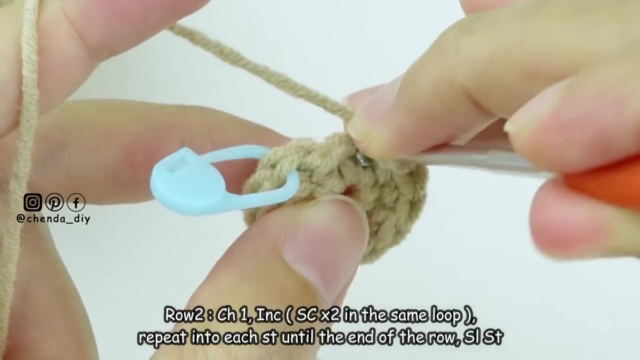 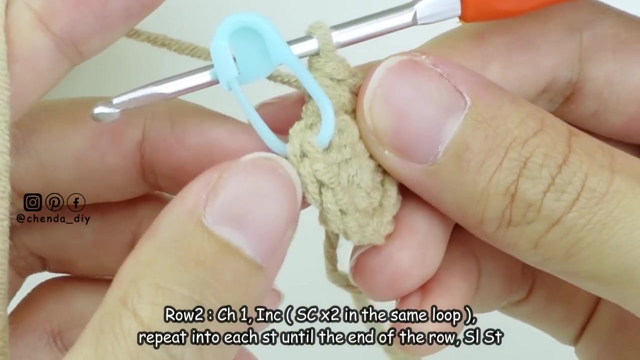 After you got 2 stitches in the same loop, then we are going to repeat the same thing by making 2 single crochet in the same loop. Thank you for watching. After you reach the end of the row, you must have 12 stitches in total. 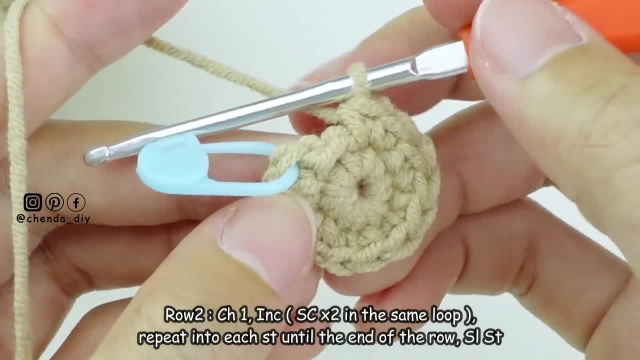 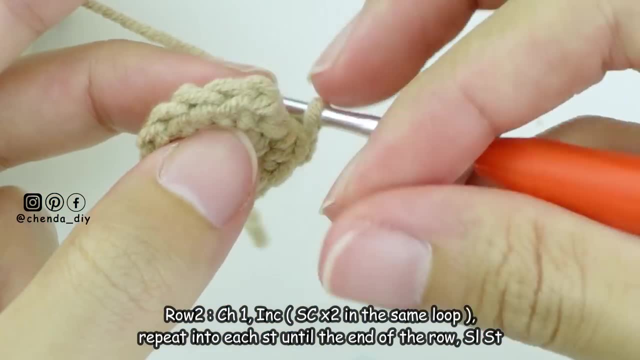 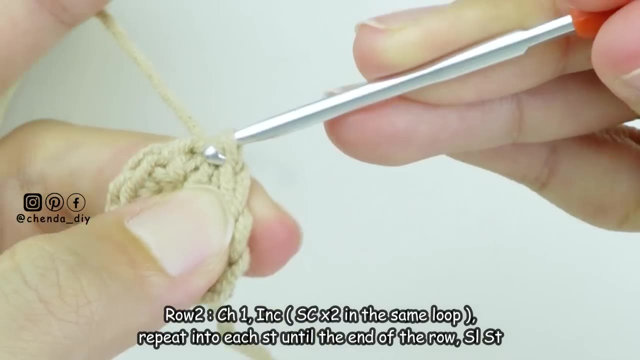 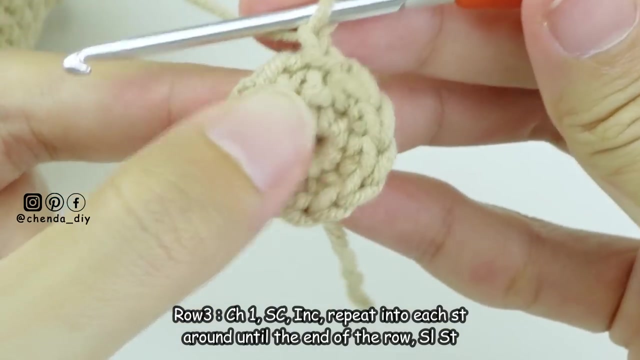 For the small loop that near chain 1, it then count as a stitch. so then make single crochet into that stitch. And then we are going to continue: make slip stitch into the stitch that we mark Next for row 3, chain 1, and make single crochet into the stitch near chain 1.. 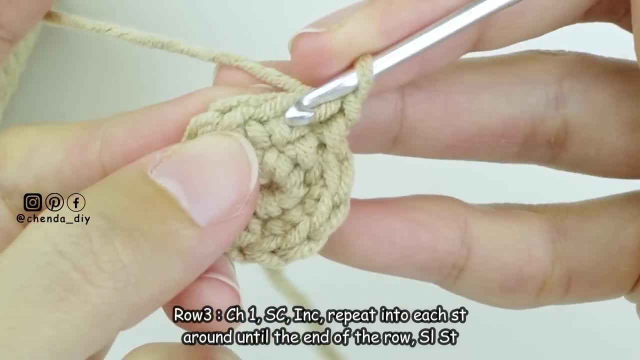 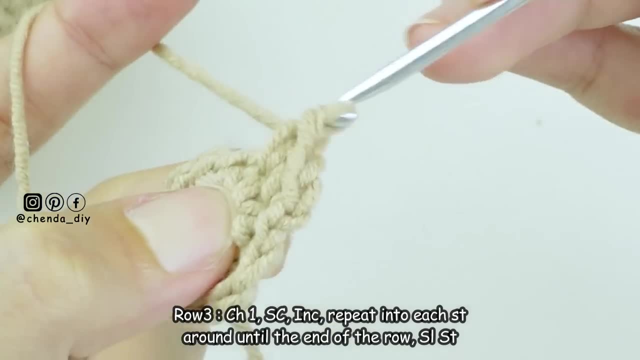 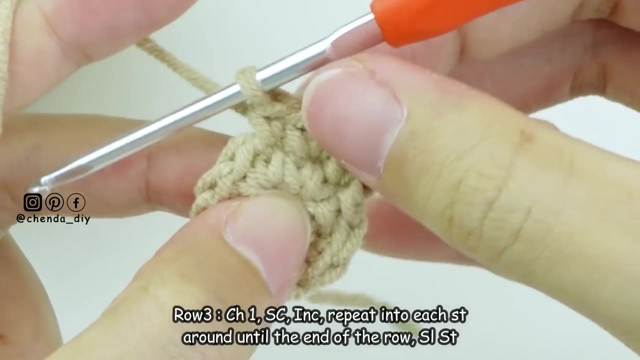 Next, we are going to make increase into the next stitch by make 2 single crochet in the same loop After you have make increase. then we are going to repeat the same thing by make single crochet in the next stitch and then make increase. 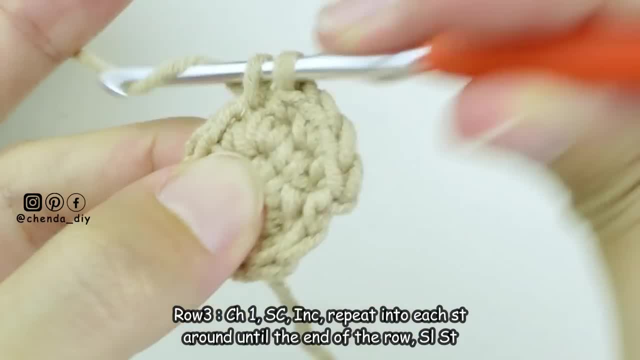 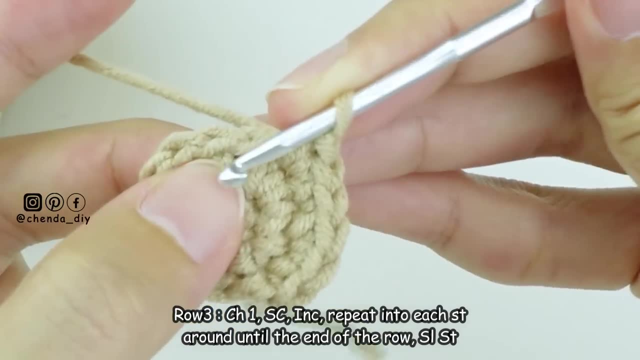 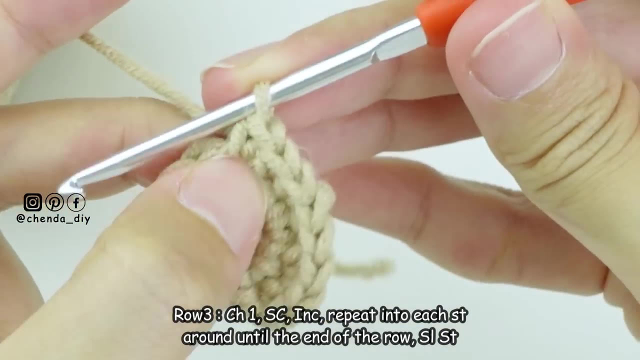 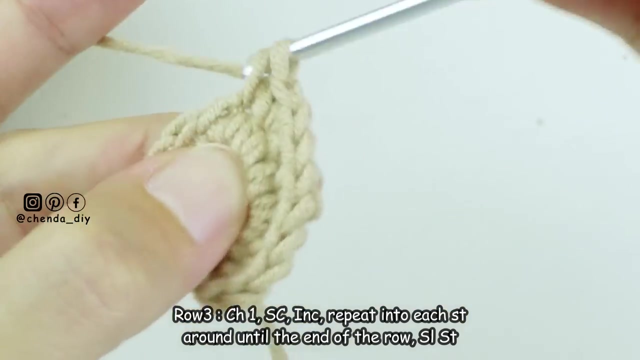 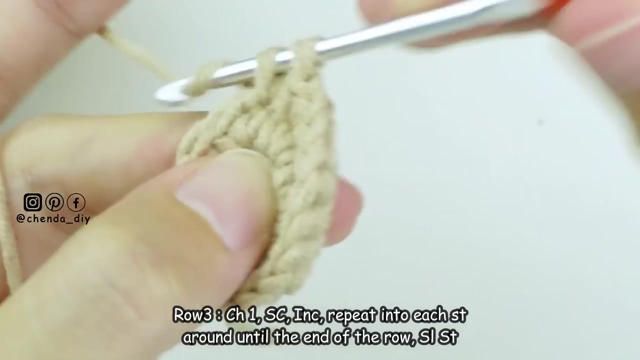 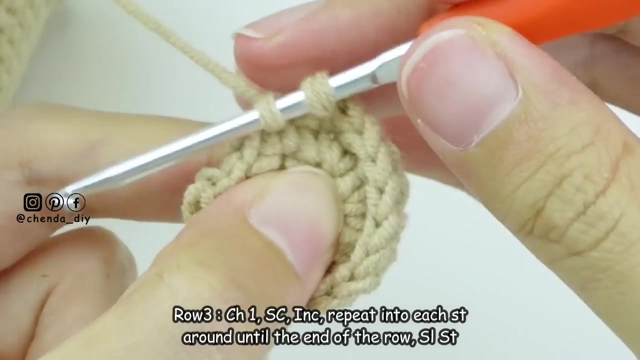 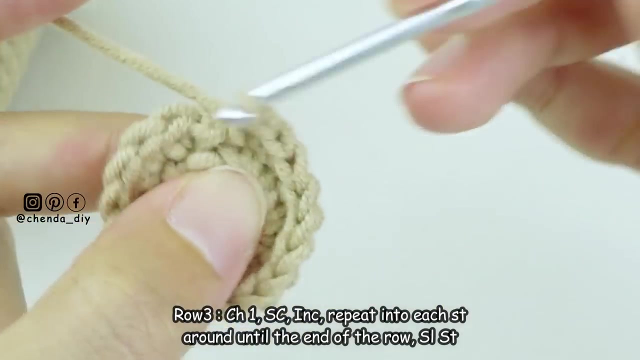 Keep repeating this around until you reach the end of the row. then we meet you back again After you have make increase. then we are going to repeat the same thing by make 2 single crochet in the next stitch, and then we meet you back again. 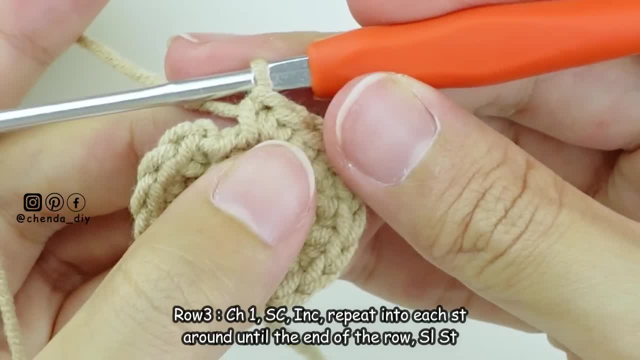 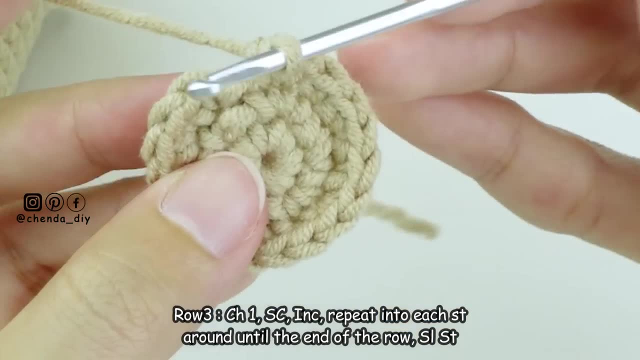 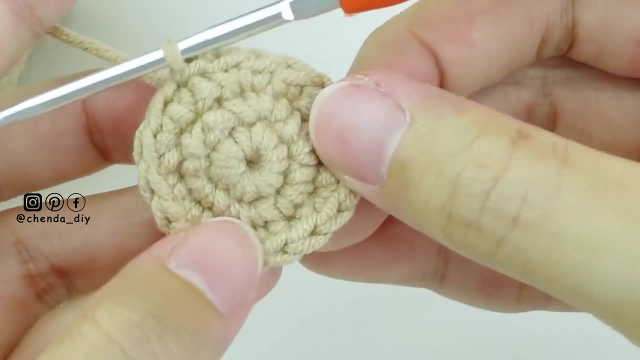 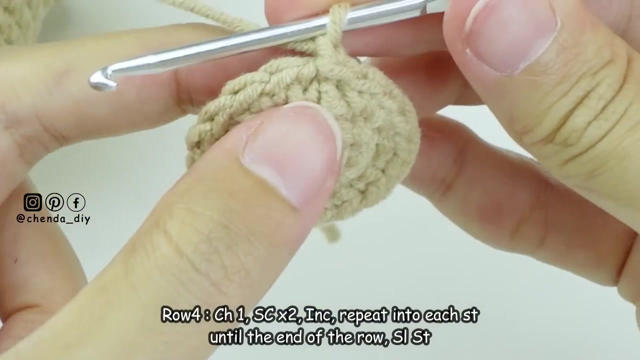 After you reach the end of the row you must end with increasing stitch And next we are going to continue. make slip stitch into the first single crochet stitch After you have. make slip stitch next for row 4,, chain 1, and make single crochet into the stitch near chain 1.. 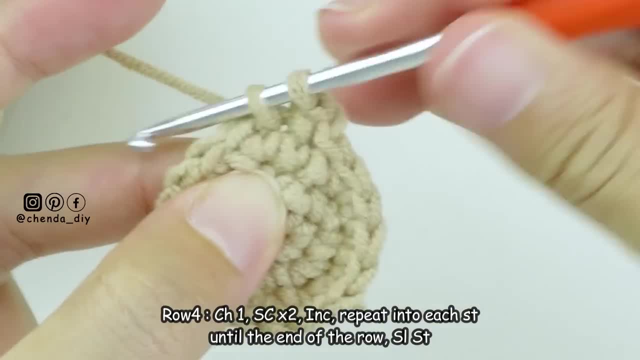 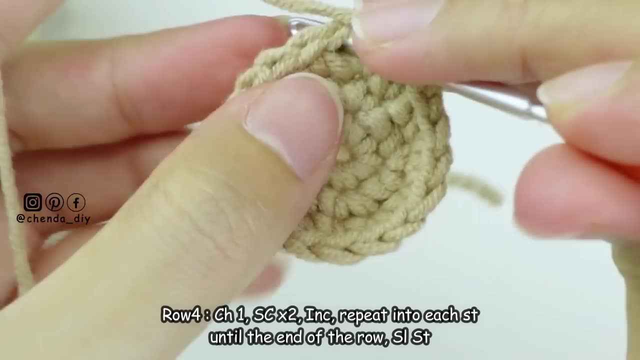 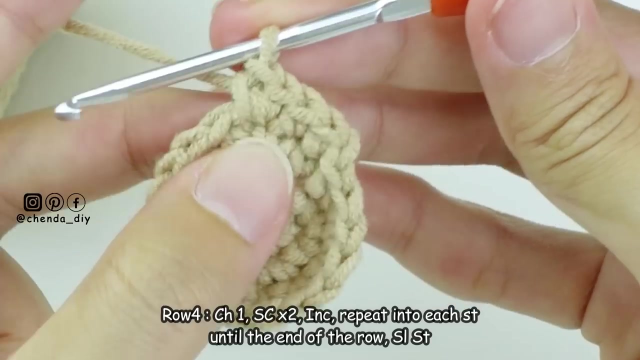 And then make another single crochet into the next stitch After you got 2 single crochet. and then we are going to make increase into the next stitch by make 2 single crochet in the same loop. After you have make increase, then we are going to repeat the same thing by make 2 single crochet. 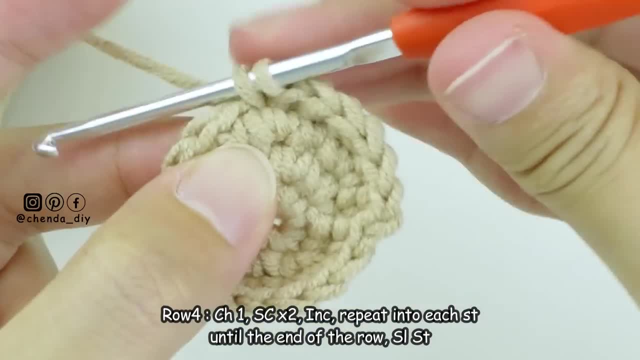 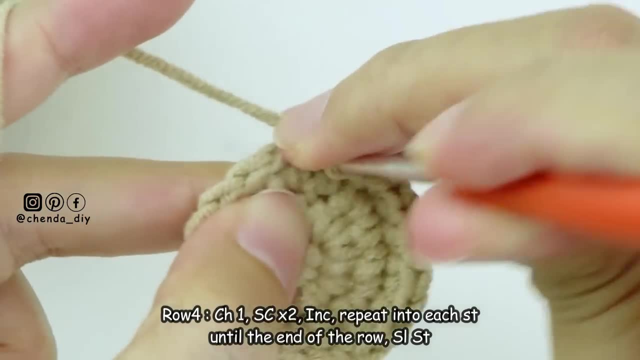 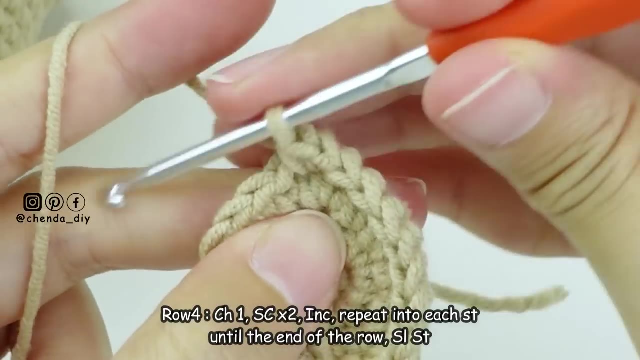 and then make increase until you reach the end of the row. then we meet you back again. After you have make increase, then we are going to repeat the same thing by make 2 single crochet into the next stitch and then we meet you back again. 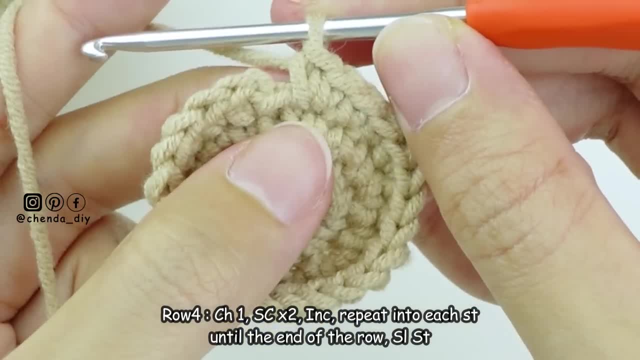 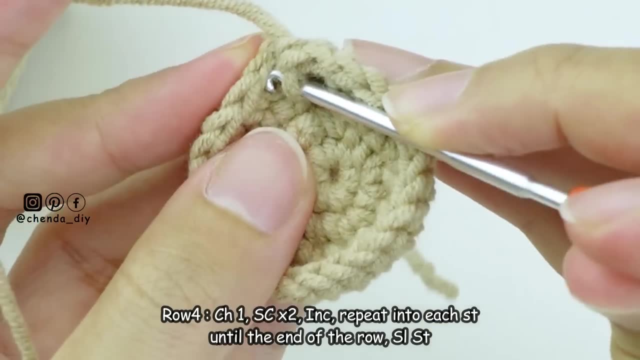 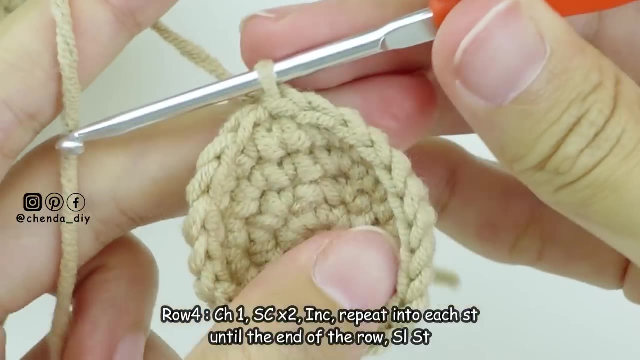 Like I said at the end of the row, you must end with increasing stitch. then we are going to continue make slip stitch into the first single crochet stitch After you have make increase, then we are going to continue make slip stitch into the first single crochet stitch. 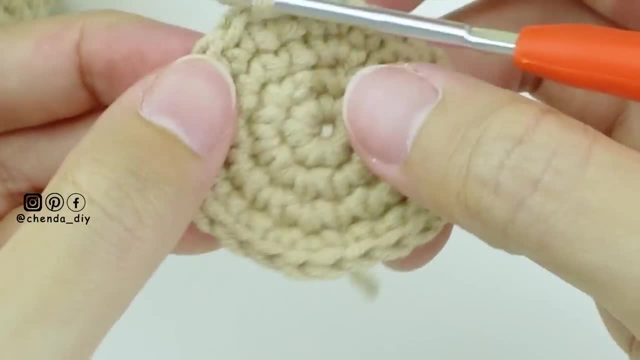 Like I said at the end of the row, you must end with increasing stitch. Next for row 5, chain 1, and make a sc into next 3 stitches. Next for row 5, chain 1, and make a sc into next 3 stitches. 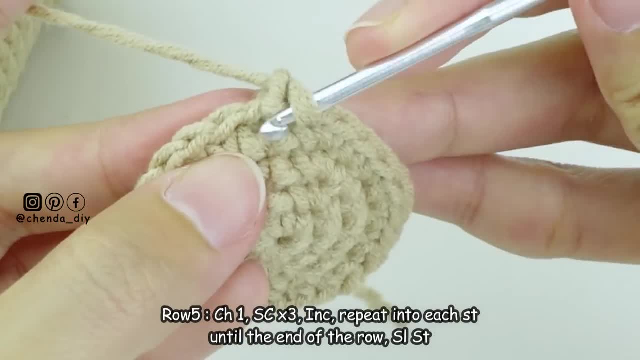 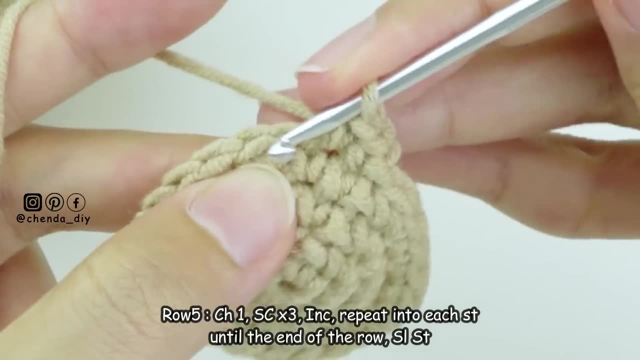 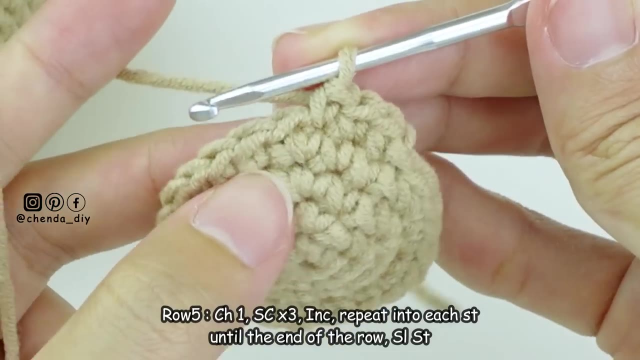 Next for row 5,, chain 1, and make a sc into next 3 stitches. Ex P T. After you got 3 sc, then we are going to make an increase into the next 3 stitches. ück, Yes, it is. 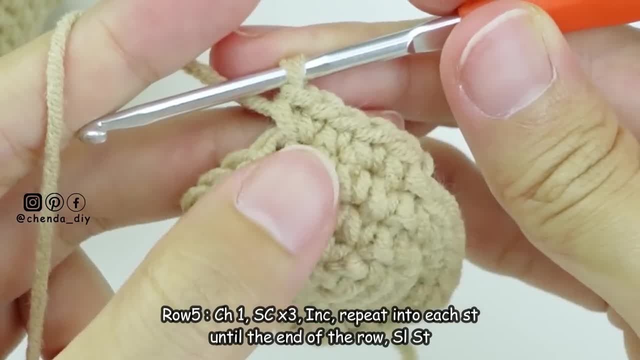 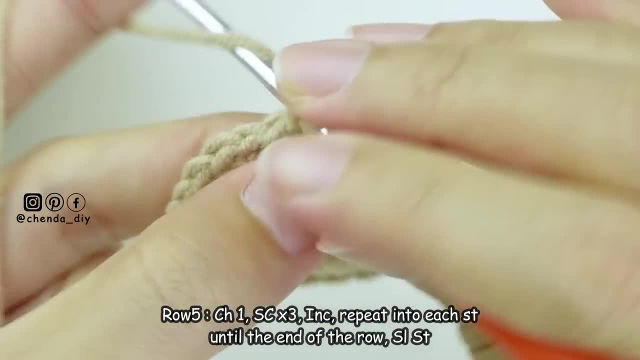 Thanks for watching. Yeah, thanks for watching. i will see you guys. Oh, thank you so much. Good bye everyone. See you all in my next video, After you have made increase. then we are going to repeat the same thing by make 3 single crochet and then increase until you reach the end of the row. then we meet you back again. 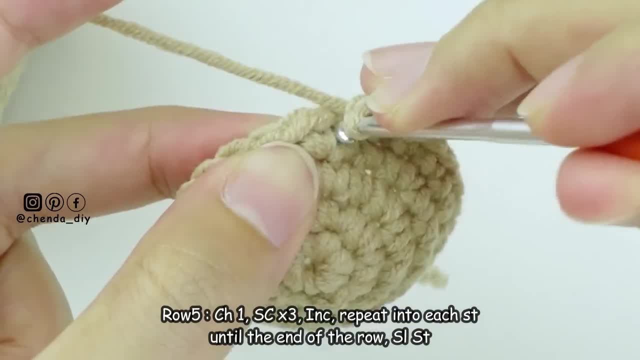 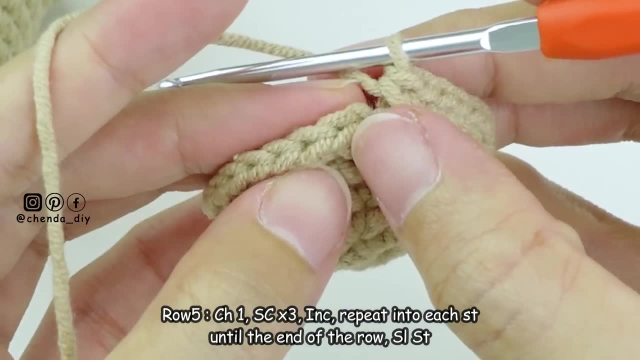 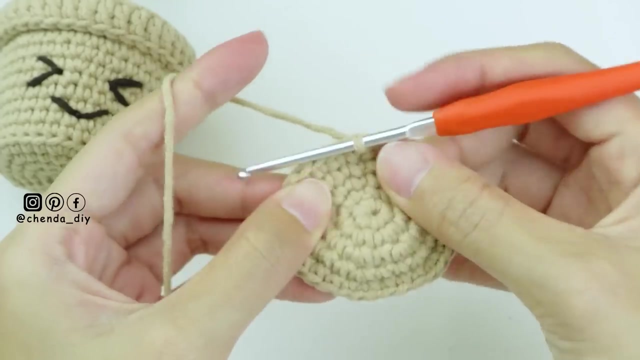 After you reach the end of the row, then we are going to make slip stitch into the first single crochet stitch. You have to stretch it a little bit to give a nice and flat circle, And this is what it looks like after you reach row 5.. 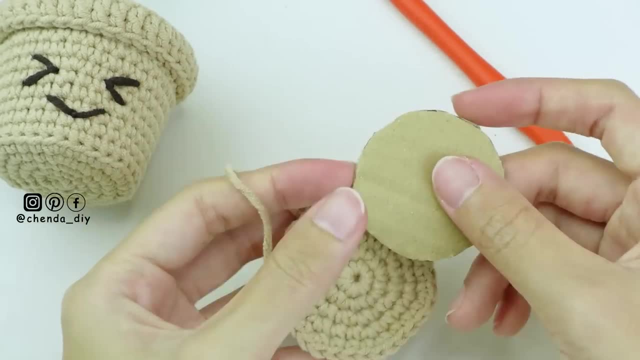 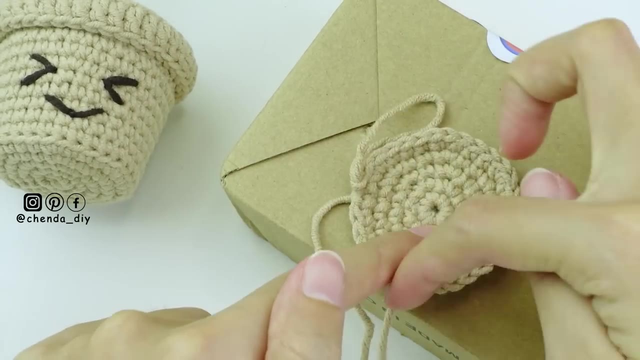 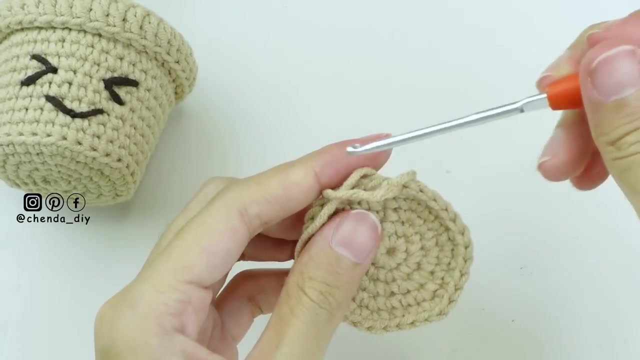 And next we are going to use this pot base to place on the cardboard. You can use any type of cardboard. You can use a pen to draw around the circle and cut it. Next, continue from where your last stitch is for row 6, chain 1.. 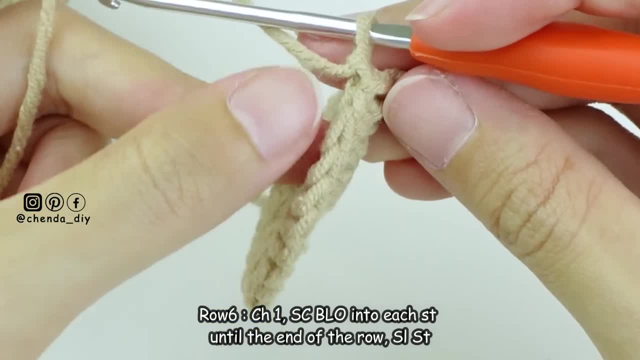 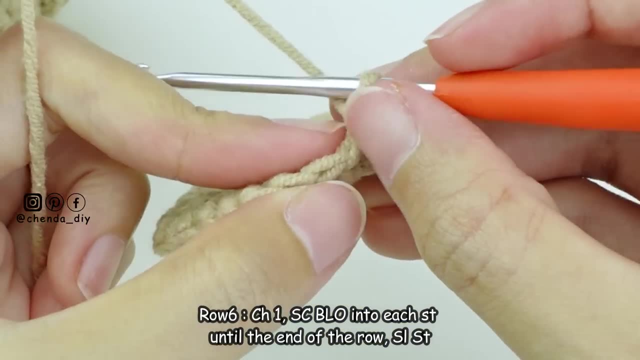 Then we are going to make single crochet but into the back loop of the stitch only. Single crochet back loop only into the stitch near chain 1.. Single crochet back loop only into the stitch near chain 1.. Single crochet back loop only into the stitch near chain 1.. 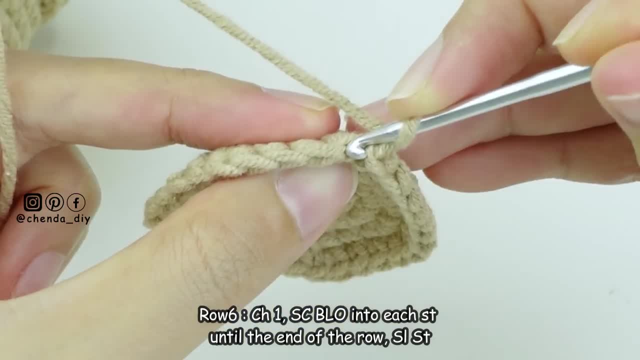 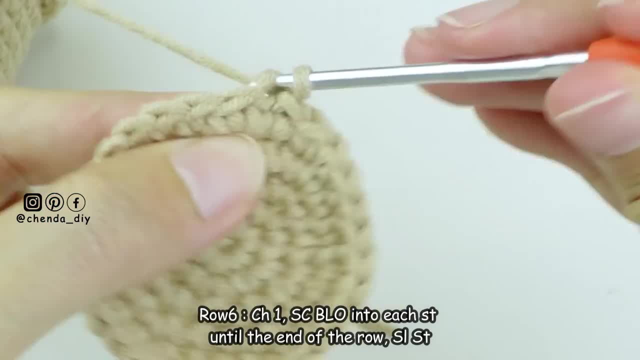 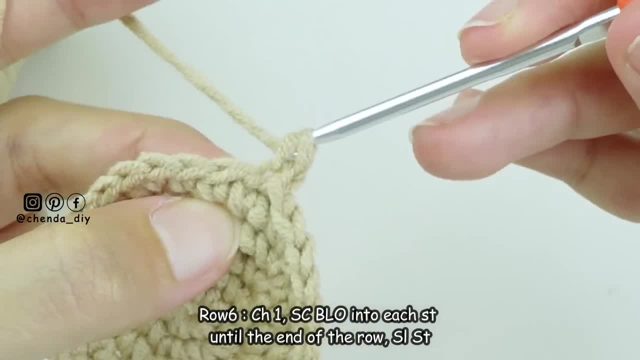 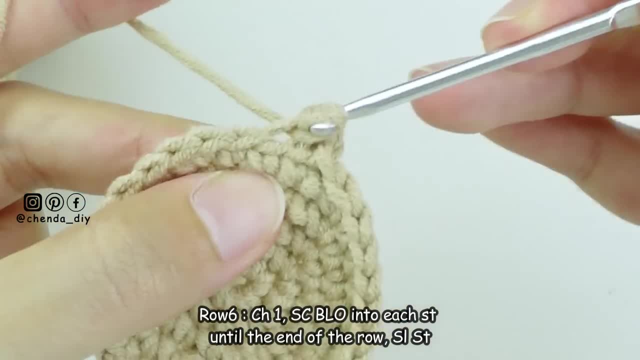 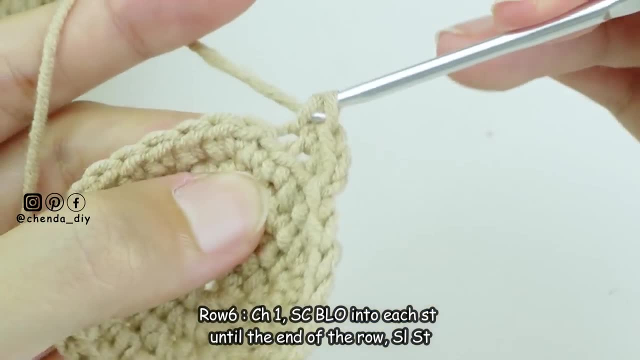 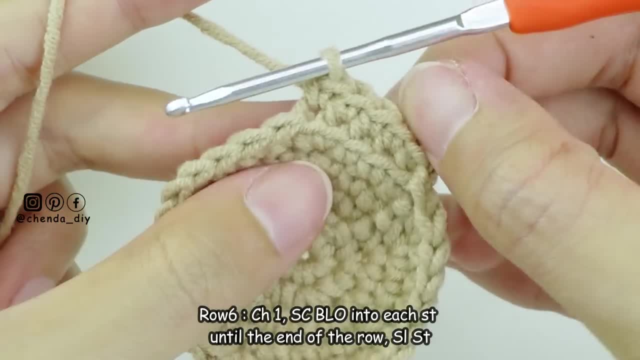 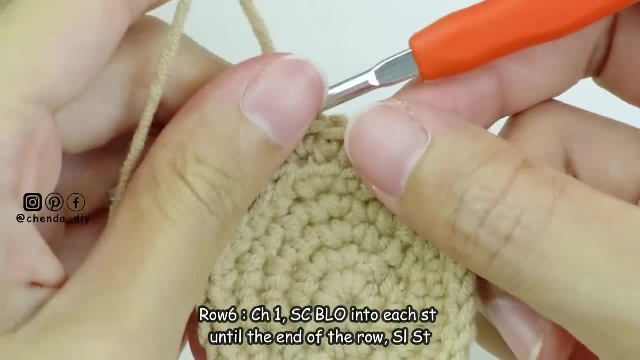 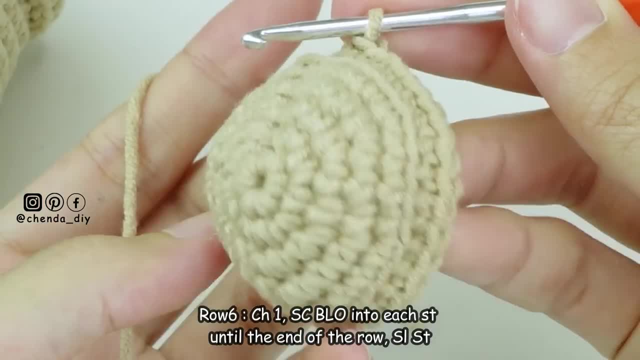 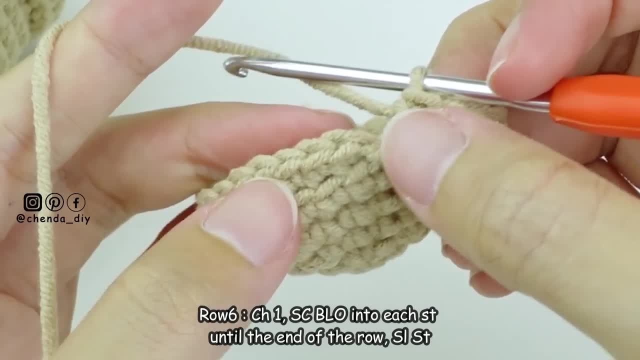 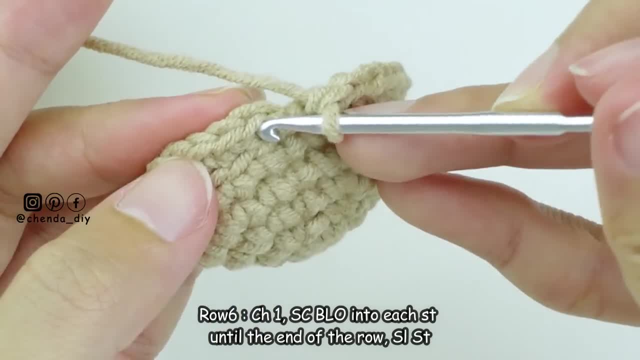 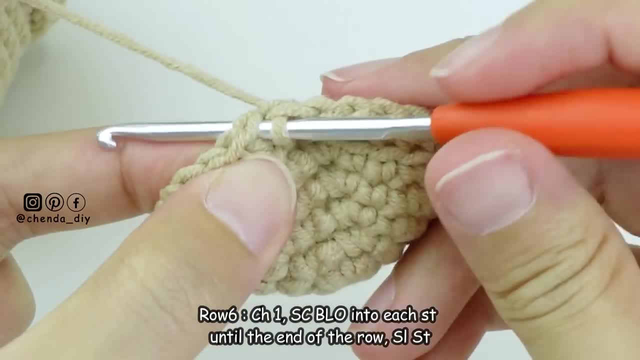 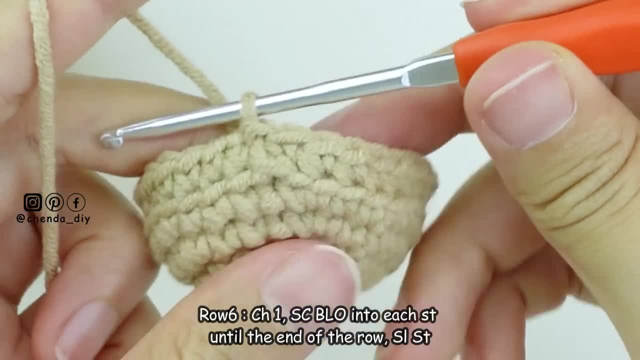 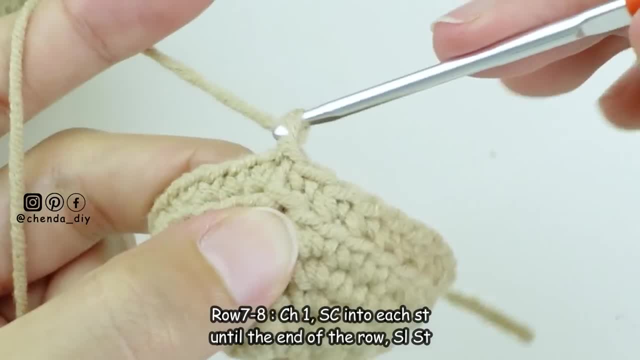 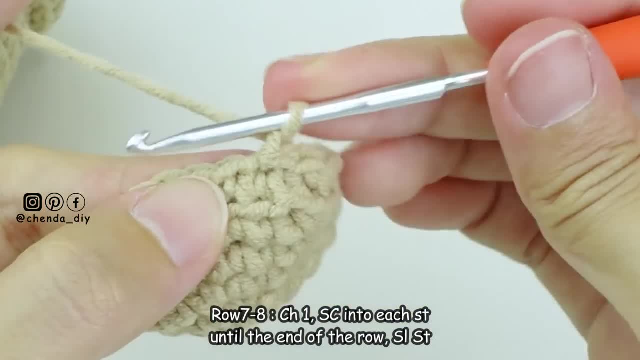 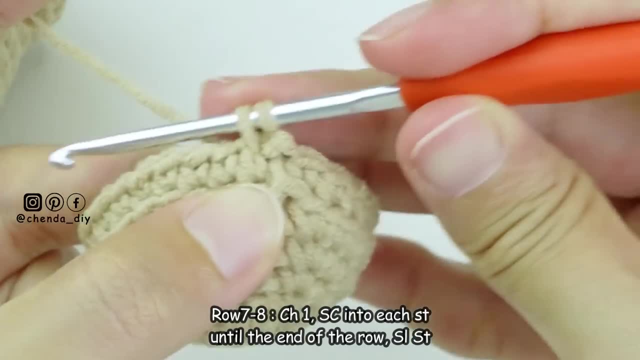 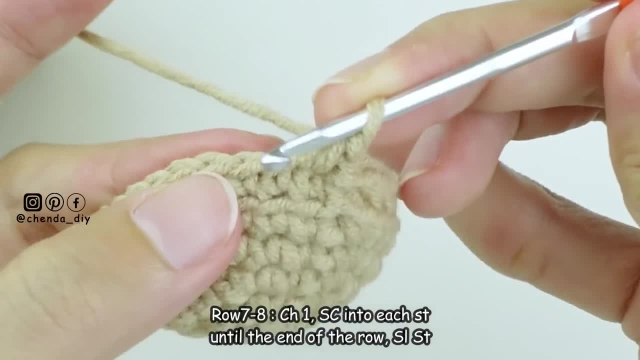 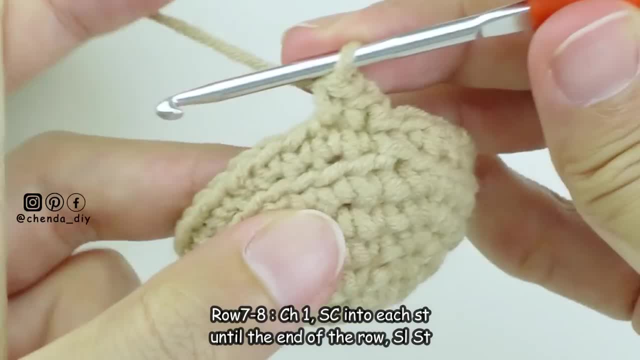 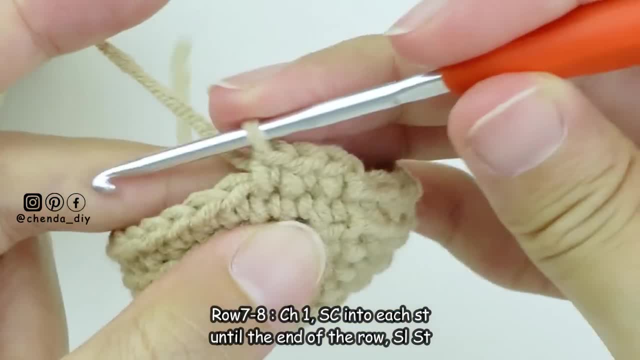 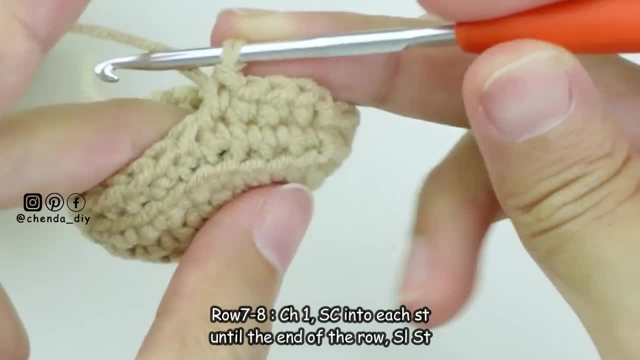 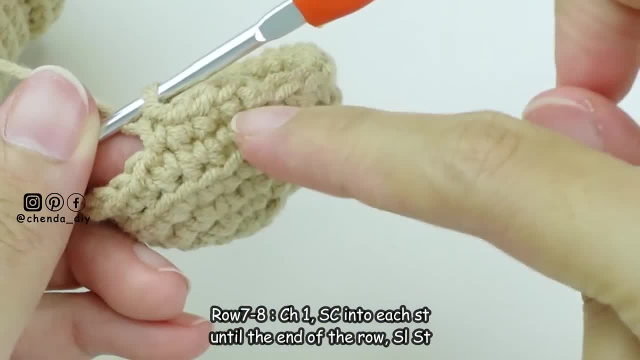 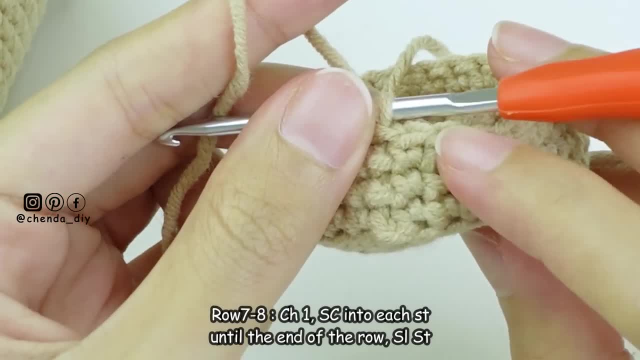 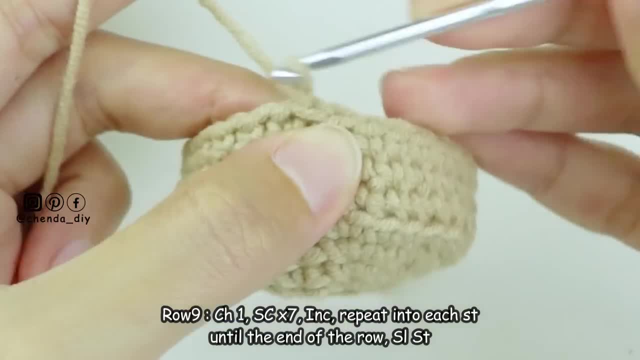 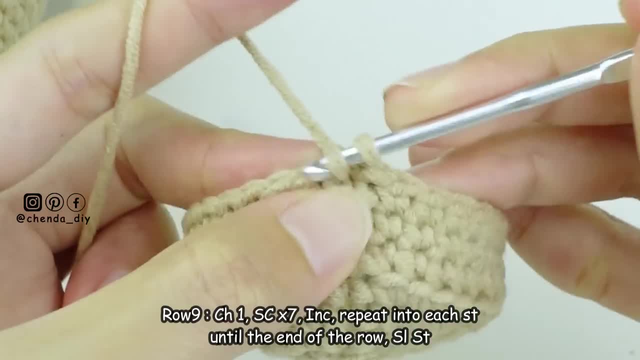 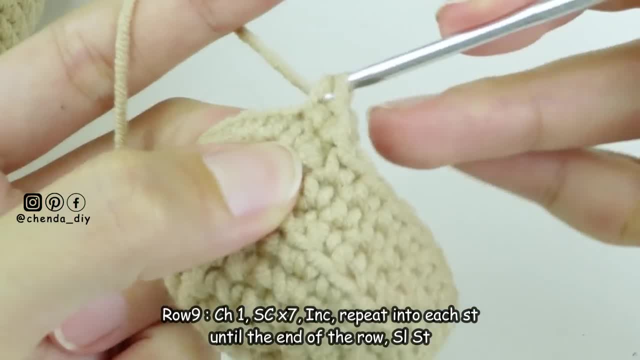 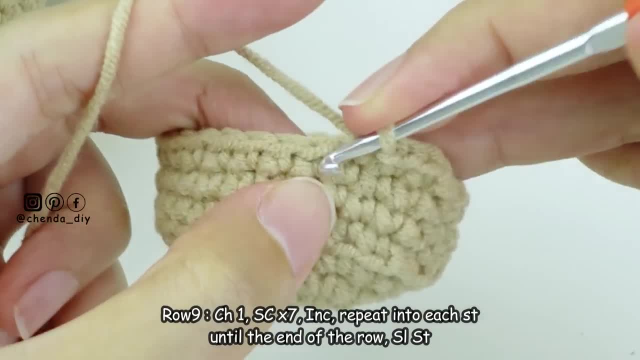 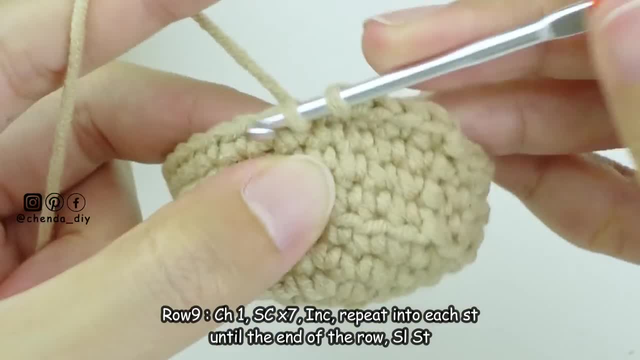 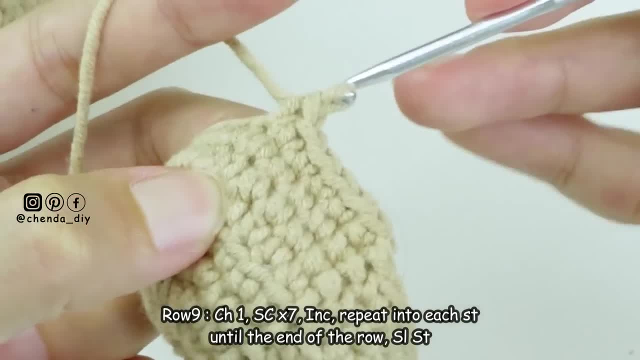 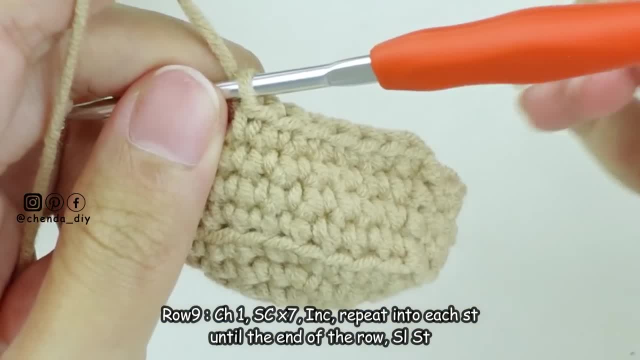 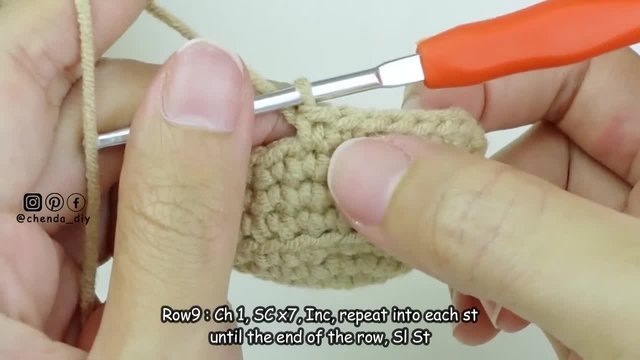 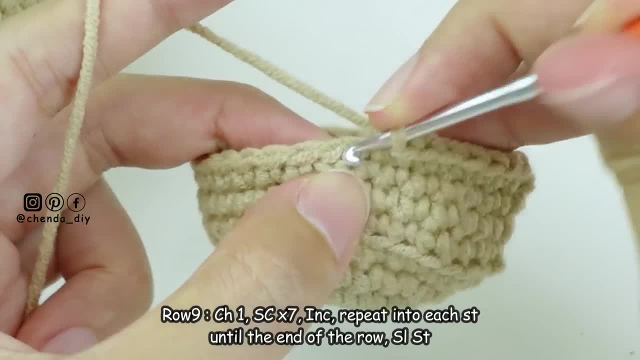 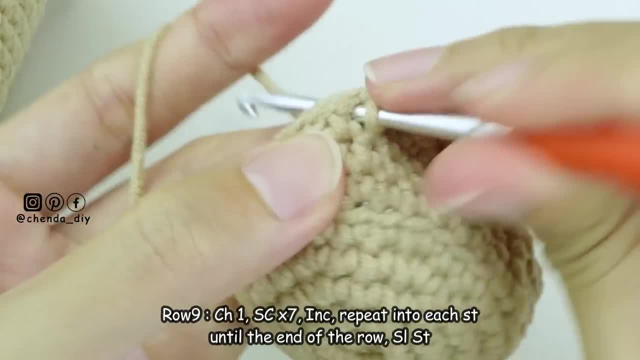 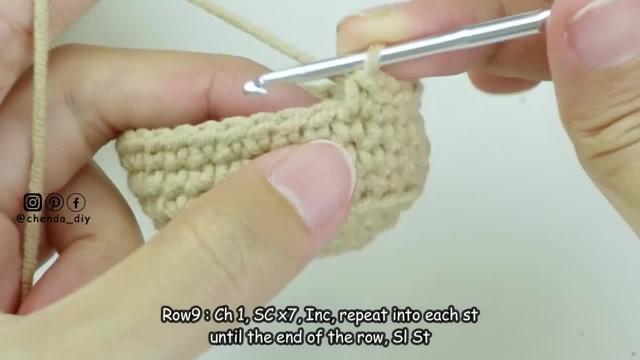 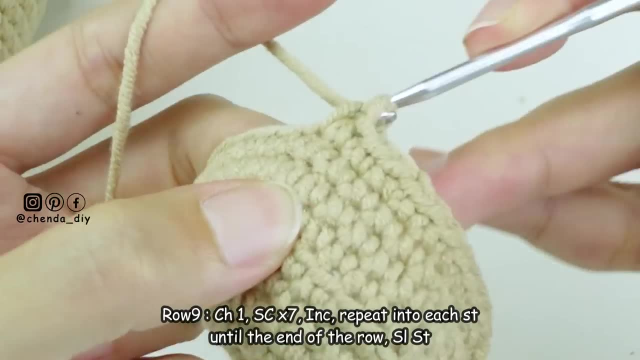 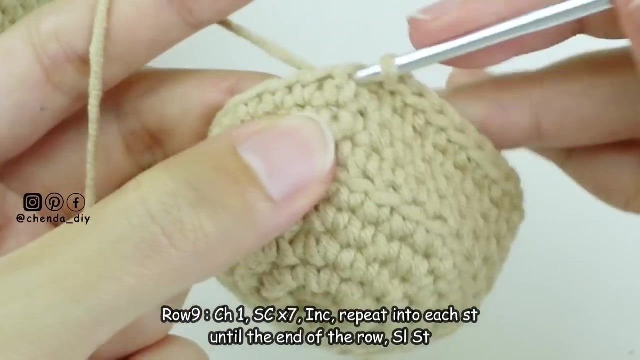 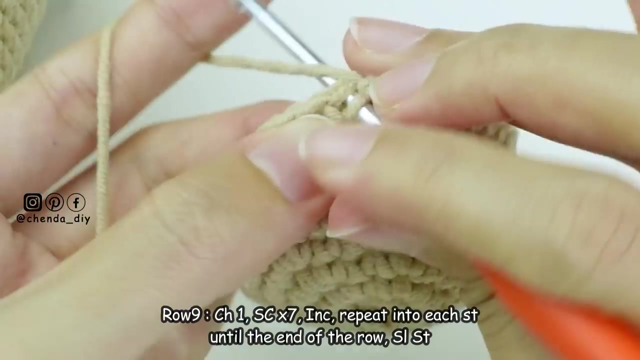 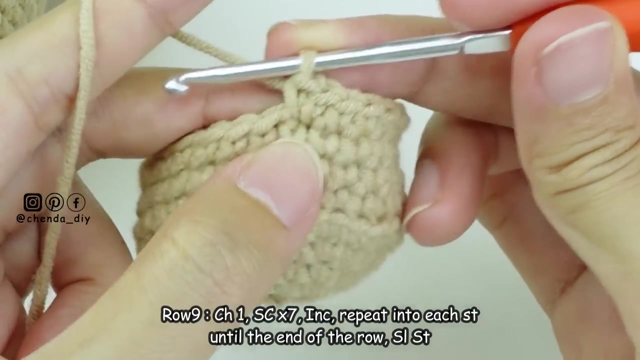 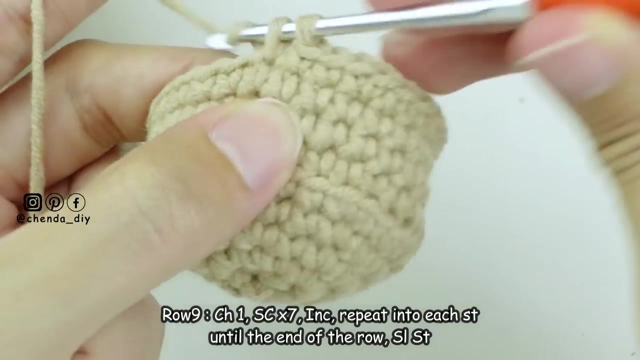 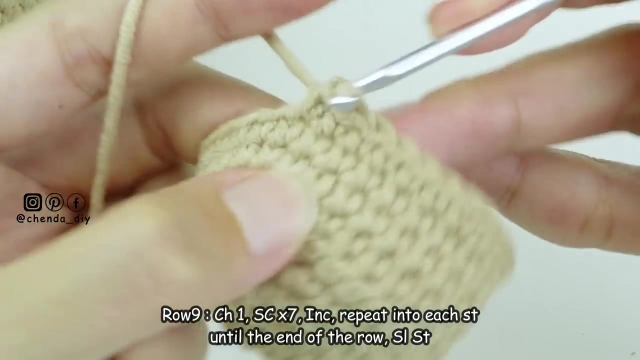 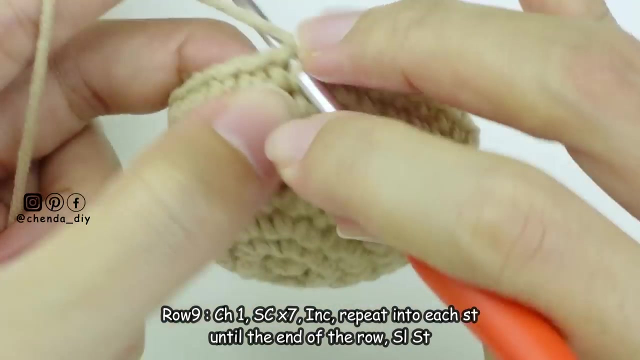 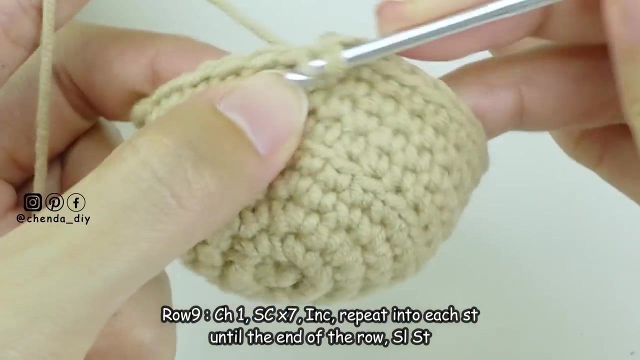 After you have made increase, then we are going to repeat the same thing by make 7 single crochet and then increase Until you reach the end of the row. then we meet you back again. Music. For this last increasing stitch, I make 5 single crochet and then increase into the last stitch of the row. 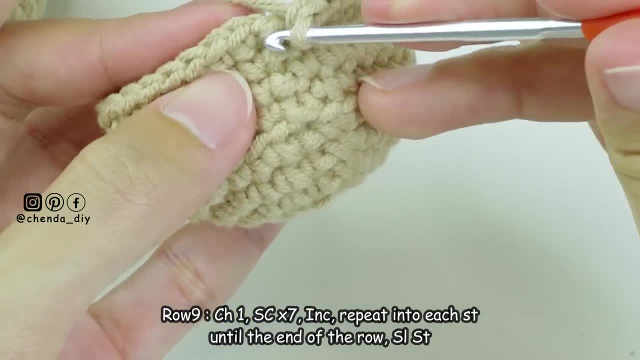 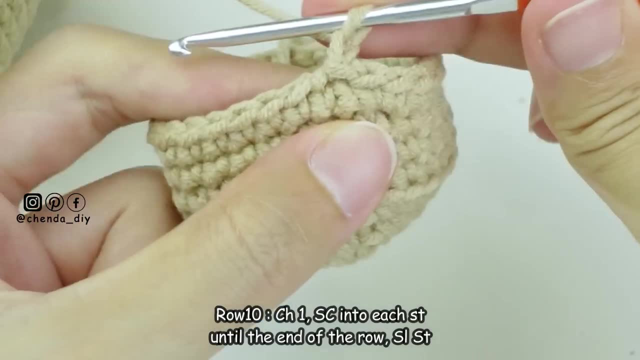 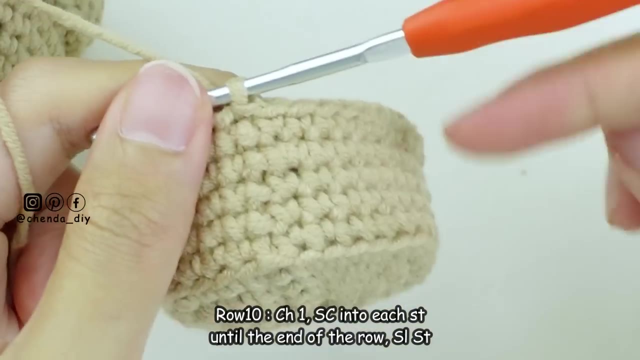 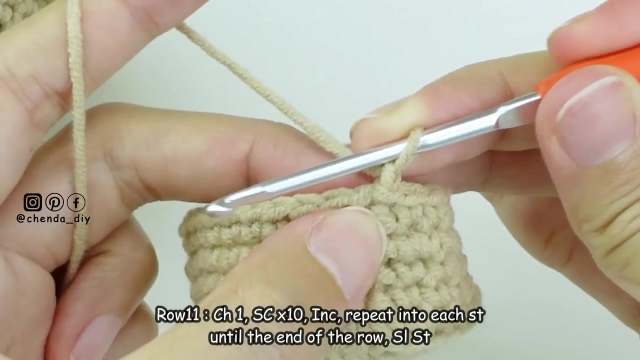 After you have made increase, then continue. make slip stitch into the first single crochet stitch. Next for row 10, chain 1, and make single crochet into each stitch around until you reach the end of the row. then make slip stitch After you have made slip stitch. next for row 11, chain 1, and make single crochet into the next 10 stitches. then I will meet you back again. 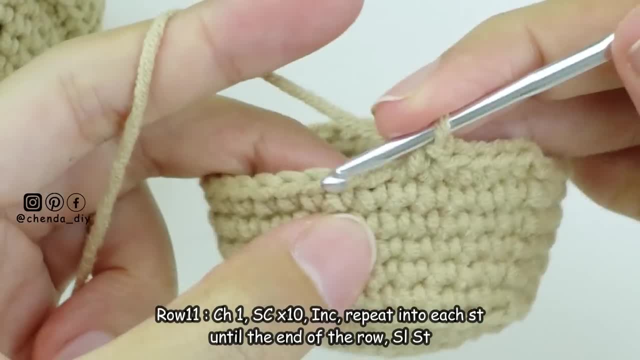 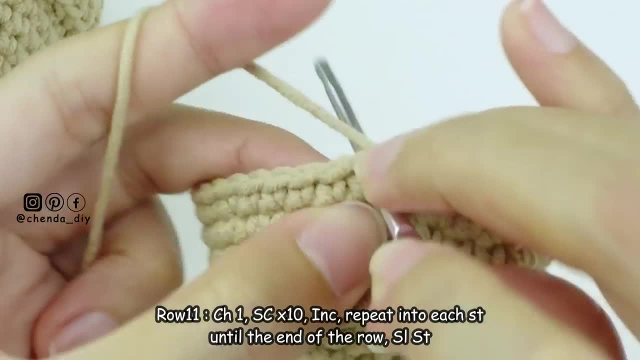 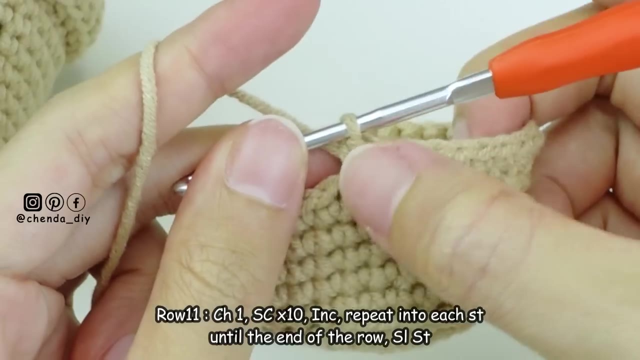 After you have made slip stitch, next for row 11, chain 1, and make single crochet into each stitch around until you reach the end of the row. then make slip stitch into each stitch around After you got 10 stitches of single crochet, then we are going to make increase into the next stitch. 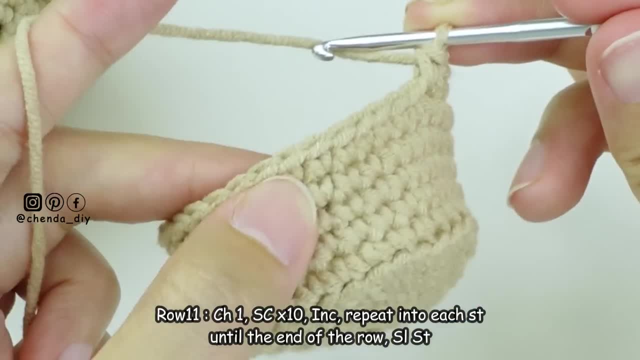 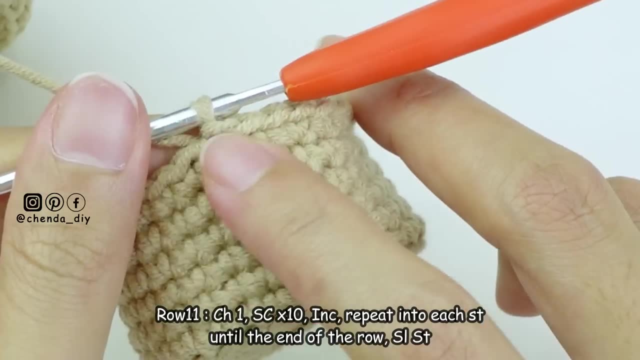 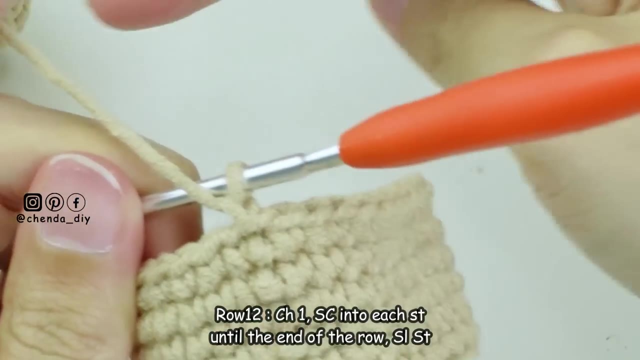 After you have made increase, then we are going to repeat the same thing by make 10 single crochet And then increase until you reach the end of the row, then make slip stitch. Next for row 12, chain 1, and make single crochet into every stitch until the end of the row, then make slip stitch. 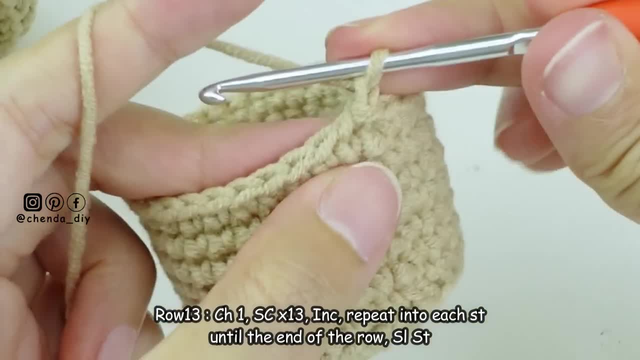 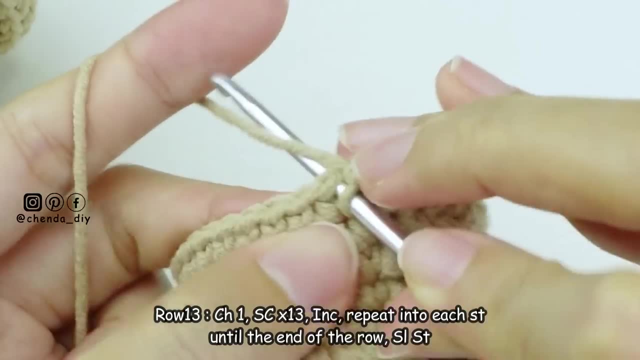 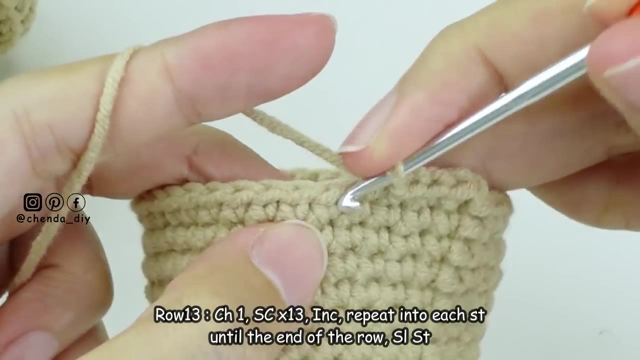 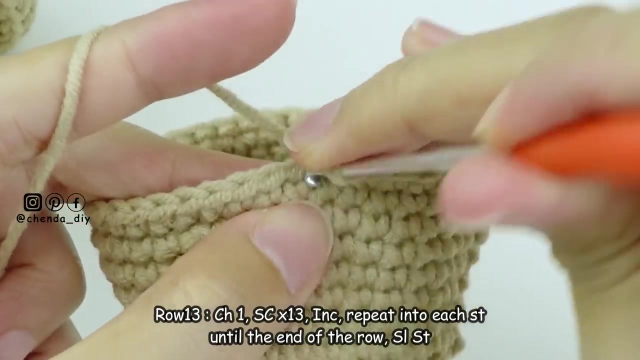 After you have made slip stitch for row 13,, chain 1, and make single crochet into the next 13 stitches, then I will meet you back again After you have made slip stitch next for row 14, chain 1, and make slip stitch into each stitch around until you reach the end of the row, then we are going to repeat the same thing by make 10 single crochet. 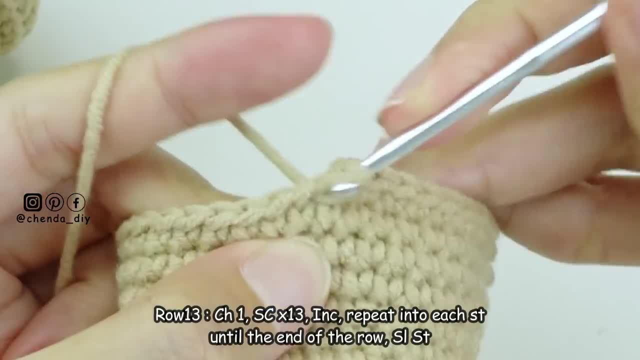 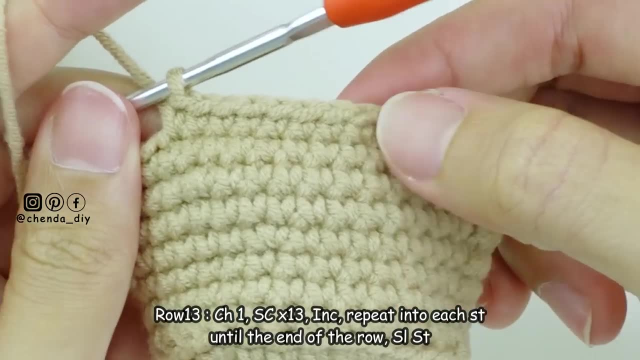 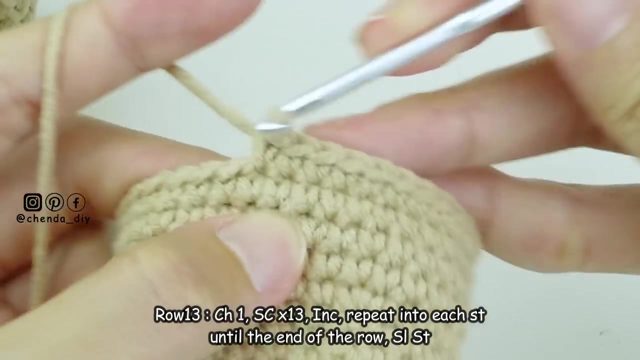 And then increase until you reach the end of the row. then we are going to repeat the same thing by make 10 single crochet. After you got 13 stitches of single crochet, then we are going to make increase into the next stitch. After you have made increase, then we are going to repeat the same thing by make 13 single crochet. 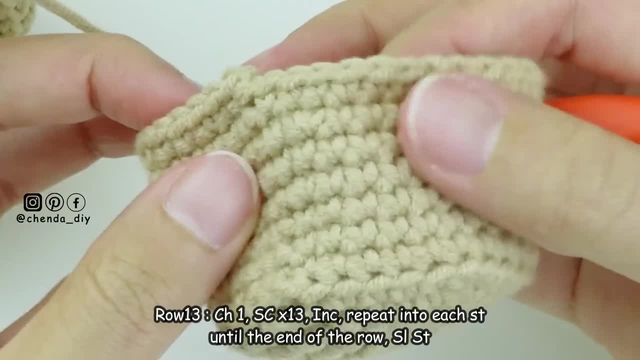 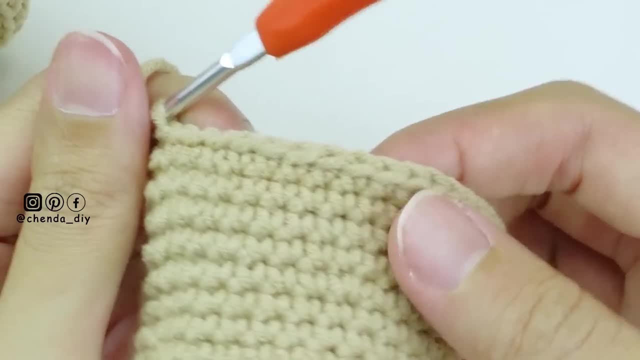 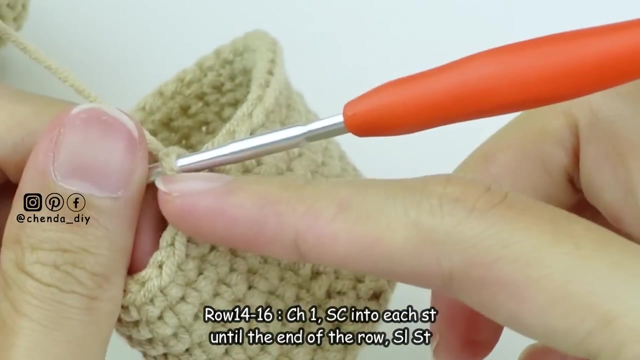 And then increase until you reach the end of the row. then make slip stitch. Next for row 14 until row 16, chain 1 and make single crochet into each stitch around until you reach the end of the row. then make slip stitch. 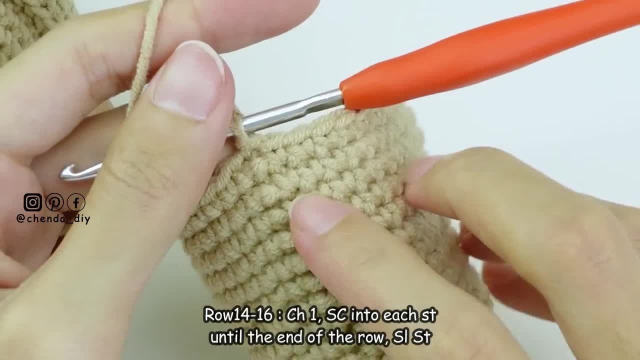 Then we meet you back again. After you have made 3 rows of single crochet, then we are going to repeat the same thing by make 13 single crochet. After you have made 3 rows of single crochet, then we are going to repeat the same thing by make 13 single crochet. 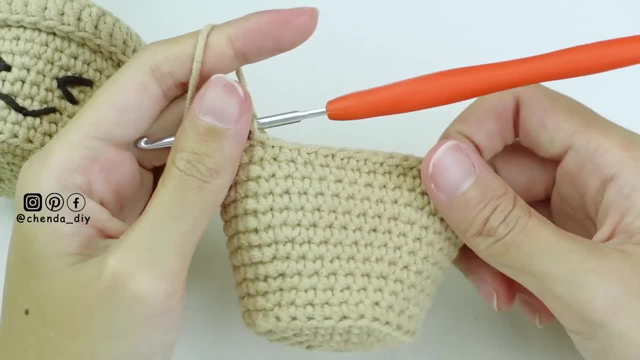 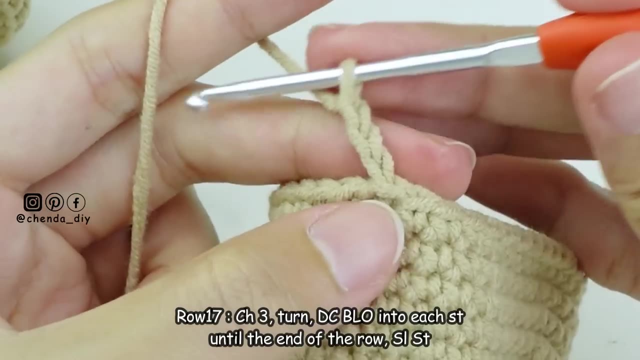 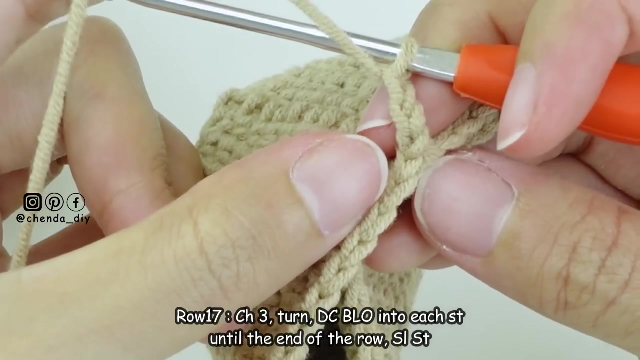 And now you must have 11 rows for the side of the pot. Next for row 17,. chain 3: Turn your work. then we are going to make double crochet back loop, only To make double crochet yarn over and sew the hook into the back loop. 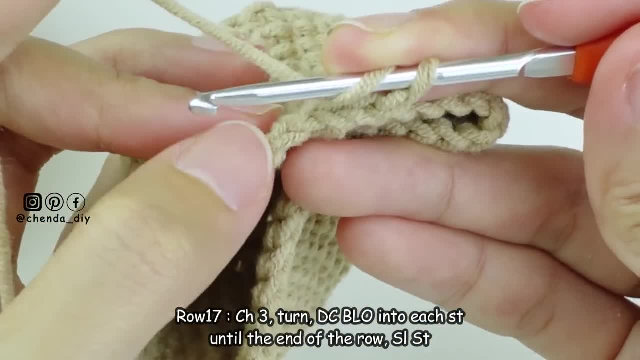 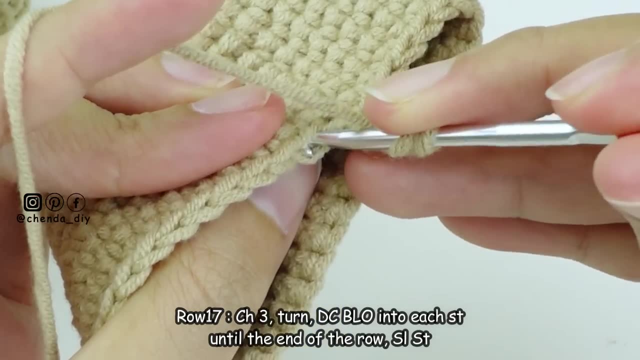 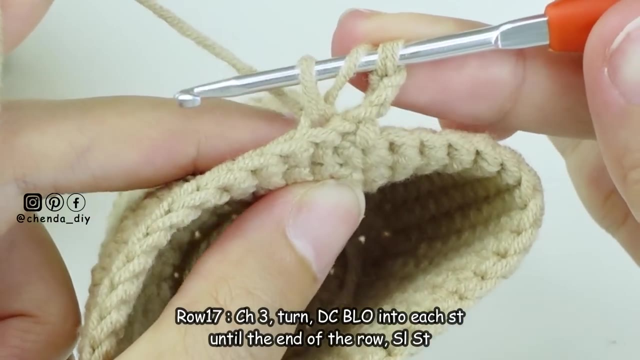 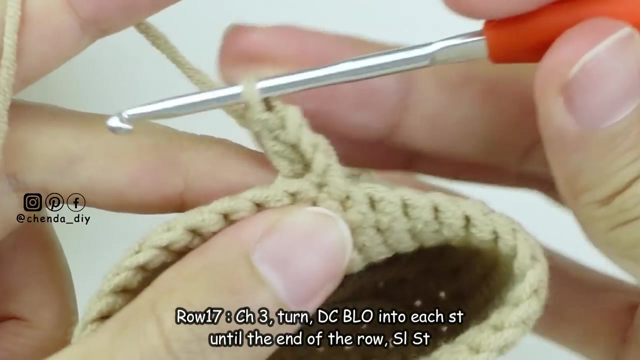 To make double crochet: yarn over and sew the hook into the back loop. Yarn over and pull up a loop, and now you have 3 loops on your hook. Yarn over, pull through 2.. And yarn over, pull through 2 loops again. 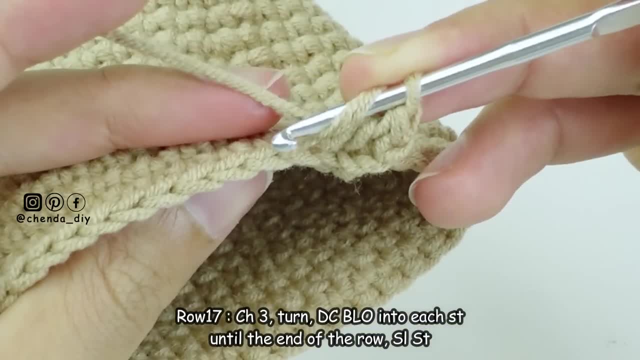 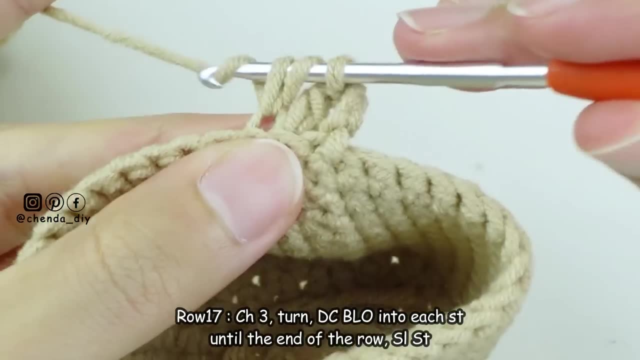 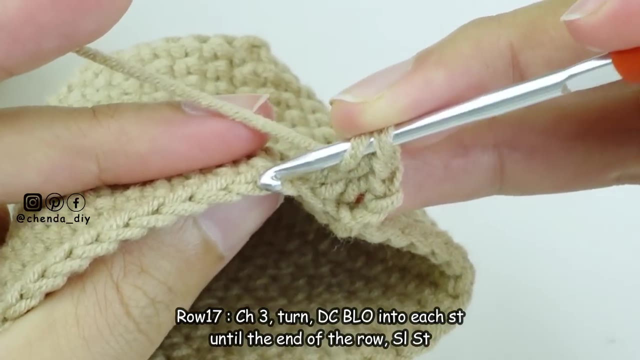 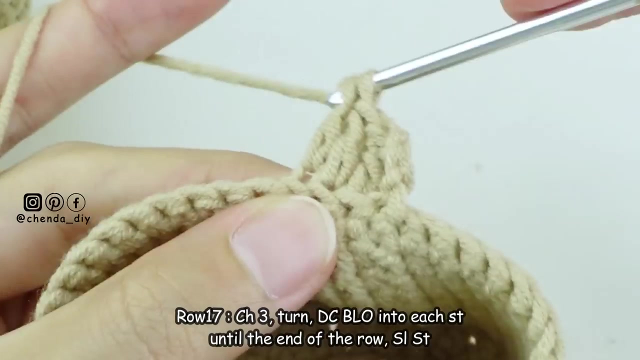 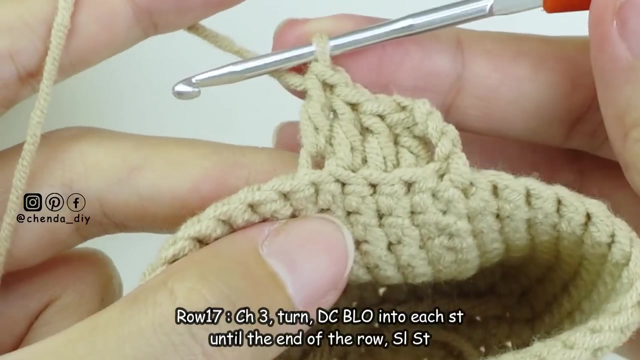 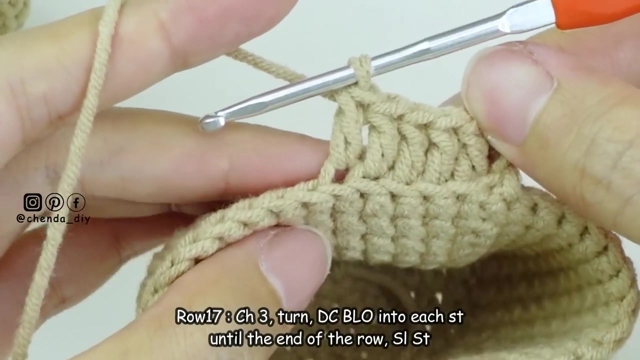 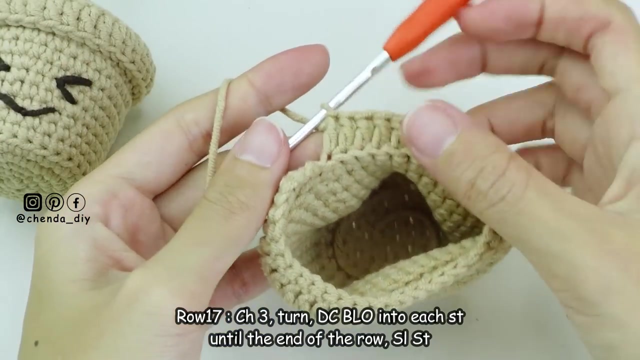 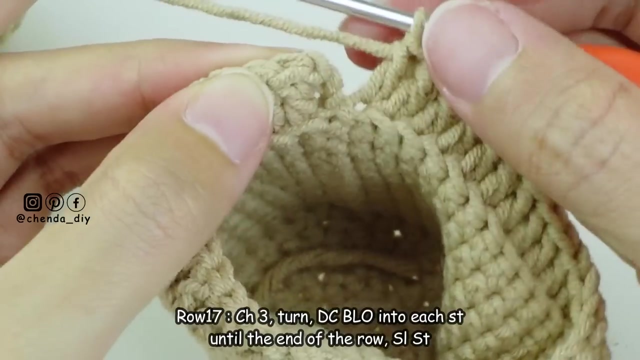 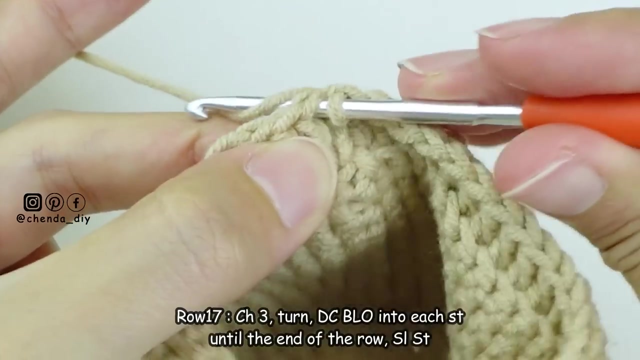 Keep making double crochet back loop only into each stitch around until you reach the end of the row And we meet you back again After you reach the end of the row. next we are going to make slip stitch into the first double crochet stitch, not into the chain. 3 stitch. 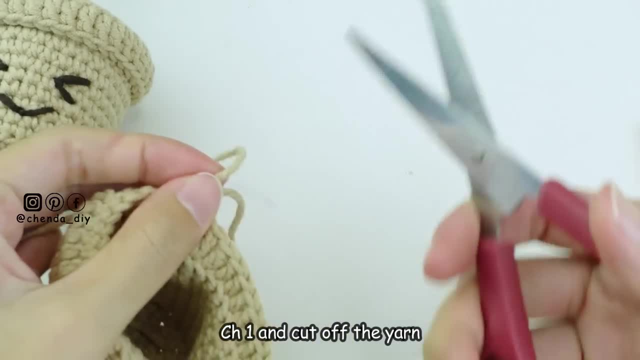 Then chain 1 and cut off the yarn. Yarn over: pull through 2.. Yarn over: pull through 2.. Yarn over: pull through 2.. Yarn under: pull though the chain and remove the yarn. Then turn the work inside out into a half這個. 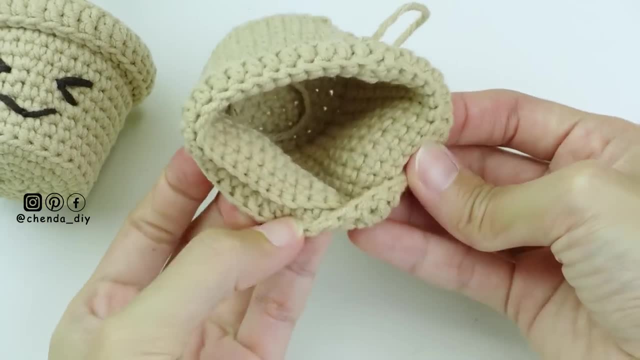 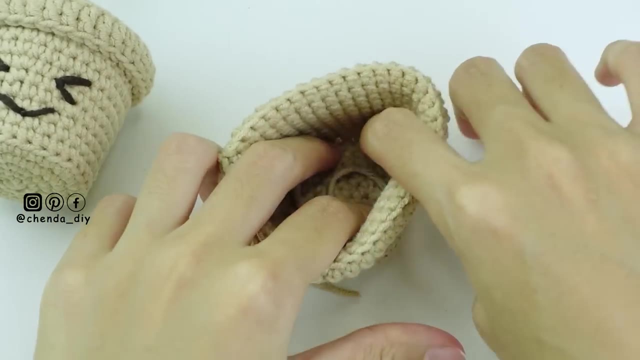 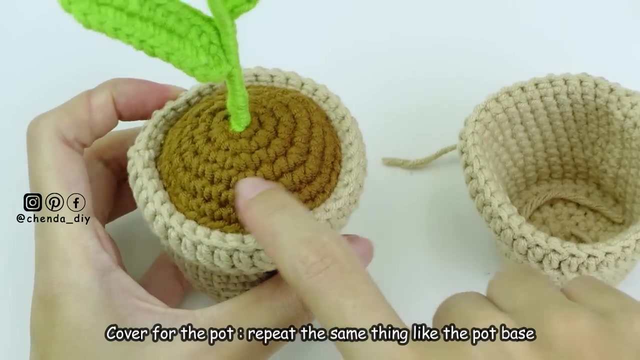 Flip the double crochet inside out like this. And now the pot is done. Next we are going to make the cover for the pot. For the cover of the pot, we repeat the same thing, like the pot base, make a magic circle. 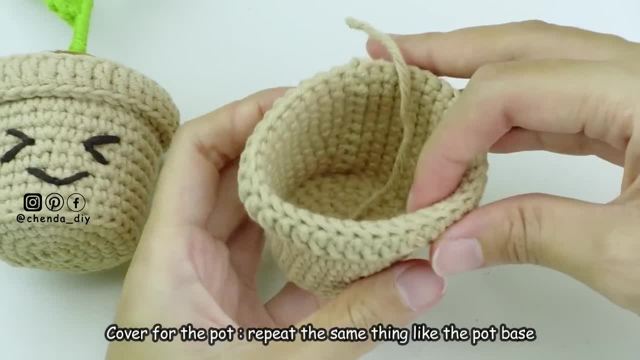 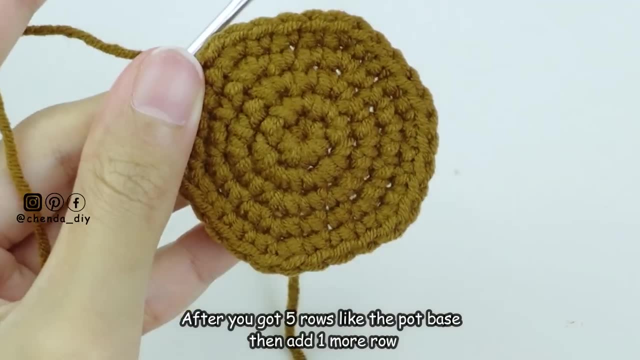 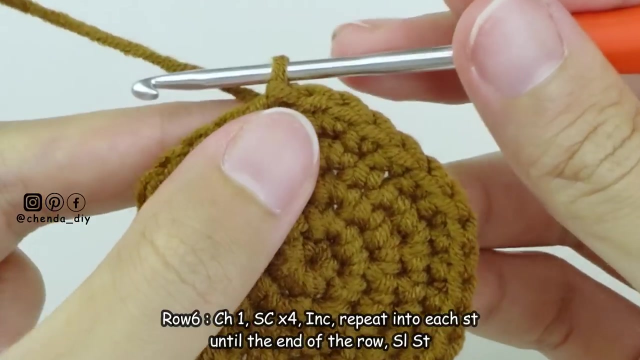 d6. into the circle and then keep increasing until you got 5 rows. After you got 5 rows, like the pot base, then we are going to add one more row. Continue from where your last stitch is For row 6, chain 1, and make single crochet into the 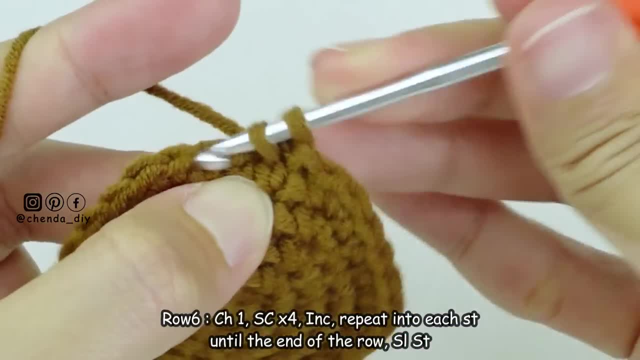 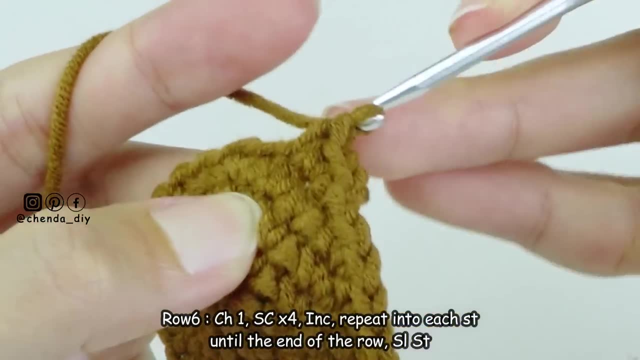 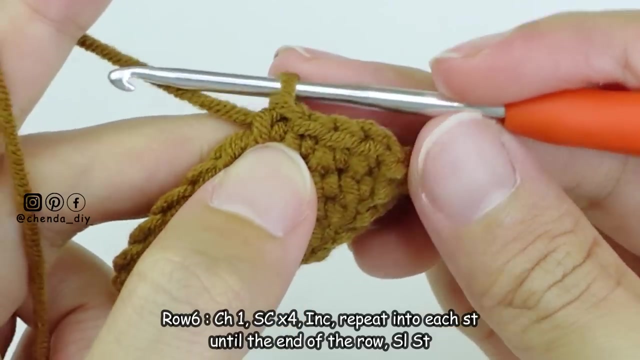 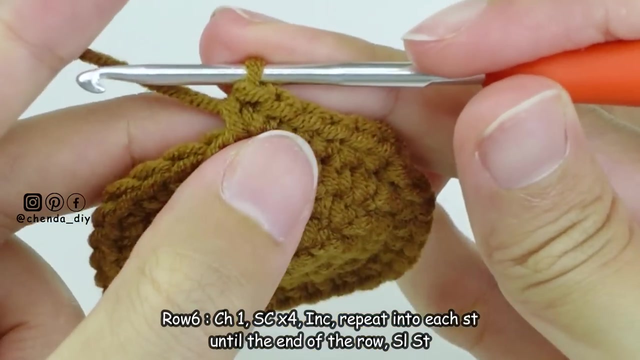 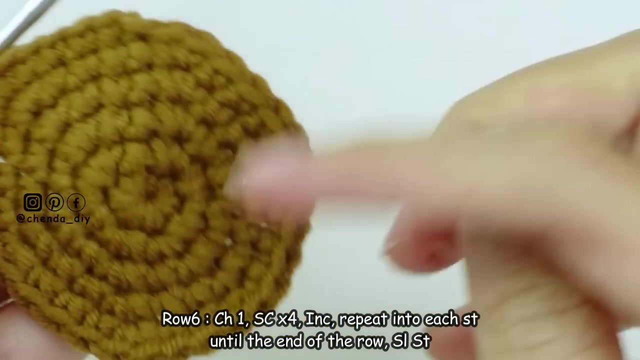 next 4 stitches. After you got 4 stitches of single crochet, then make increase into the next stitch. After you have made increase, then we are going to repeat the same thing by make 4 single crochet and then increase. Repeat this until you reach the end of the row, then make slip stitch into the. 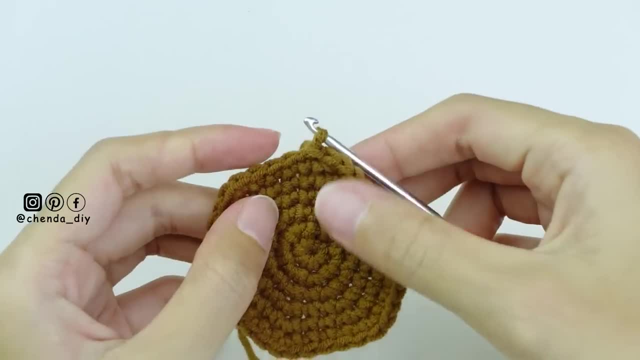 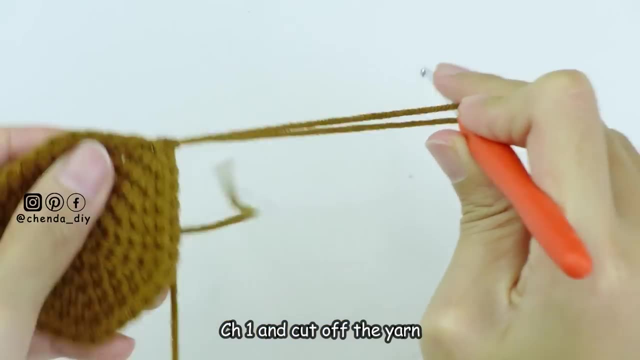 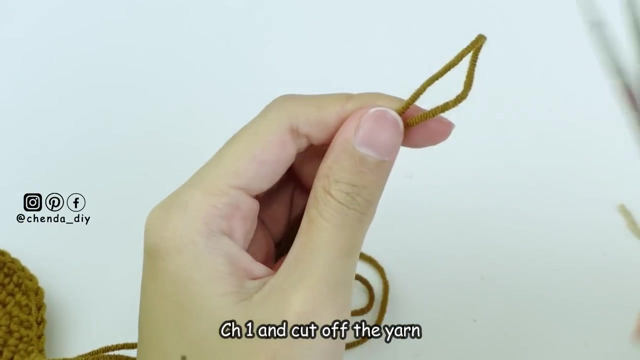 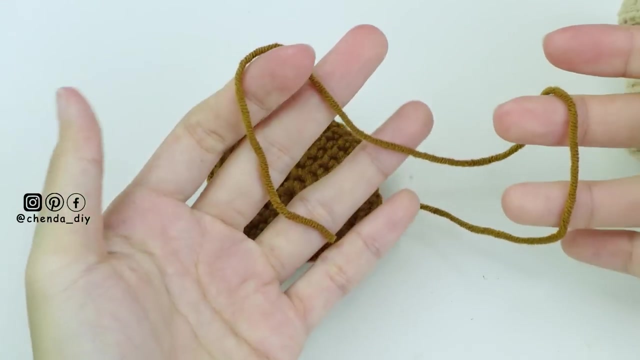 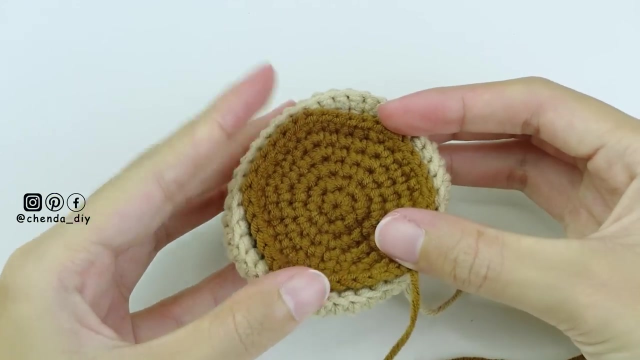 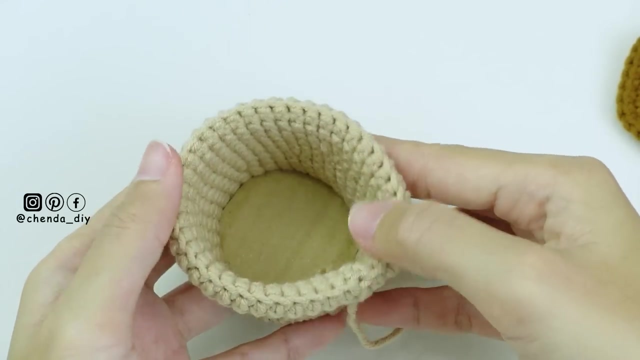 first single crochet stitch. After you have make slip stitch, then chain 1 and leave a long tail of yarn it keep for sewing and cut it off. Next we are going to sewing the cover of the pot into the pot. So first you have to make a half-circle from the both ends of the 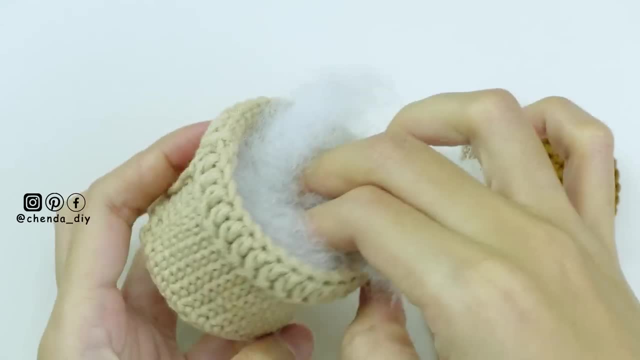 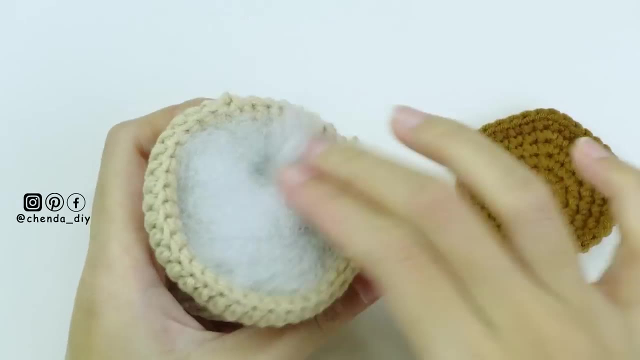 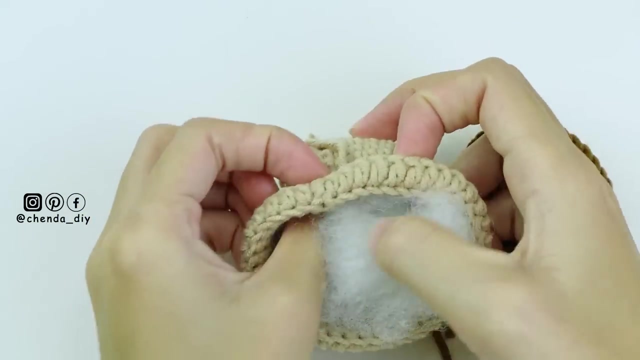 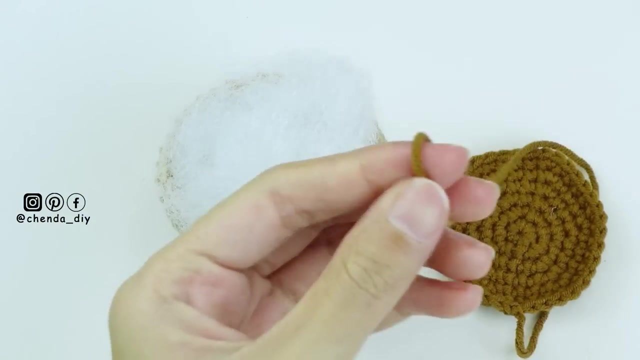 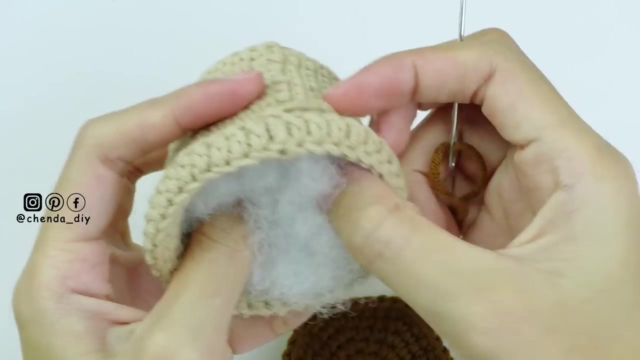 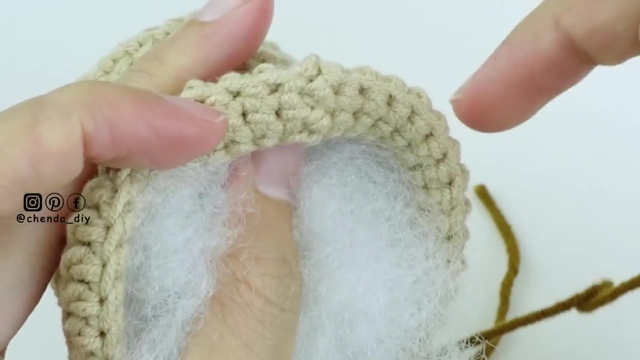 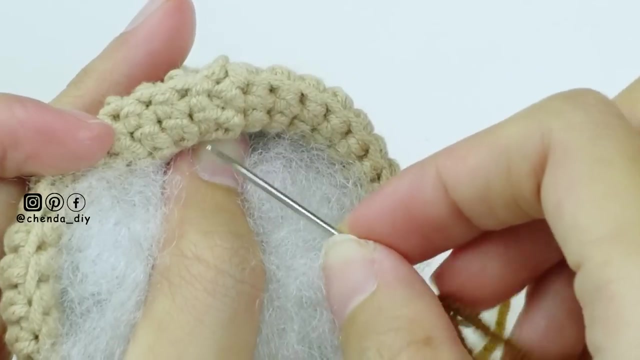 swap the entire on one side not to miss one row. Then you continue to cut the part from the other side to the head. After that you rest it, And done so, i'm going to skip the first row and insert the needle into the second row, as you can see. 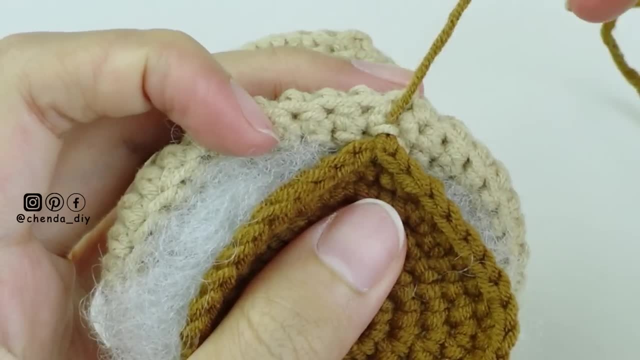 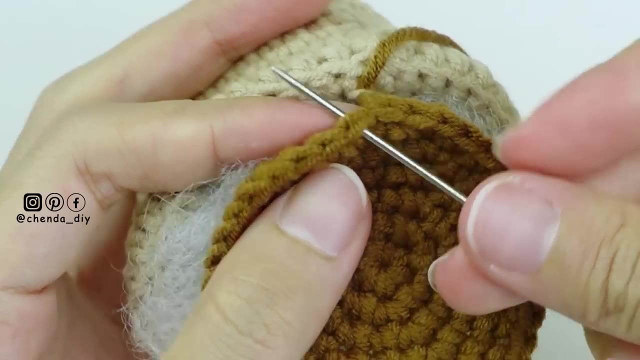 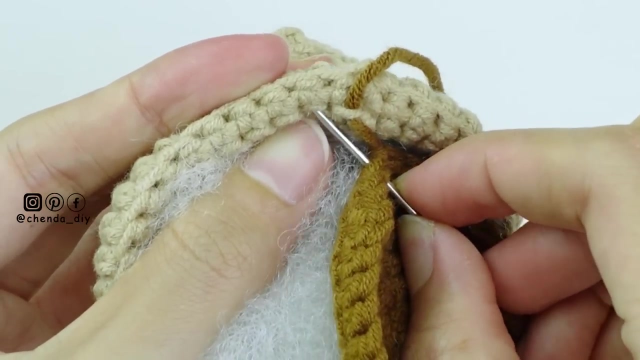 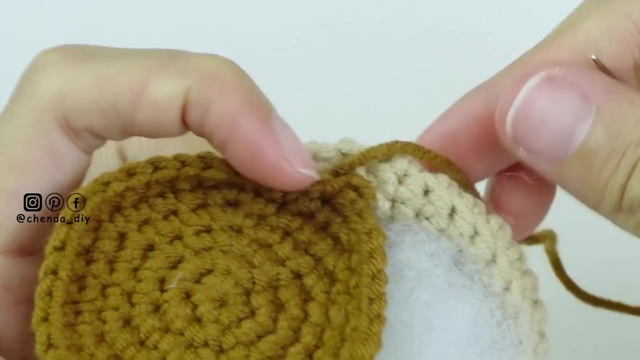 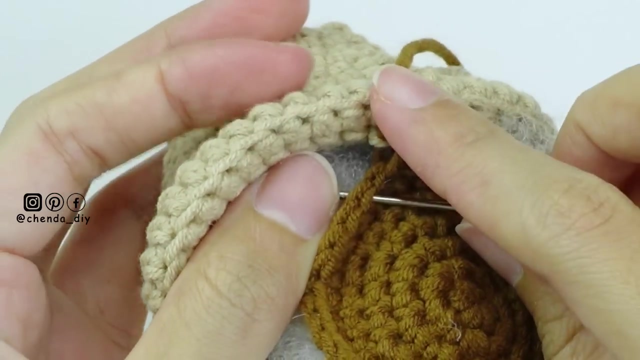 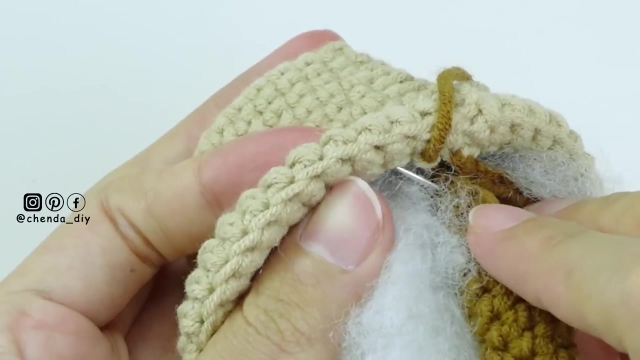 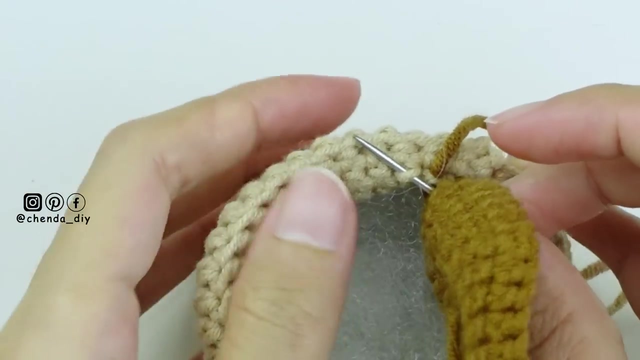 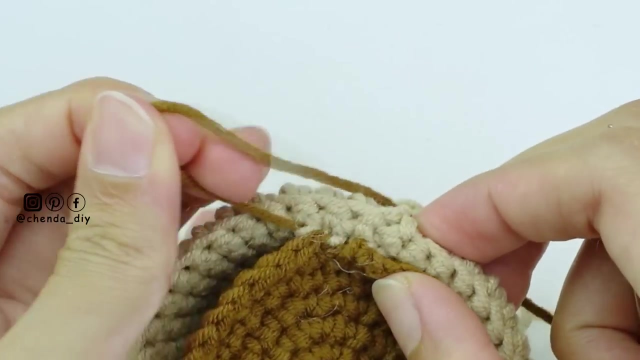 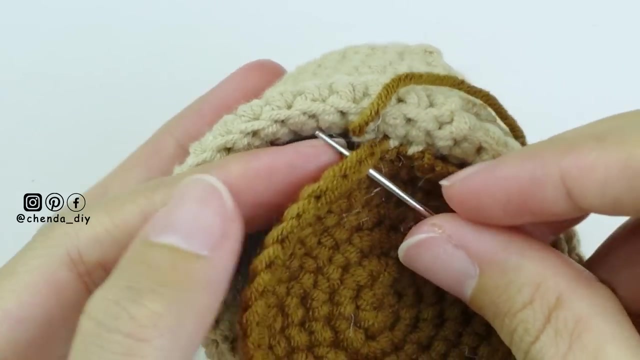 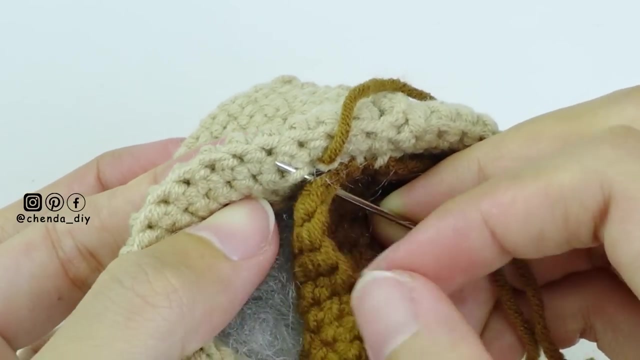 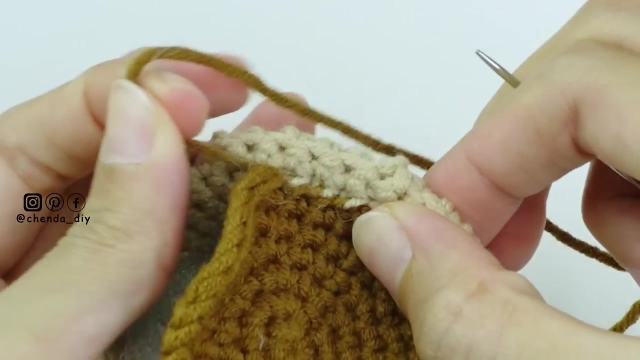 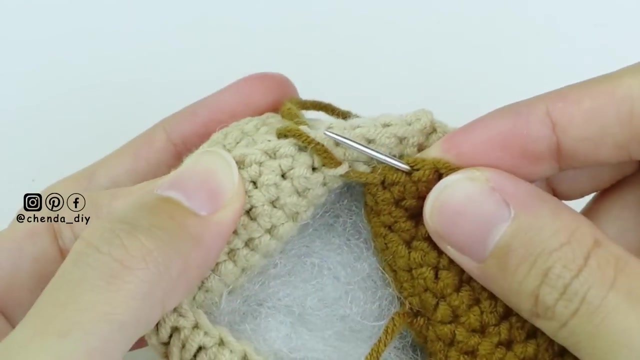 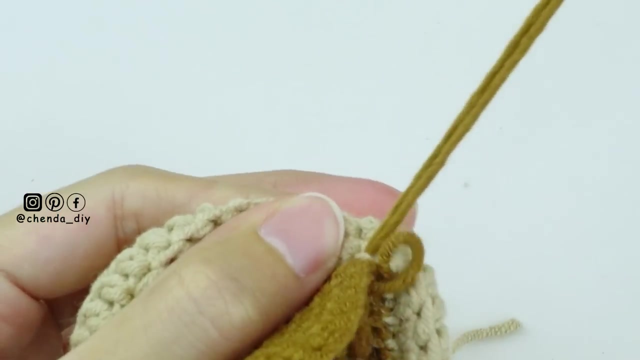 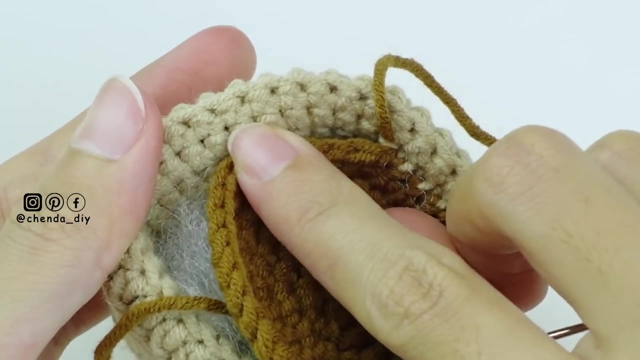 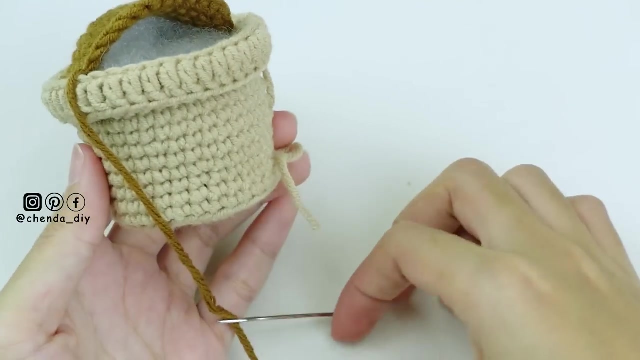 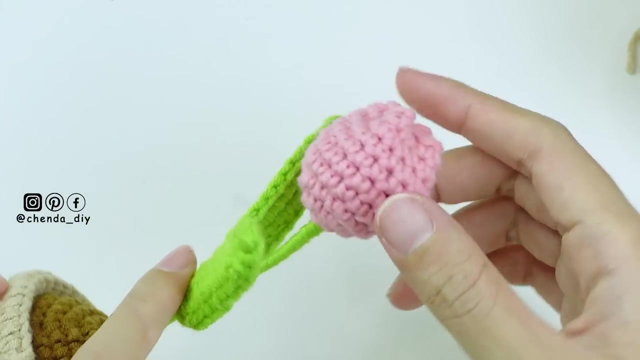 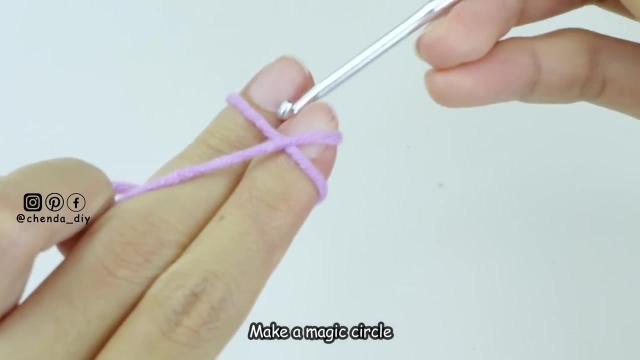 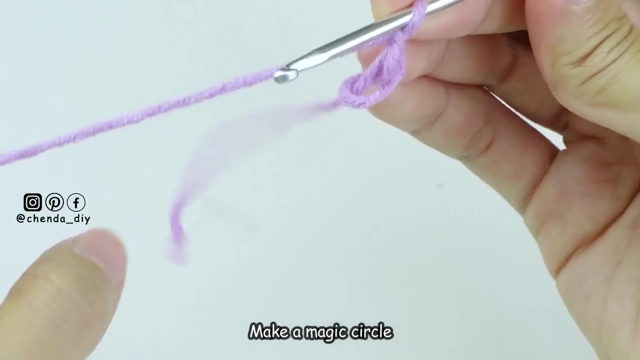 so, Thank you, Thank you, Keep sewing it around, but don't close it yet. You have to keep some space. And next we are going to make tulip flower To begin, make a magic circle And then make 6 single crochet into the circle. 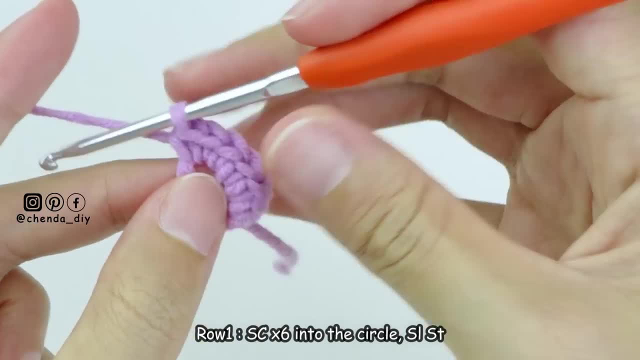 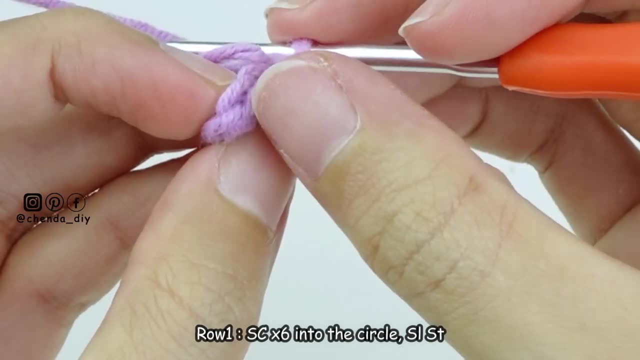 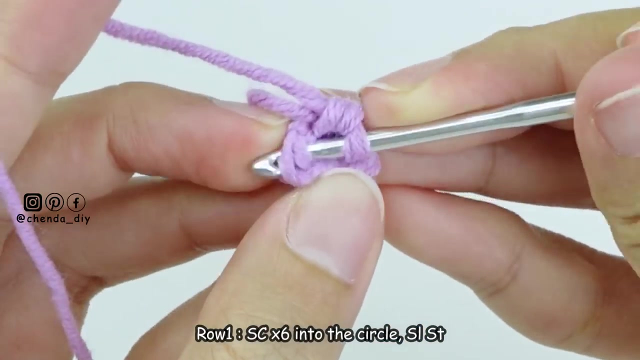 After you got 6 single crochet, then pull the short string of yarn tight to close the circle. And next we are going to continue, make slip stitch And then make 6 single crochet into the first single crochet stitch. Next for row 2, chain 1.. 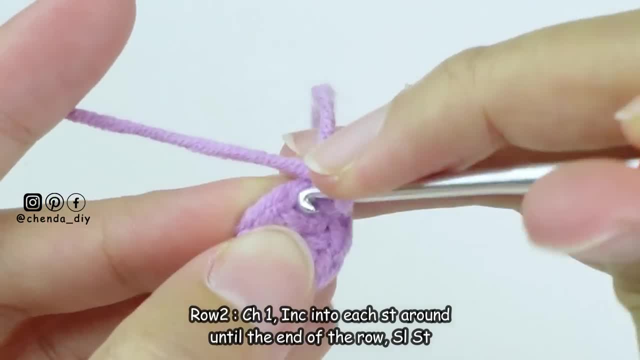 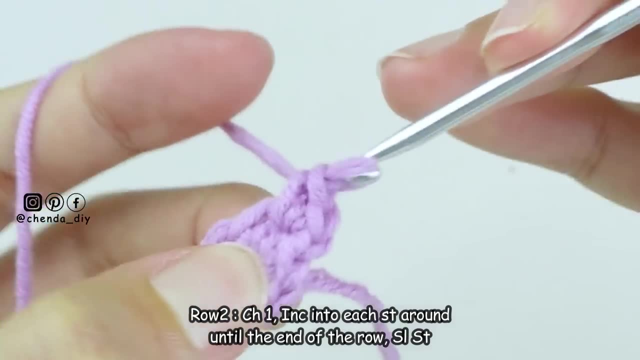 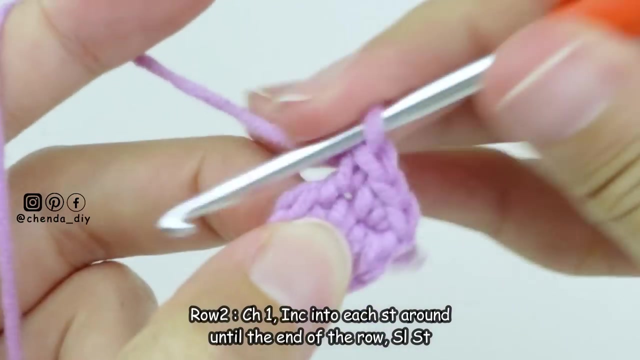 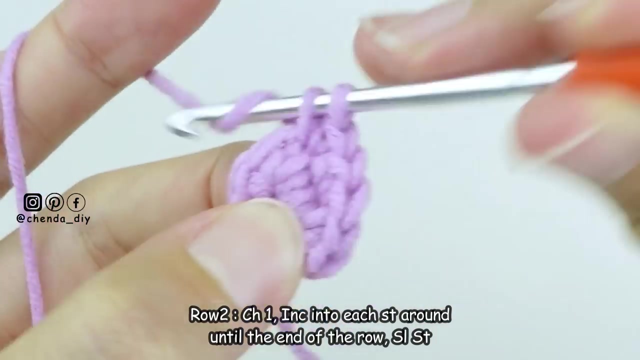 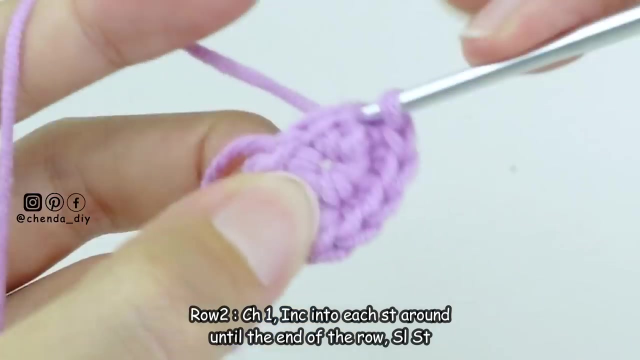 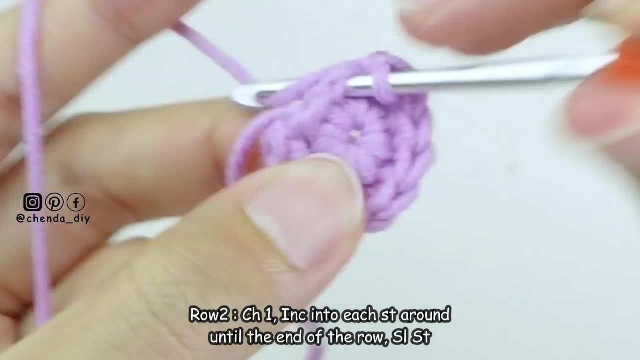 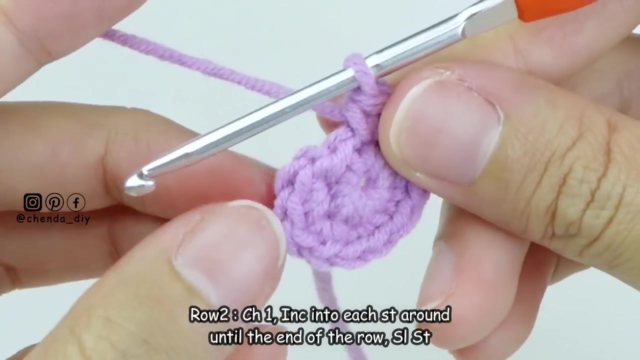 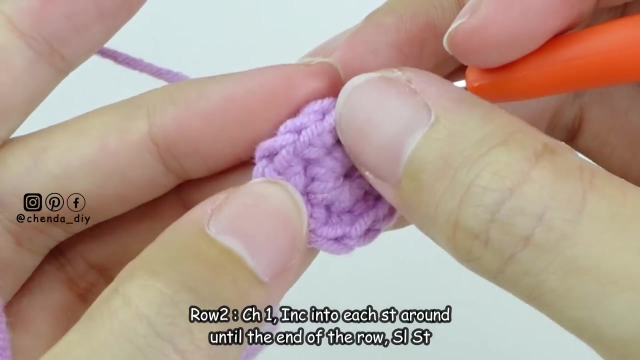 And make increase into each stitch around until the end of the row. Then we meet you back again, And we meet you back again Until you reach the end of the row. you must have 12 stitches of single crochet And then we are going to continue. make slip stitch into the first single crochet stitch. 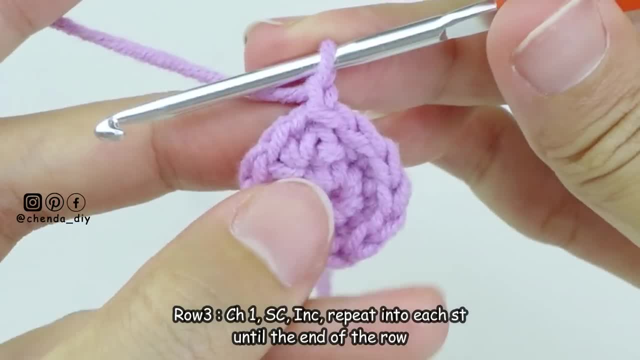 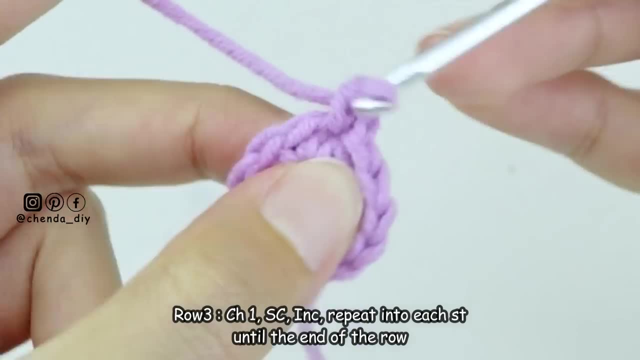 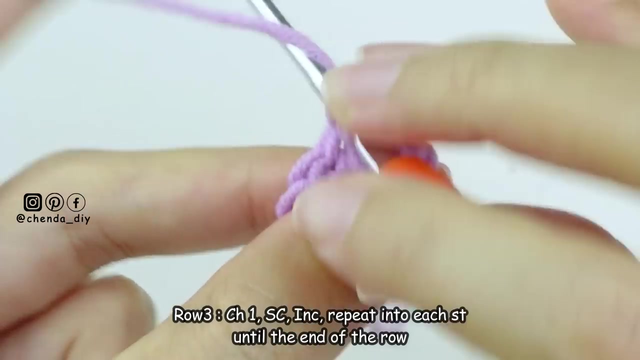 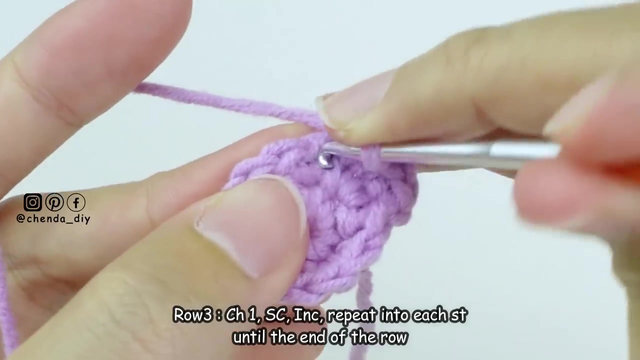 Next for row 3,, chain 1.. And make single crochet into the stitch near chain 1.. After you have made single crochet, then make increase. After you have made increase, then we are going to repeat the same thing by make 1 single crochet and then increase. 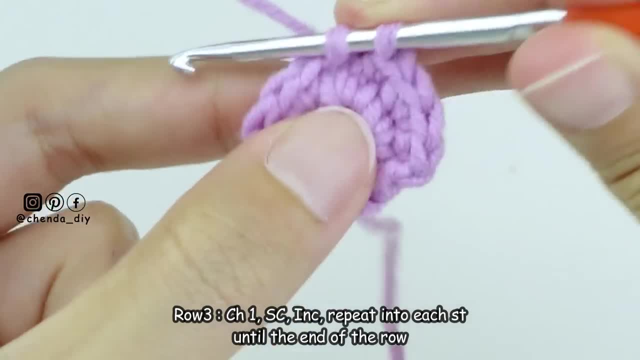 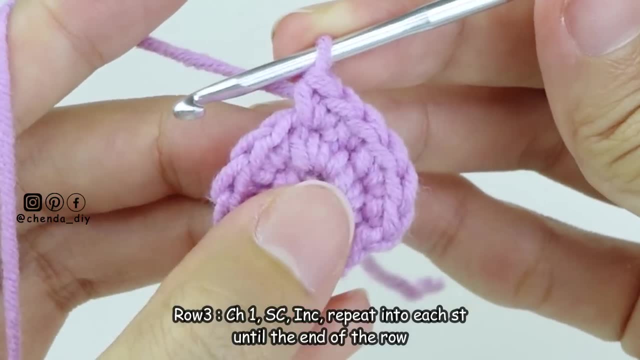 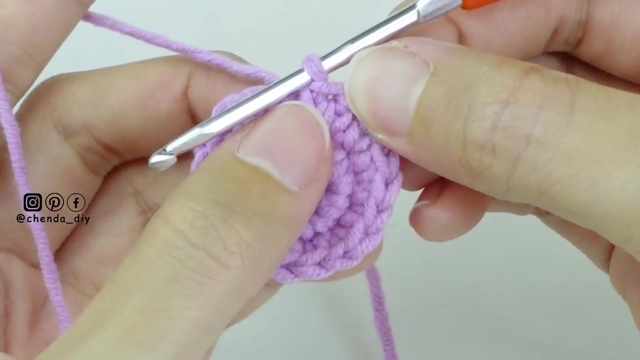 Until you reach the end of the row. then we meet you back again. After you reach the end of the row, you must end with increasing stitch And next you have to make a slip stitch into the stitch near chain 1.. You don't have to make slip stitch to connect the row. 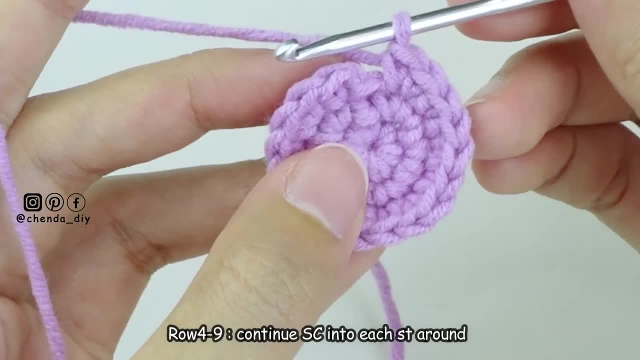 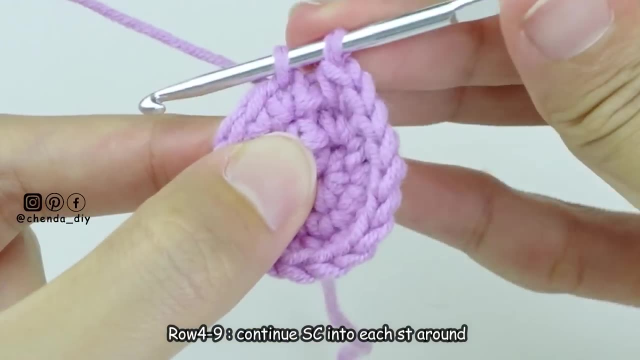 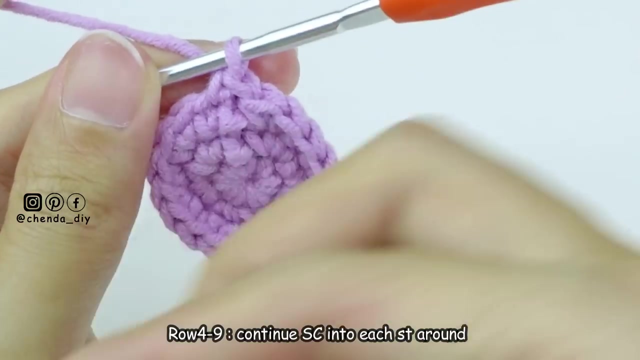 For the next, next row, start from row 4 until row 9.. Just continue, make single crochet into the first single crochet of row 3.. And then don't forget to use stitch marker to mark at this single crochet stitch. It is easy to know where to start the new row. 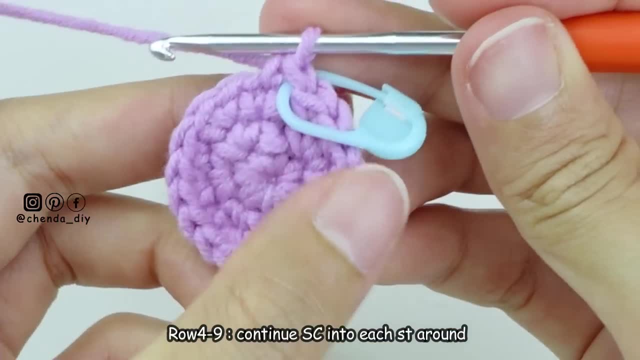 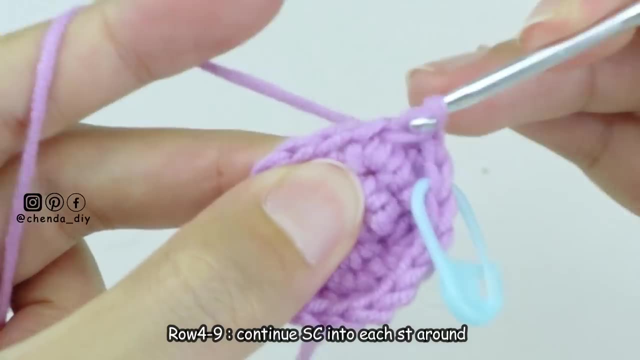 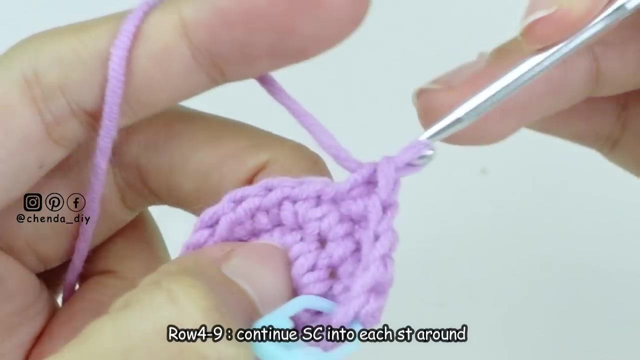 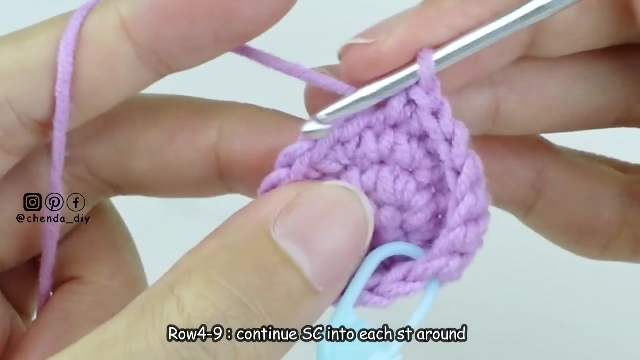 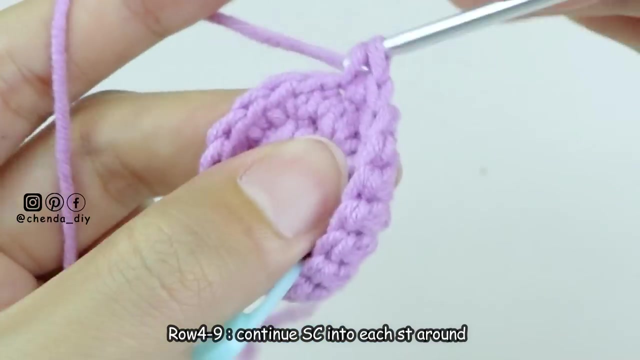 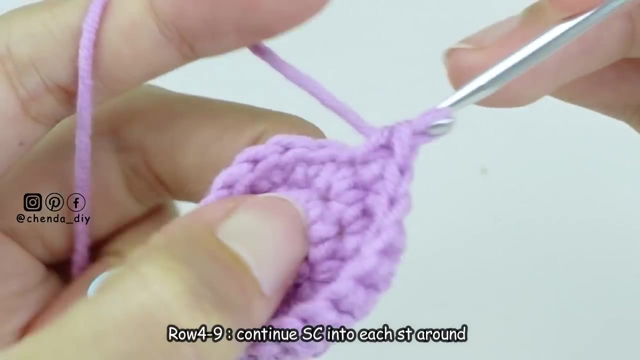 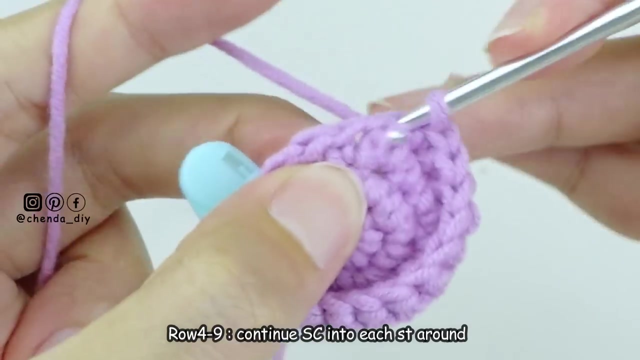 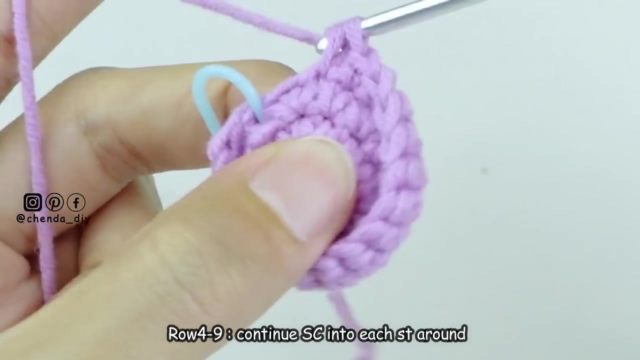 Keep making single crochet into each stitch around until you reach row 3.. Row 9, then we meet you back again. So start from row 4, we don't make increase, just make normal single crochet stitch around. Yes, So now the first one is a slip stitch into the stitch that became a double cross. 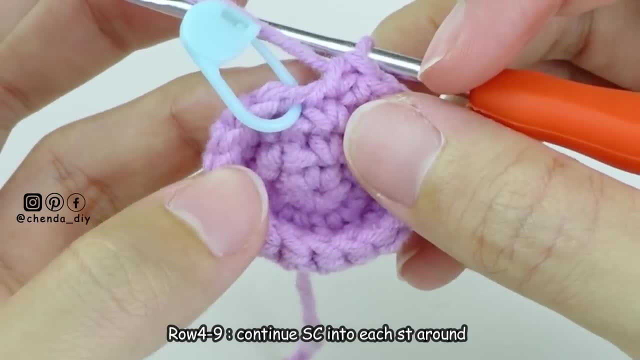 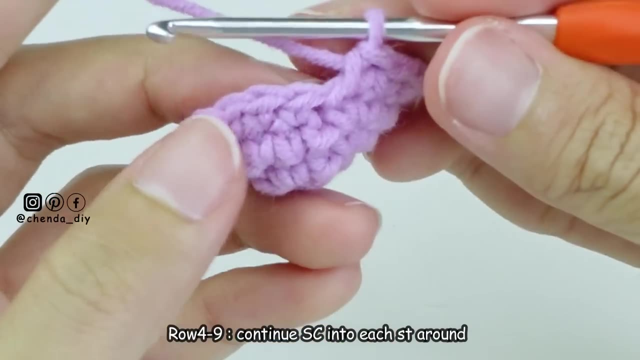 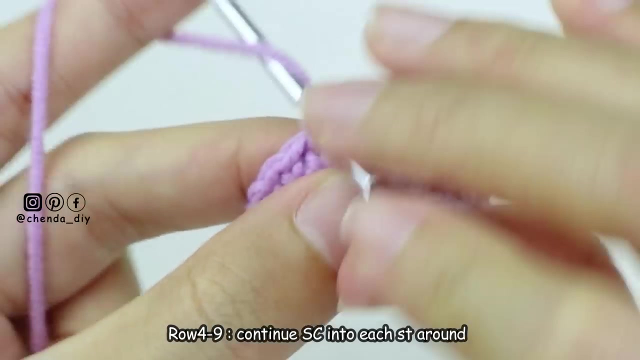 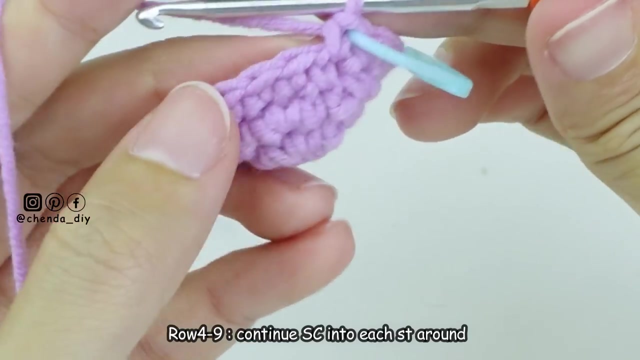 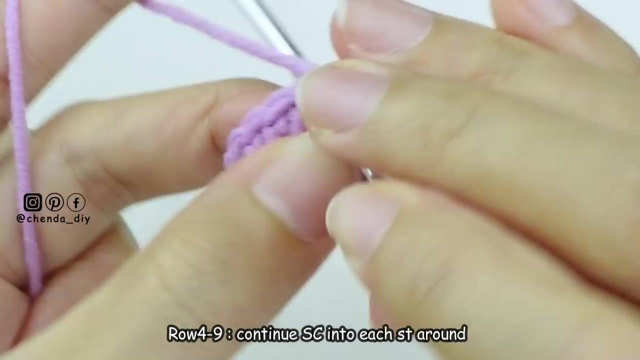 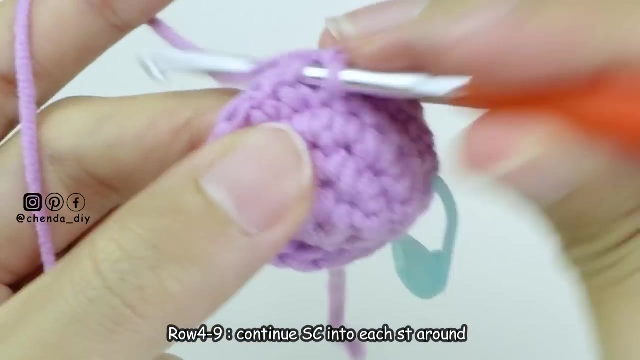 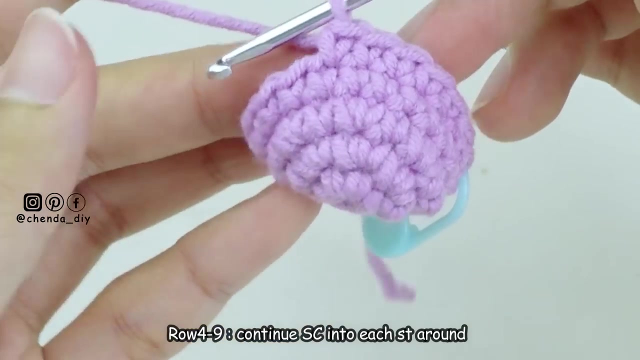 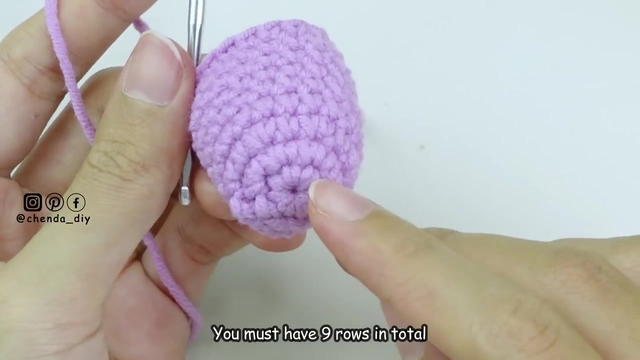 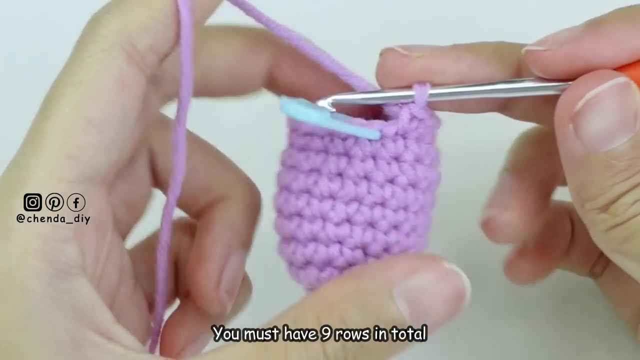 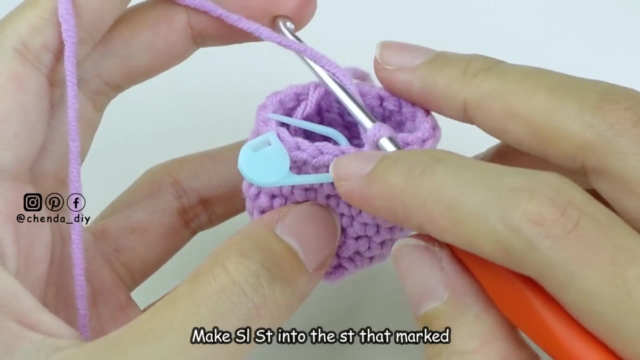 Next start from row 8,. we start with only 1 single crochet into each stitch around. Thank you, And this is what it looks like after you reach row 9.. In total, you must have 9 rows, And then we are going to continue: make slip stitch. 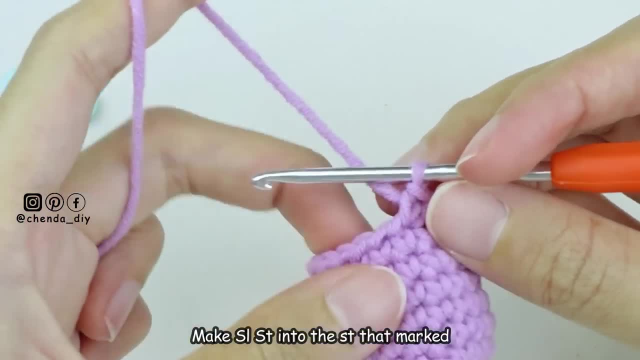 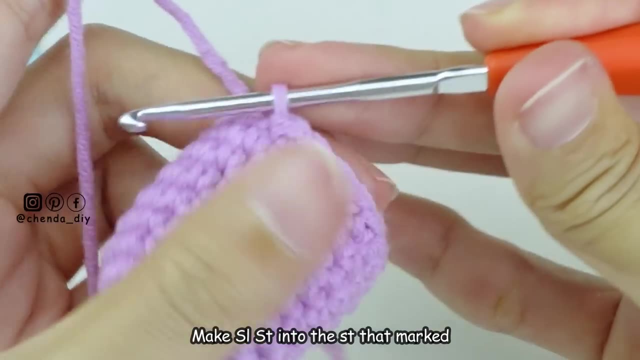 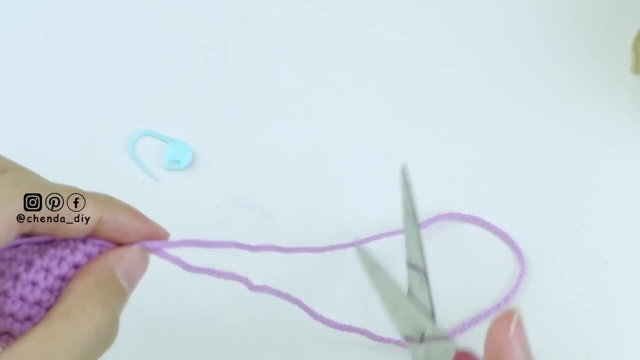 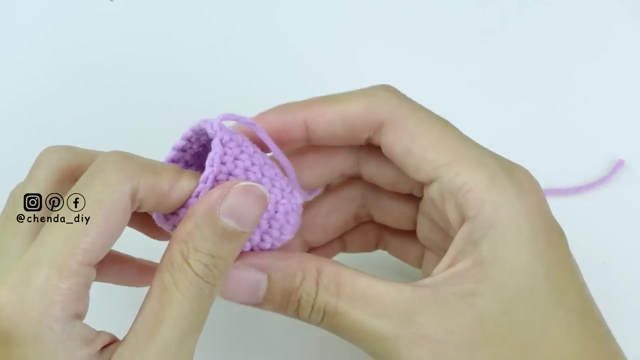 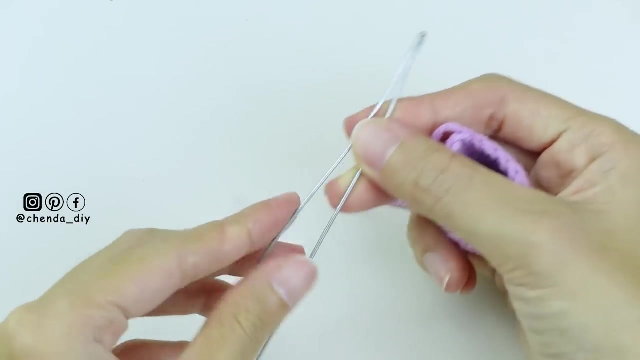 into the stitch After you have made slip stitch. then leave a long tail of yarn it keep for sewing and cut it off. Then cut the wire for 12 inches and fold it in half. Then fold it into two pieces like this. We use it as a stem of the tulip. 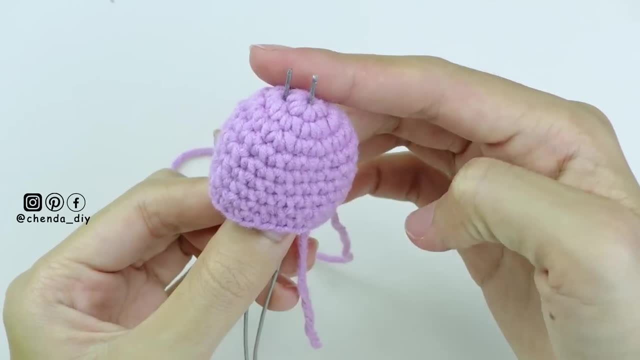 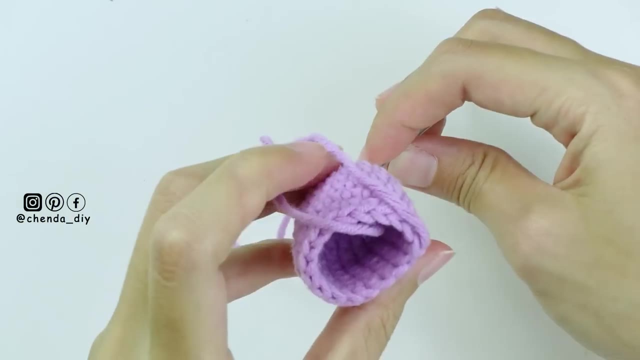 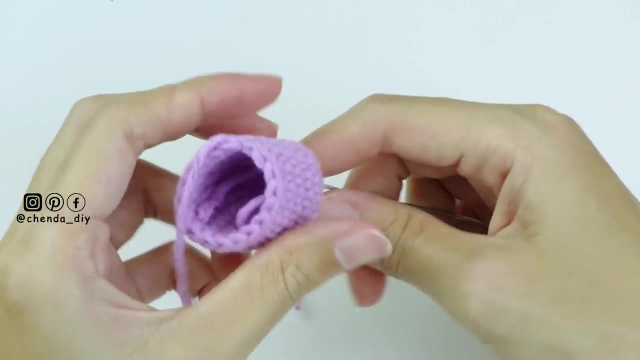 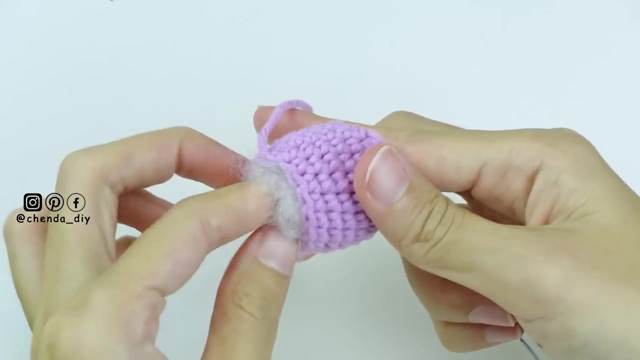 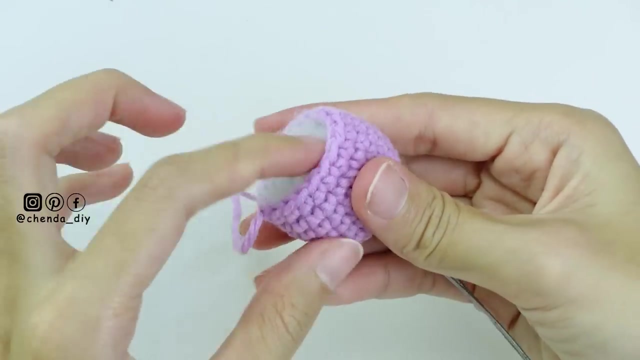 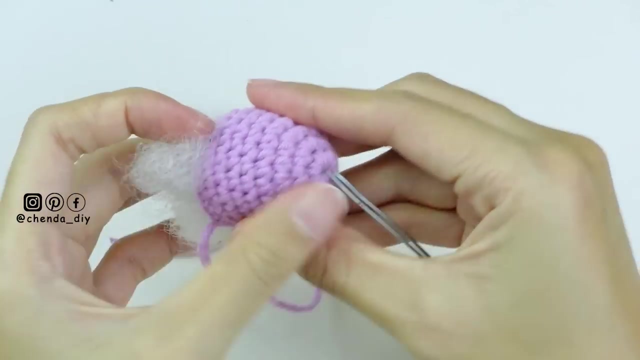 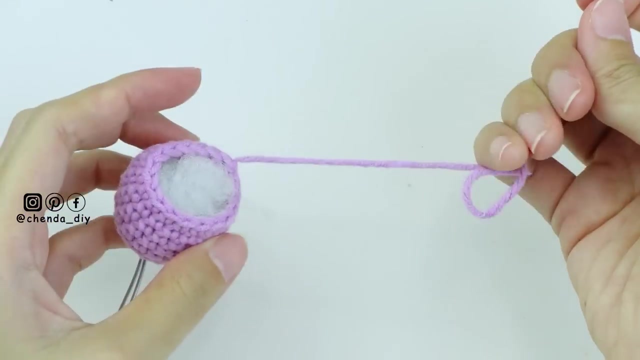 We use it as a stem of the tulip. We use it as a stem of the tulip, Adding the toy, stuffing as much as you can to make the tulip look fluffy, to make the tulip look fluffy. to make the tulip look fluffy. 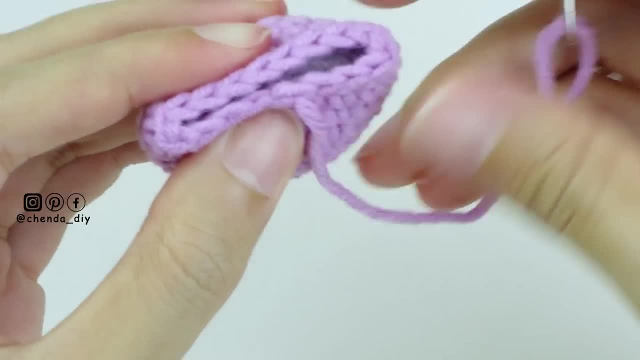 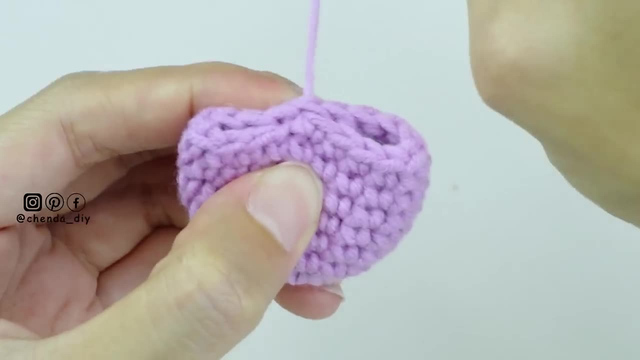 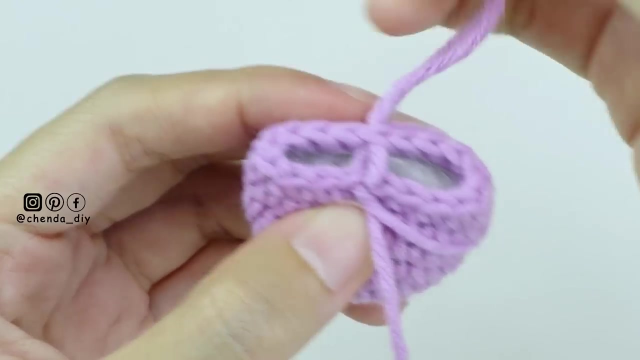 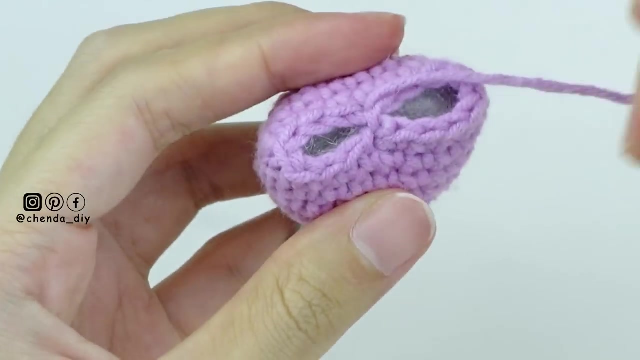 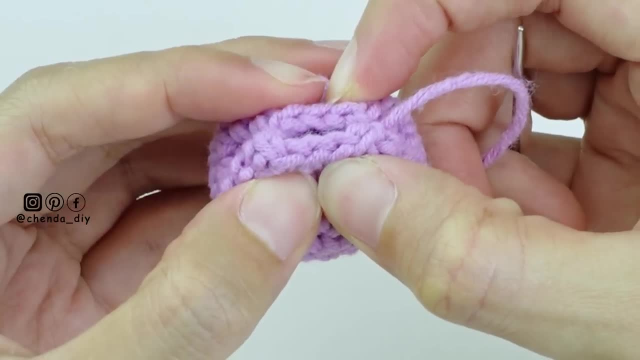 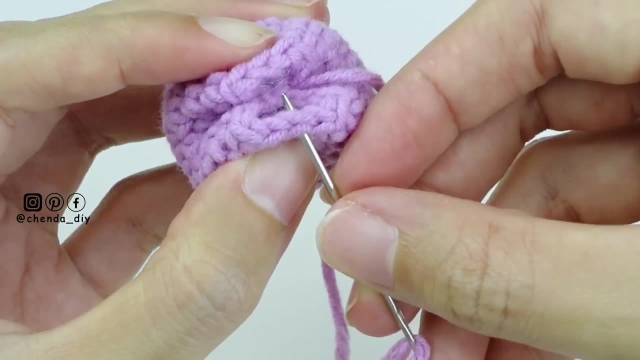 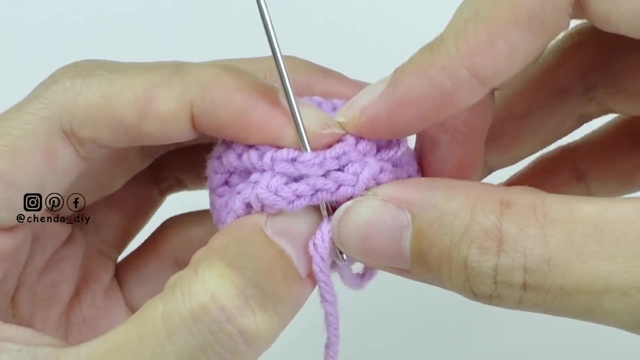 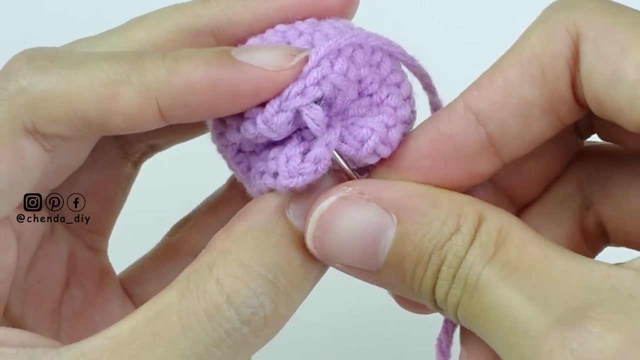 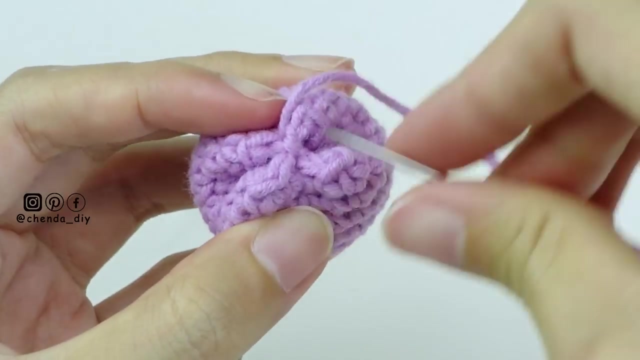 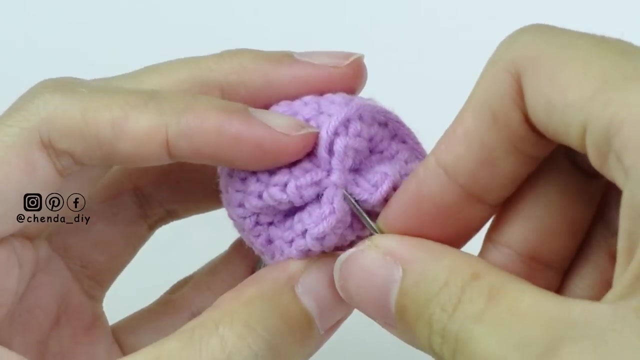 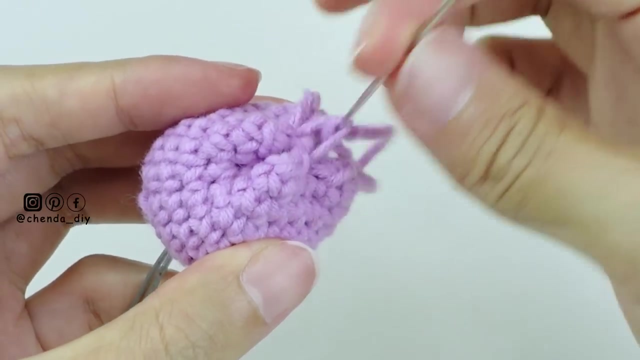 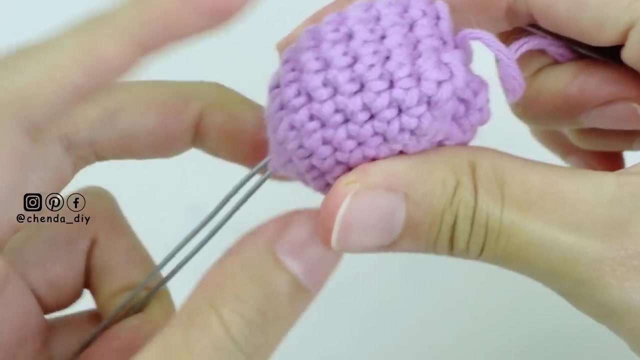 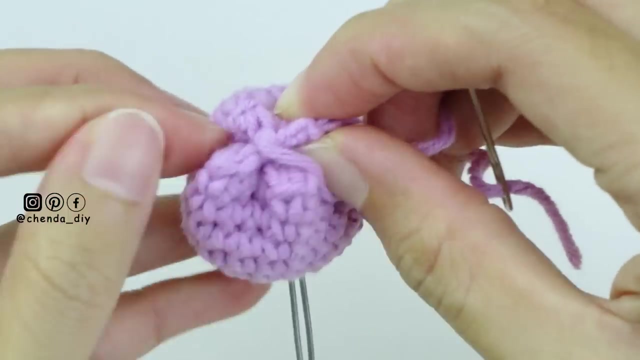 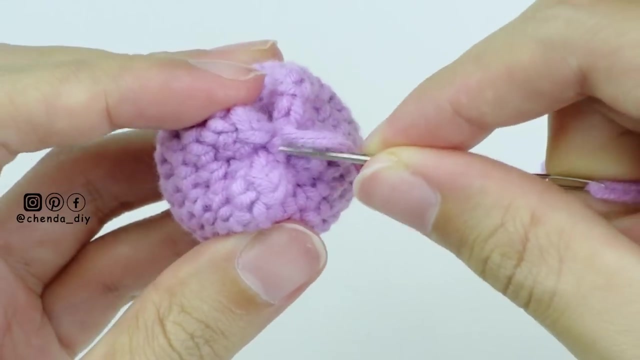 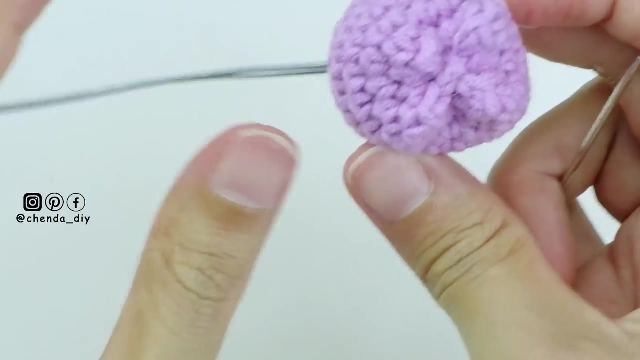 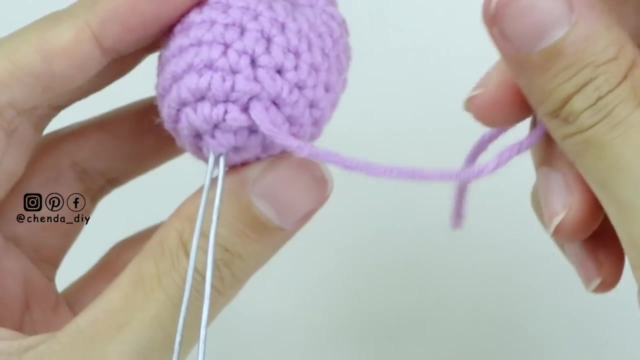 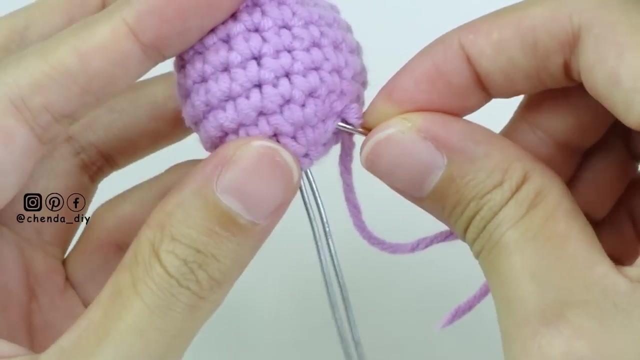 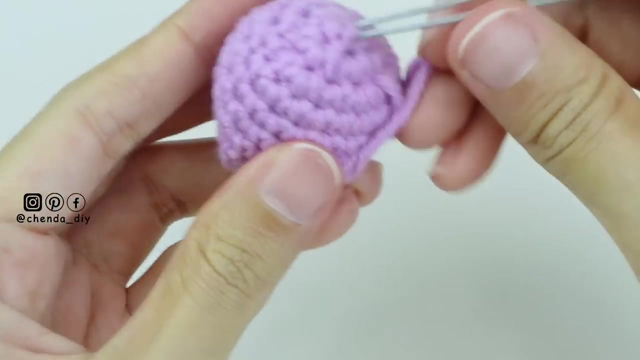 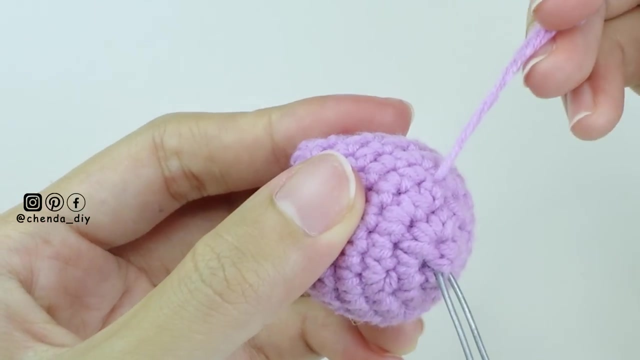 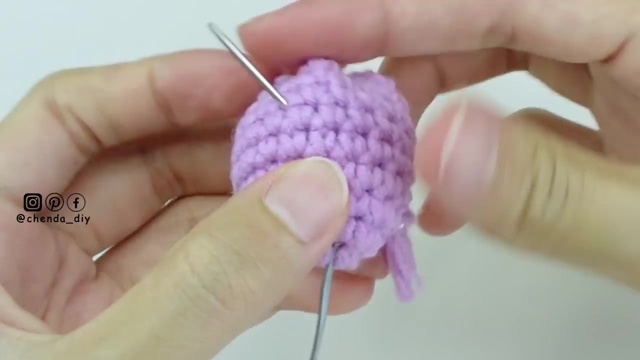 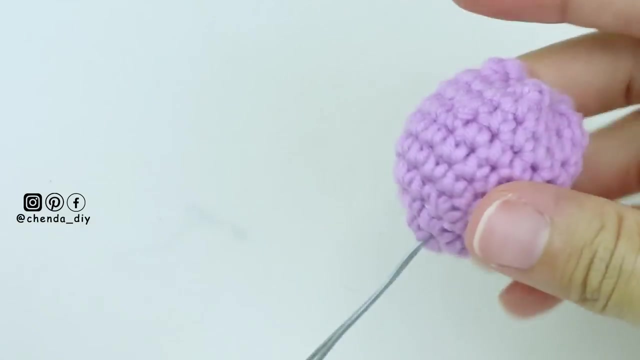 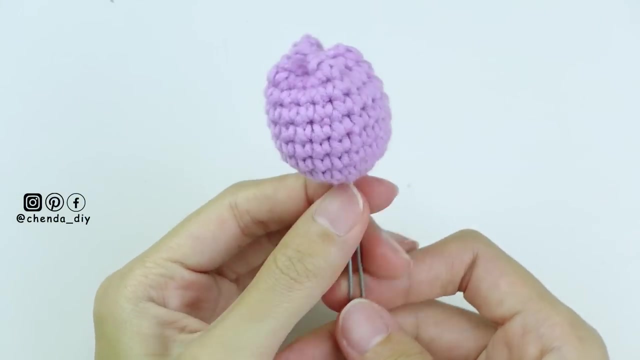 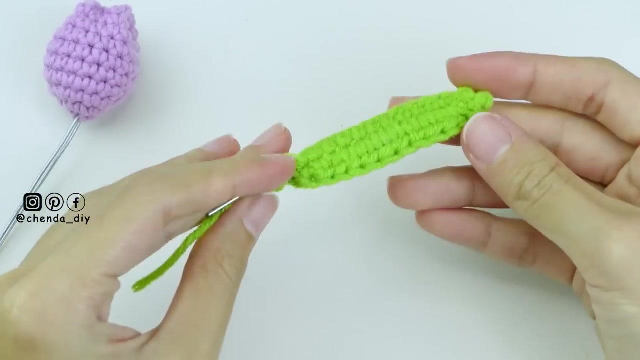 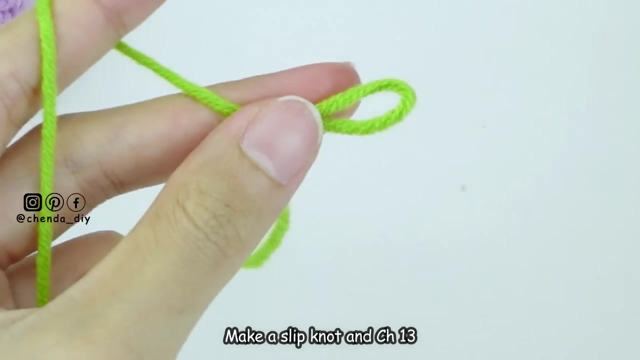 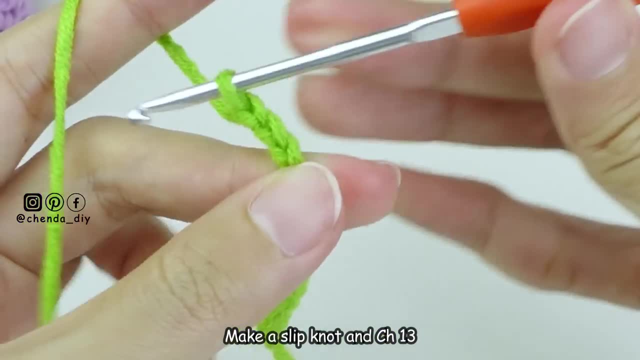 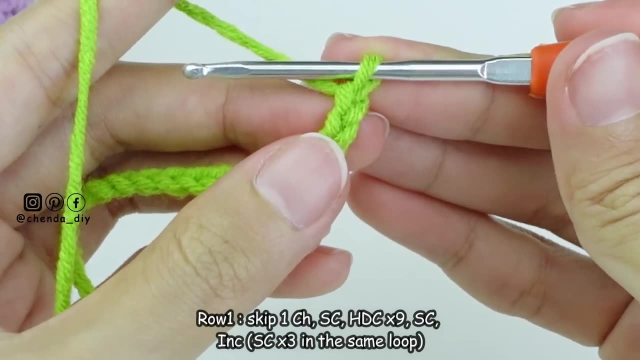 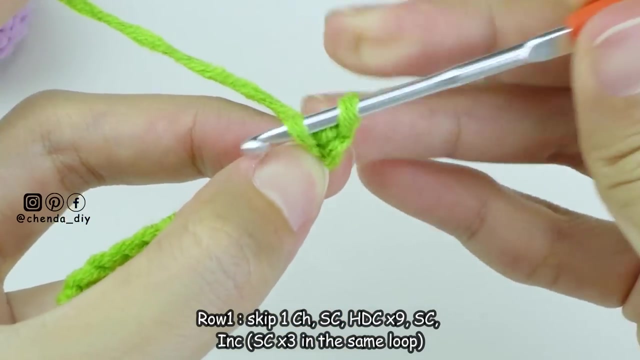 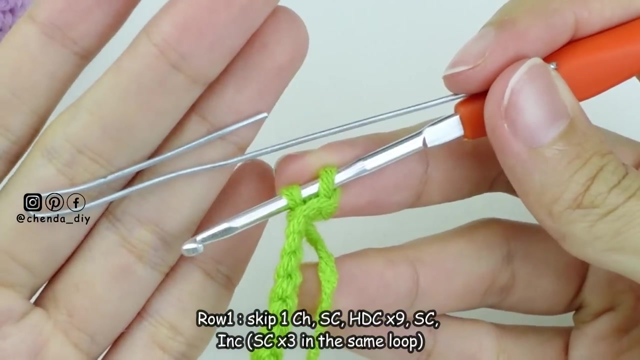 After you got certain chains, next for row 1, skip 1 chain and make single crochet into the next chain And then bring the wire that we cut for 7 inches and fold it in half like this, And we are going to make single crochet. 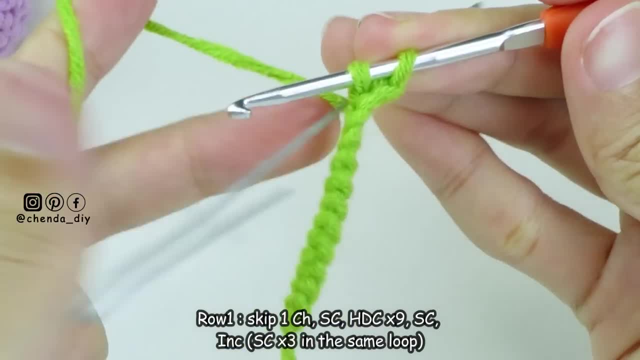 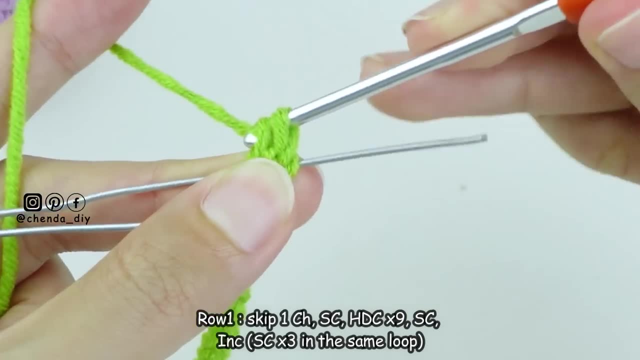 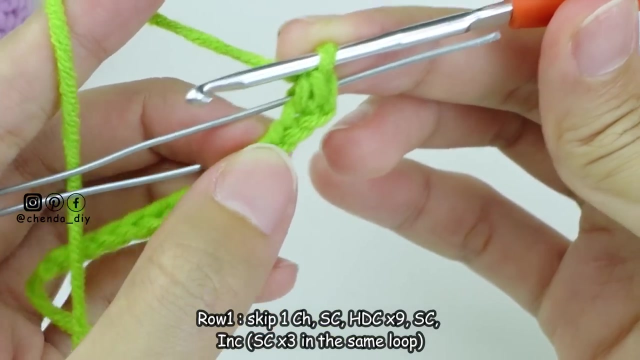 and carrying this along with the row By placing the wire on top of the yarn and yarn over, pull through 2 loops And now, as you can see, the wire is inside the stitch. Next, we are going to make half the bokeh shade. 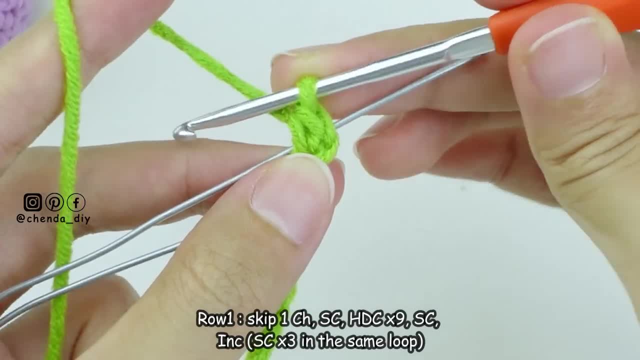 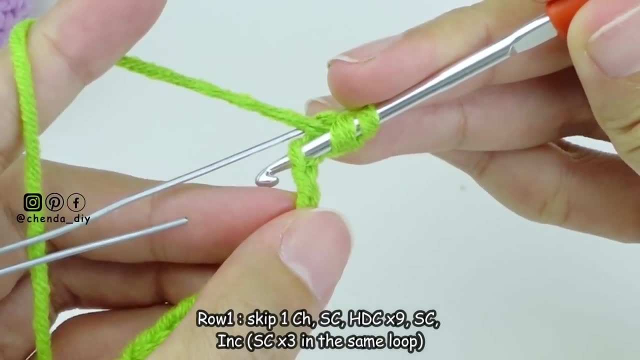 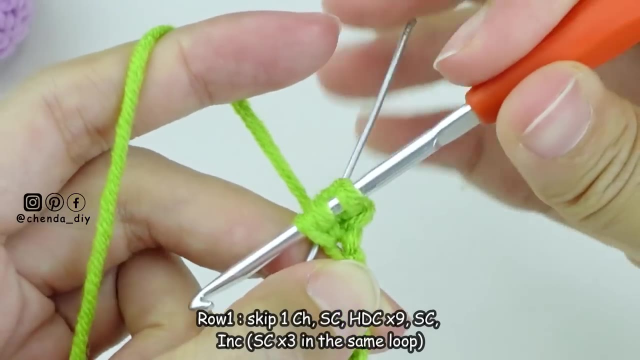 into the next chain To make half the bokeh shade yarn over. insert the hook into the loop and then place the wire on top of the hook, yarn over and pull up a loop And now you have 3 loops on your hook. 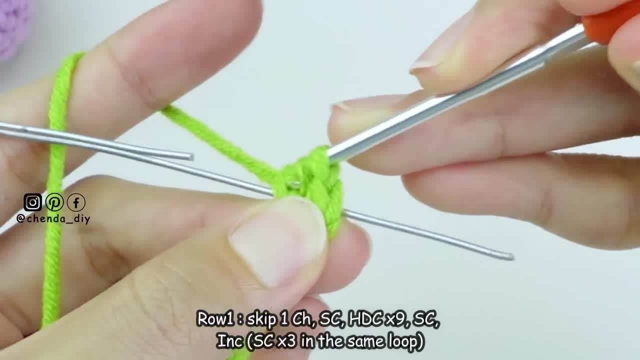 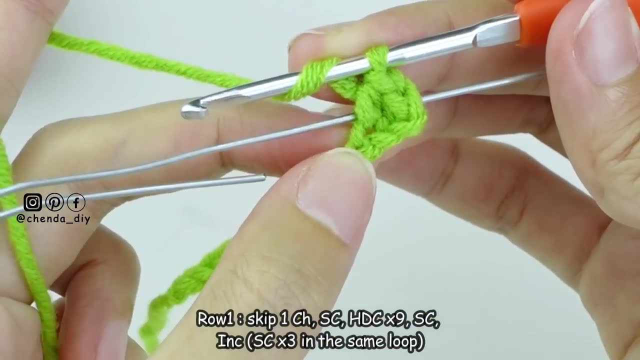 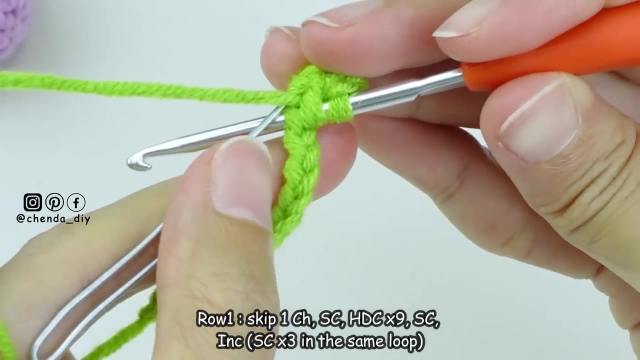 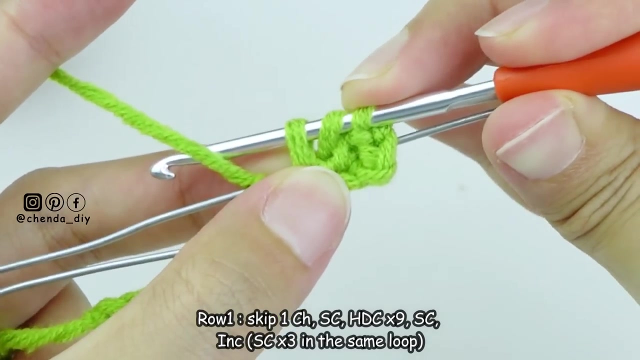 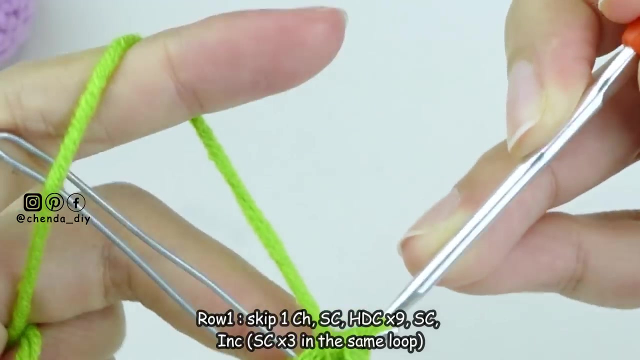 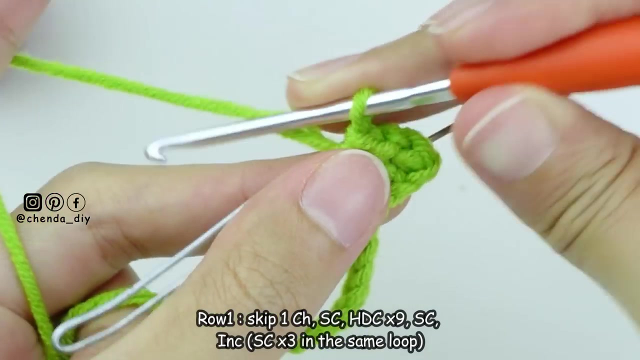 Yarn over and pull through all 3 loops. Keep making half the bokeh shade into every chain until you have 2 last chains. Then we meet you back again. If you have any questions or suggestions, feel free to ask them in the comments. 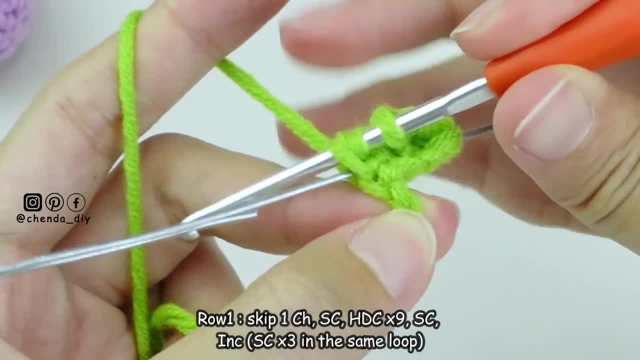 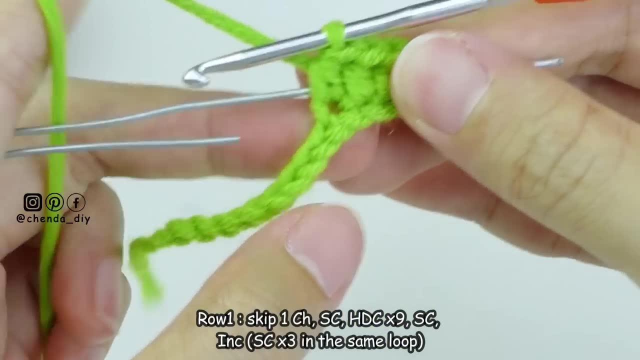 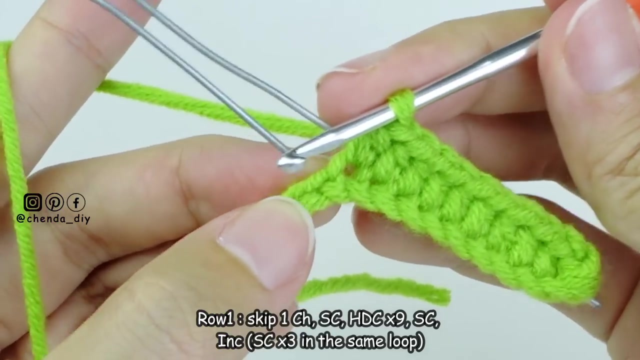 Thanks for watching this video, END. If you enjoyed it, please like, subscribe and share it with your friends. Join the crew for more videos. Bye, Bye. After you have 2 last chains, then we are going to make single crochet. 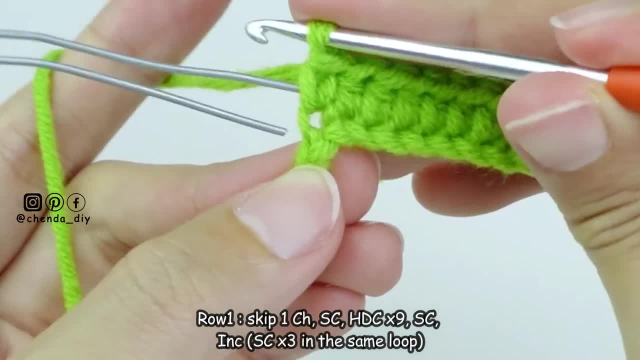 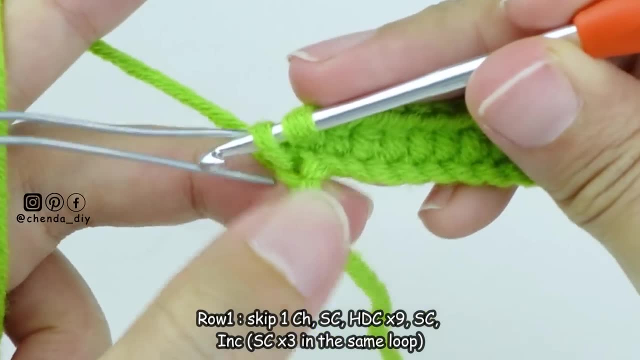 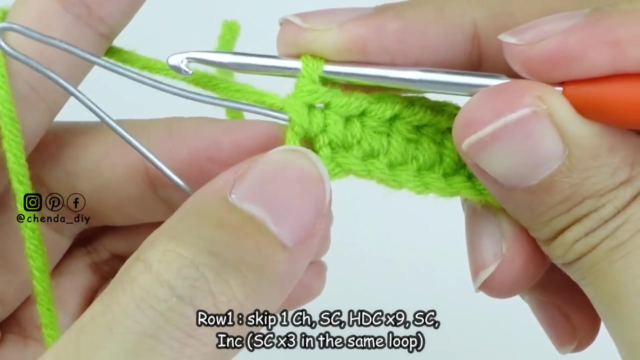 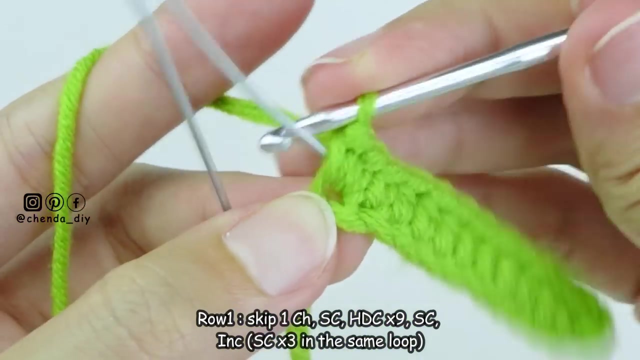 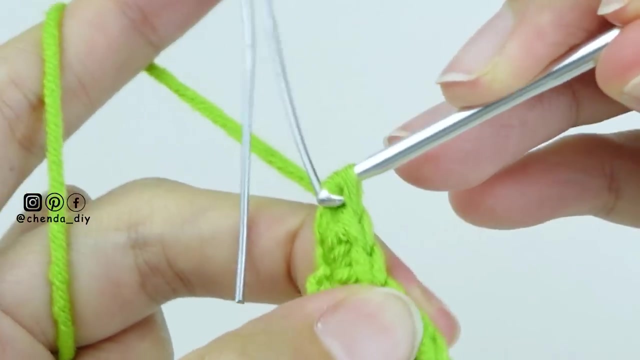 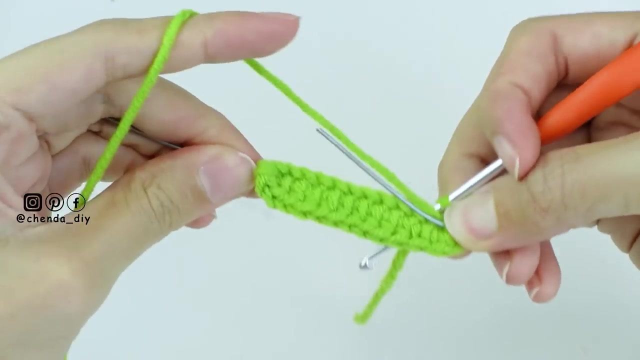 After you have made a single crochet for the last chain, we are going to make increase by make 3 single crochet in the same loop. After you got 3 single crochet in the same loop, then pull this increasing stitch onto the top of the wire. 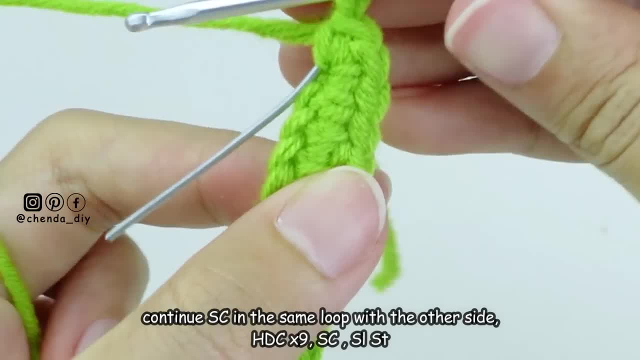 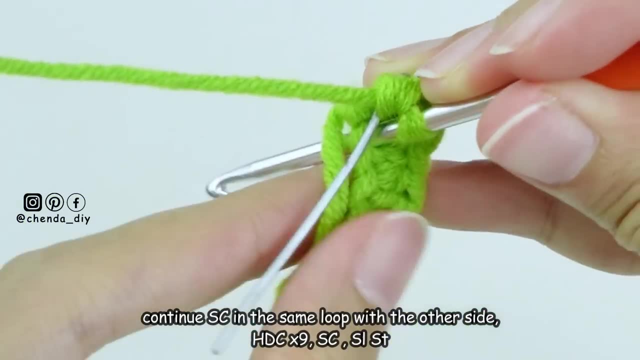 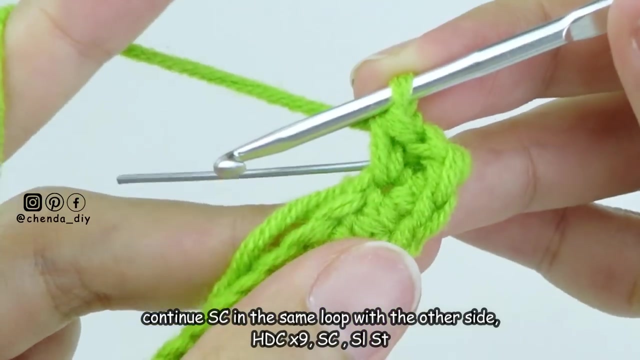 And next we are going to make this other side of the leaves To begin, make single crochet with the other side stitch, Make sure that the wire and this tail of yarn is on top of the hook. We are going to carry them along with the row After you have made a single crochet and then make half double. 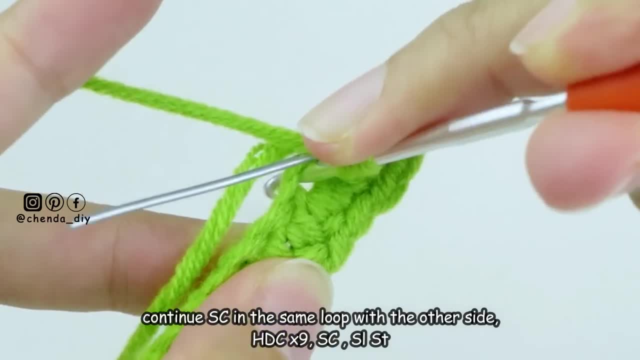 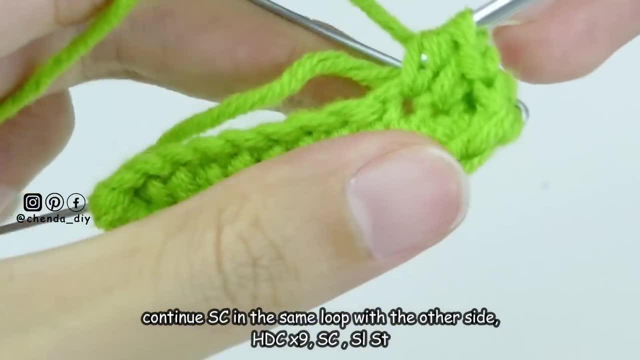 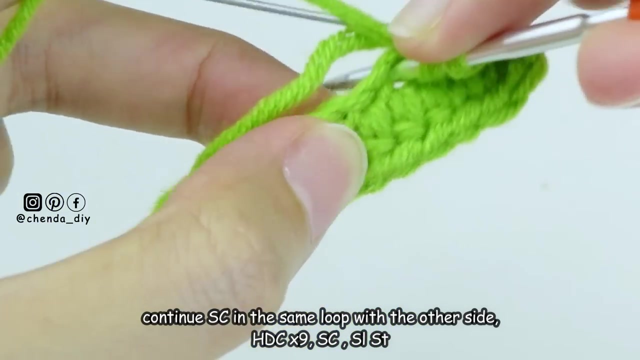 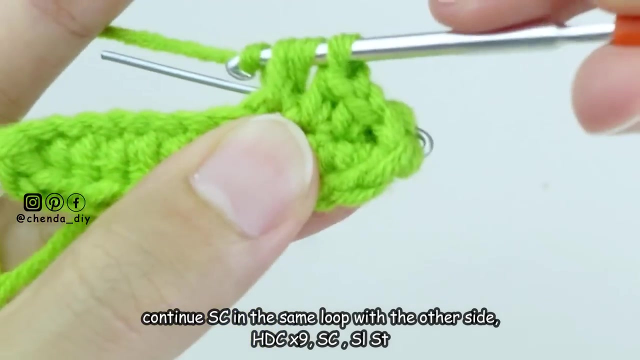 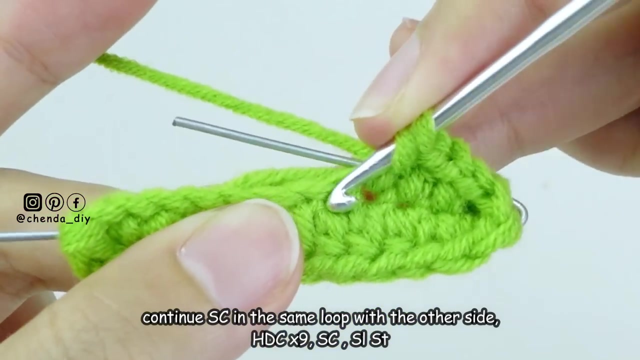 crochet into each stitch until you have 1 last stitch. then we meet you back again and make a double crochet in the same loop, And now we are going to make another single crochet and pull behind the right end of the last stitch. So that's what we have got. 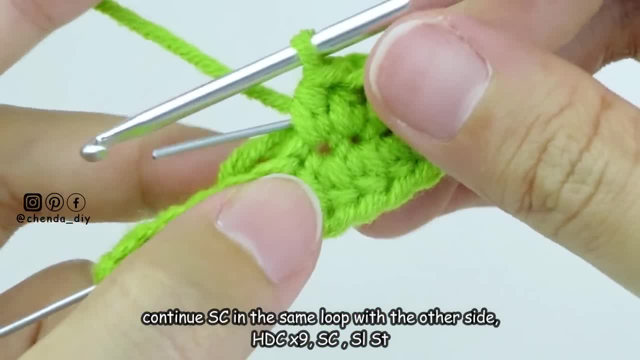 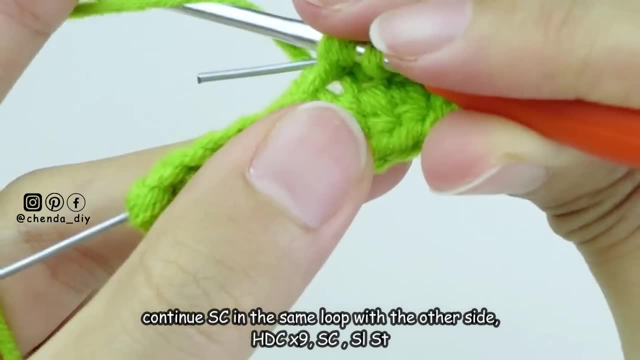 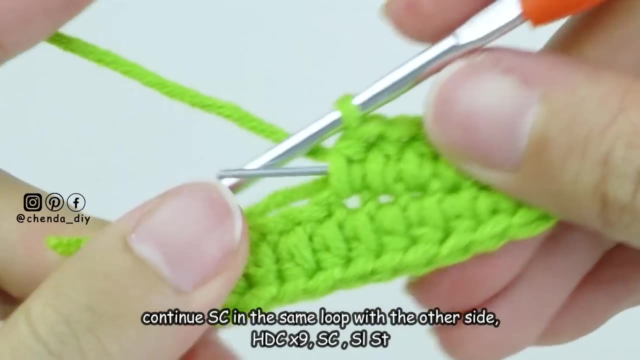 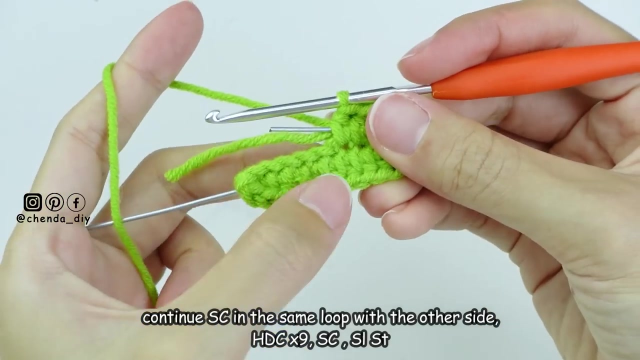 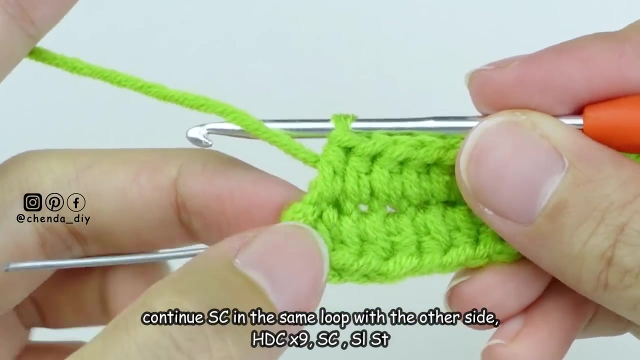 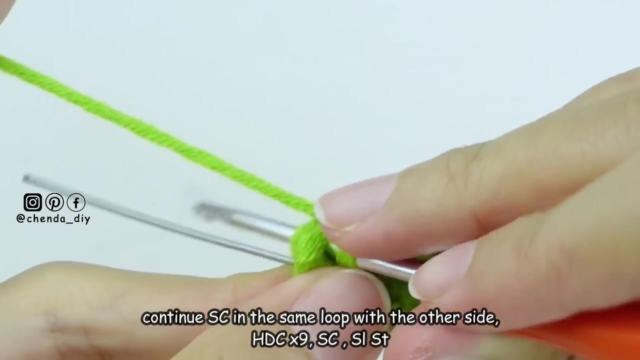 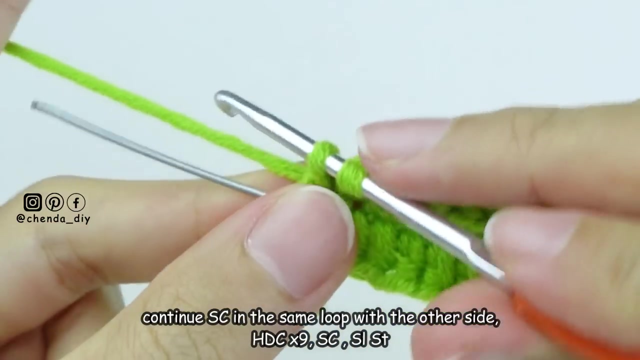 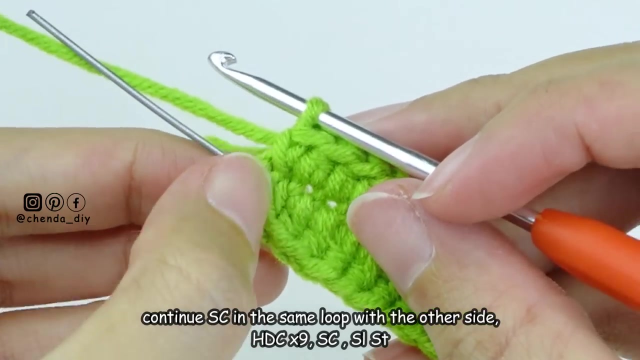 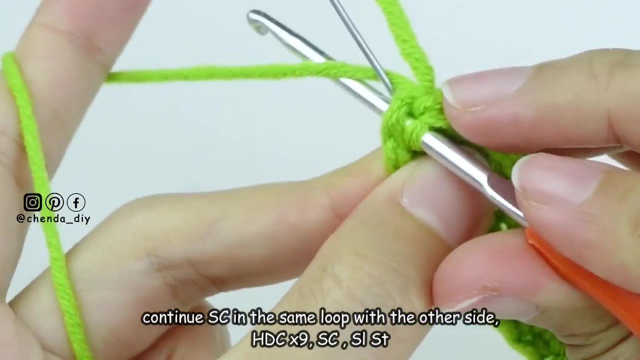 After you have made a single crochet, push up the left chain. After you have one last stitch, then we are going to make single crochet. After you have a single crochet, then continue, make slip stitch into the first single crochet stitch of the other side. 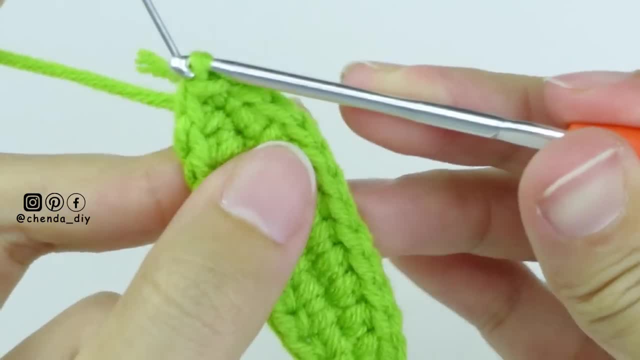 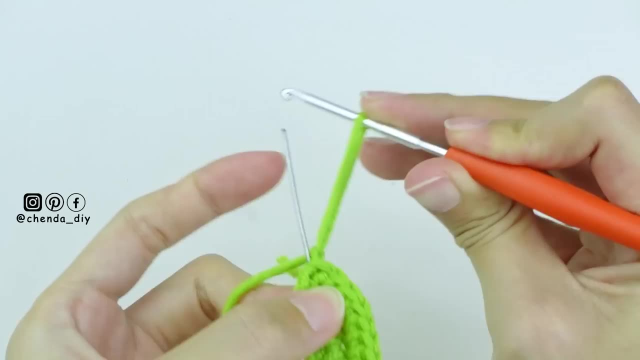 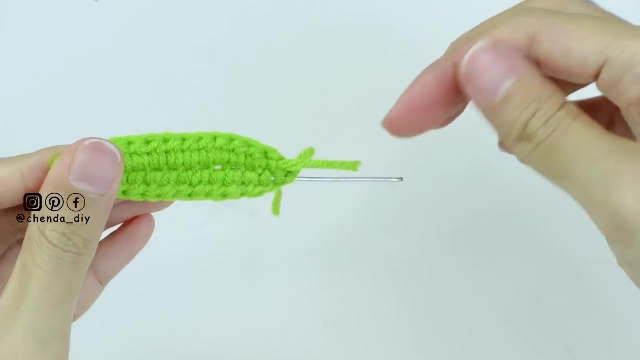 After you have made a single crochet, then continue, make slip stitch into the first single crochet stitch of the other side. After you have made a slip stitch, then make another slip stitch and cut off the yarn. And now we are done for the leaves. don't forget to repeat the same thing to the other leaf. 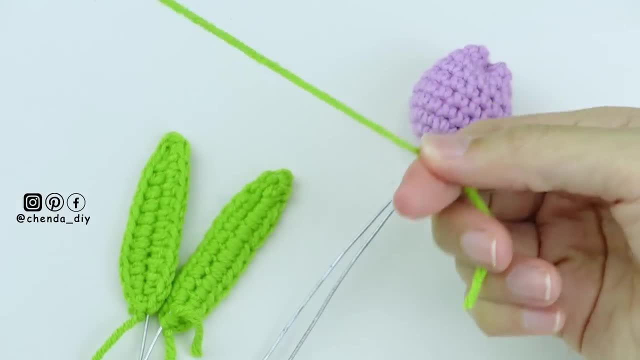 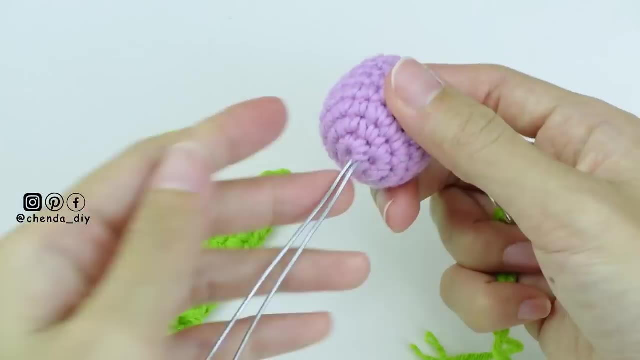 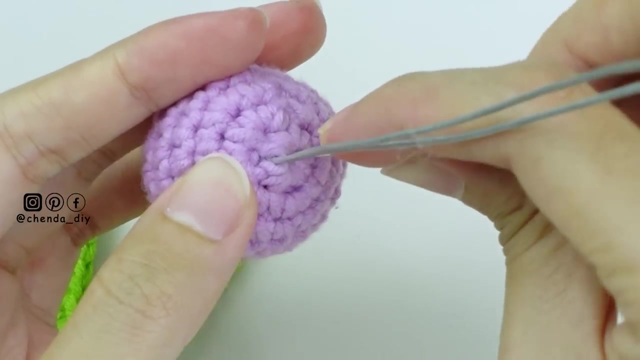 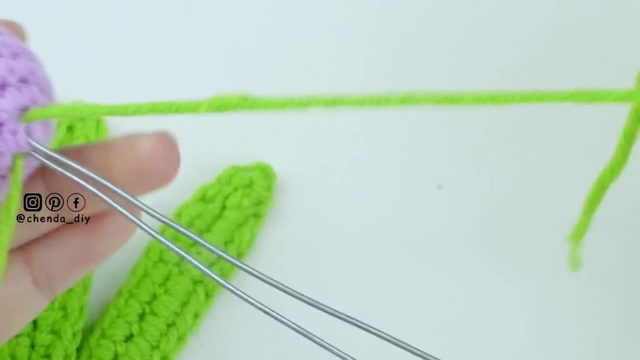 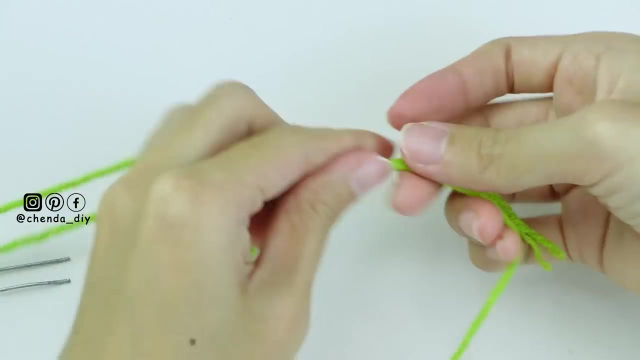 Next we are going to attach the leaves with the stem. To begin, you have to attach the green yarn into the bottom of the tulip And then leave both strings long enough. It keeps 4 wraps around the stem, which is the wire, Then cut it off. 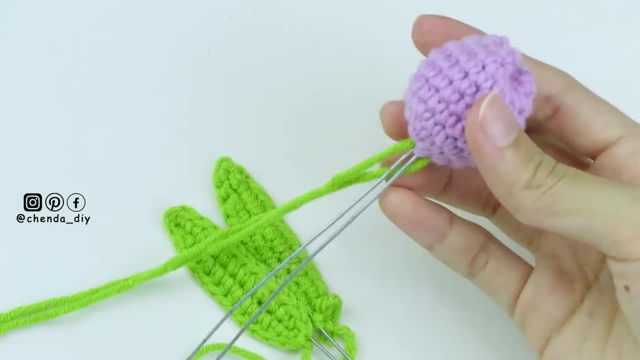 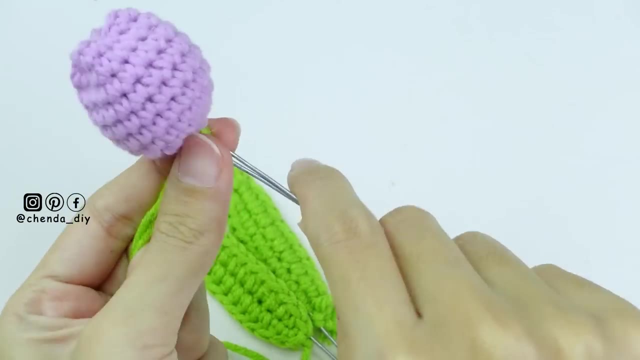 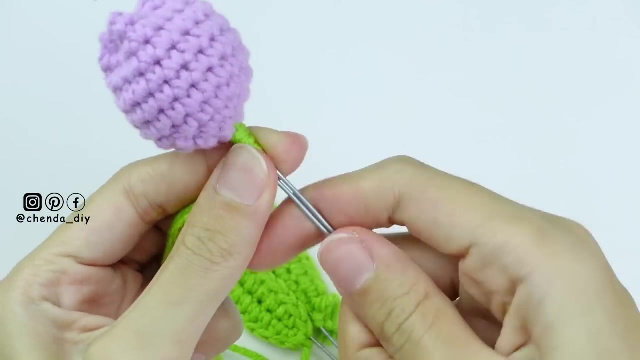 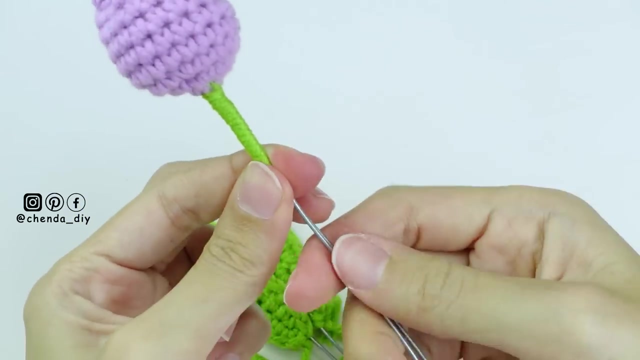 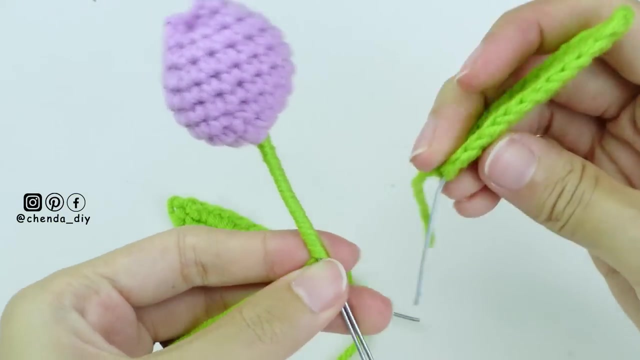 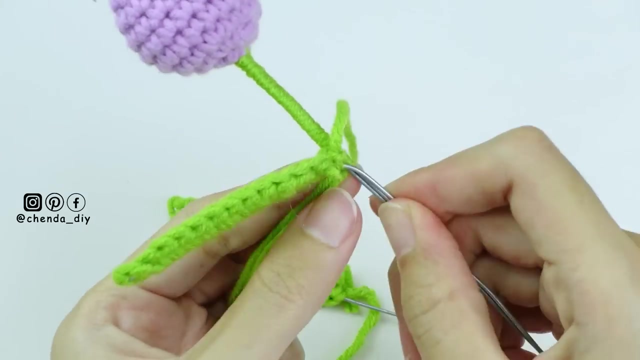 And now we are going to attach the green yarn into the bottom of the tulip. Next, wrap the yarn around the wire. Make sure that you wrap it really tight, And then, kalau you twist the twill with the twill wire, you will be able to put it back together. 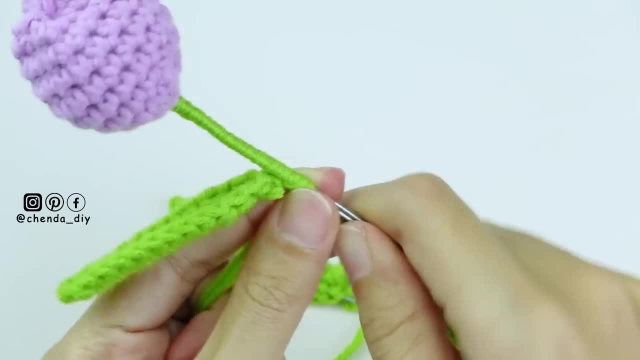 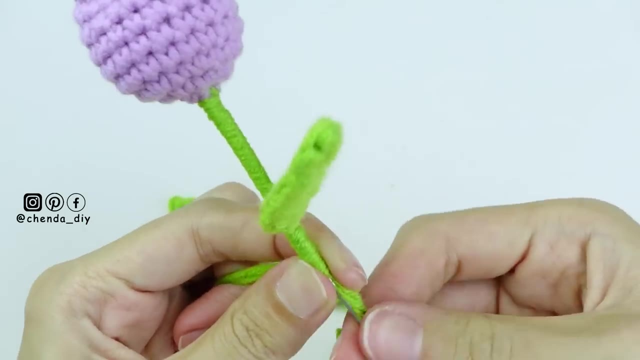 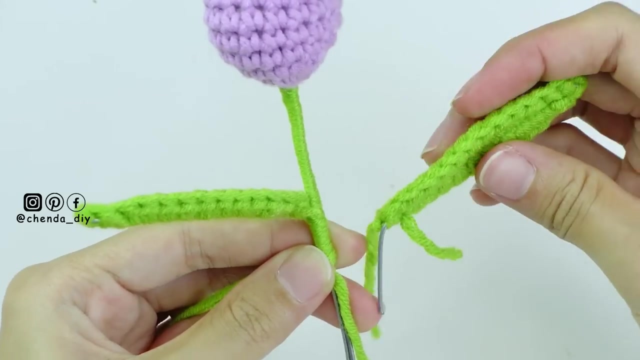 Also, if you don't have a twill wire, you can use a real one. But pues, we are going to attach the green yarn into the long loop And then make a slip stitch. You can also do this using a three way knot. If you want to do this, you can just twist the twill back and forth. 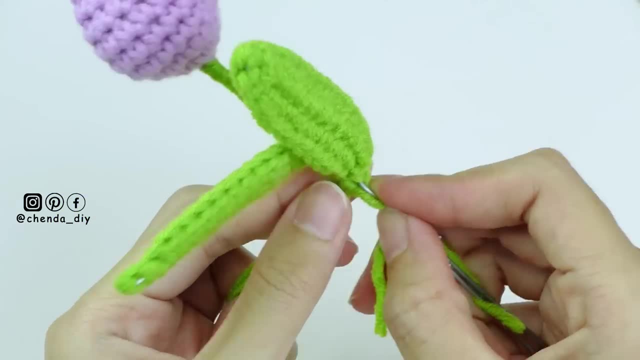 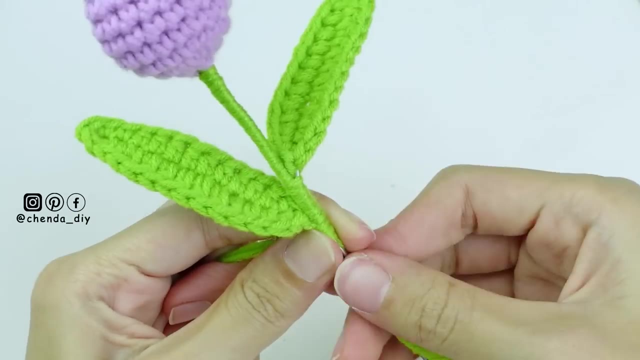 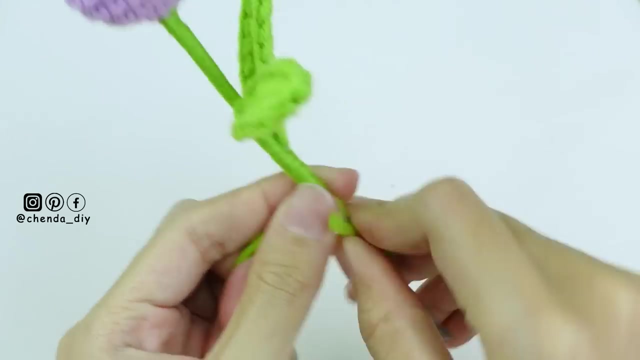 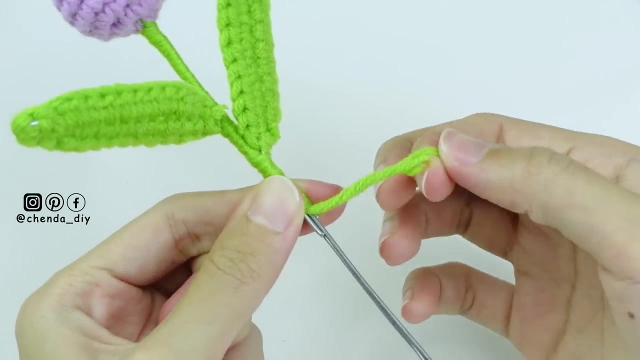 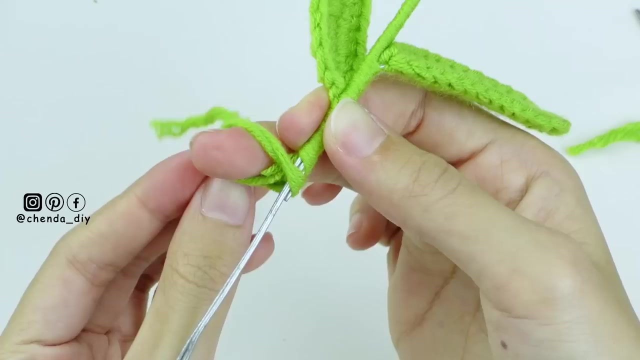 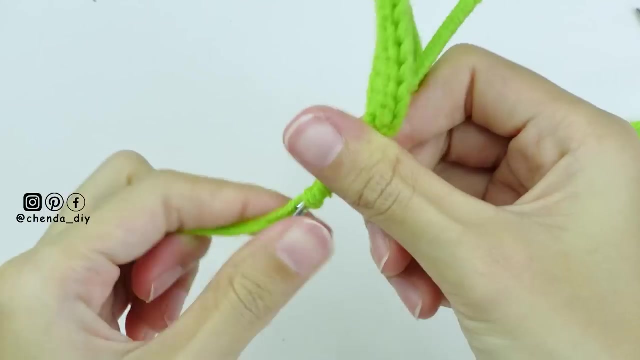 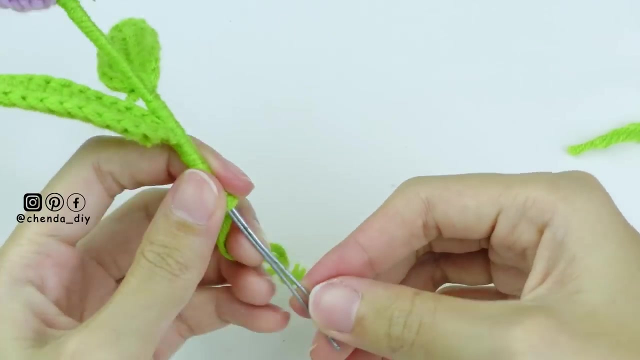 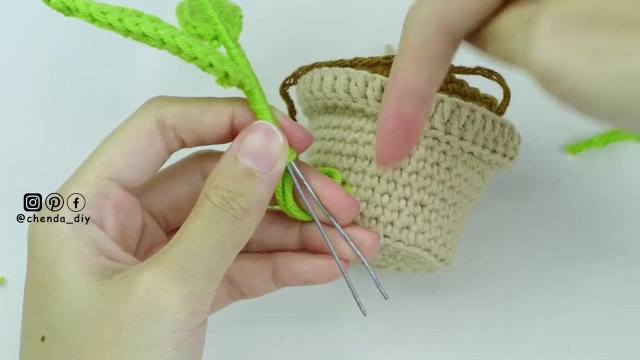 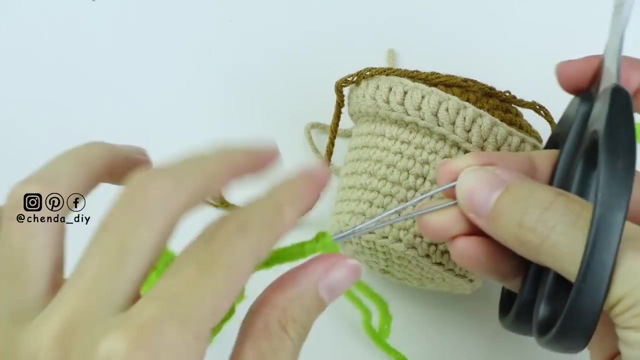 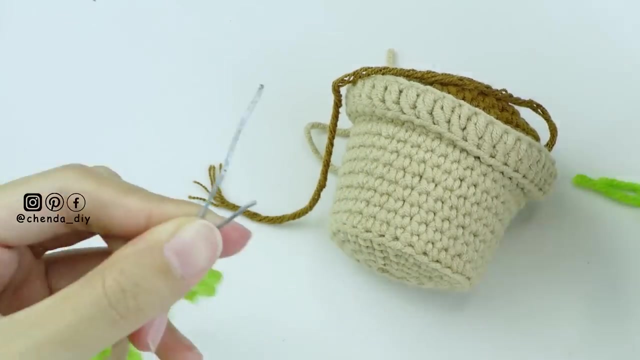 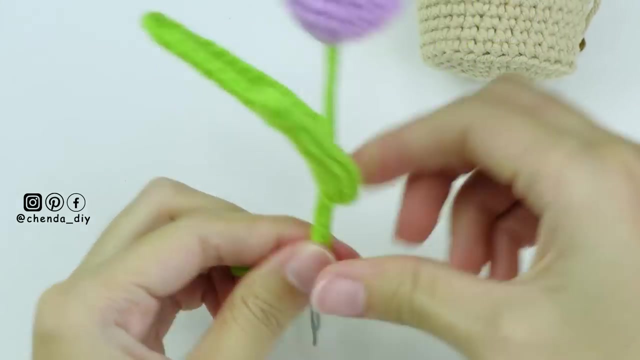 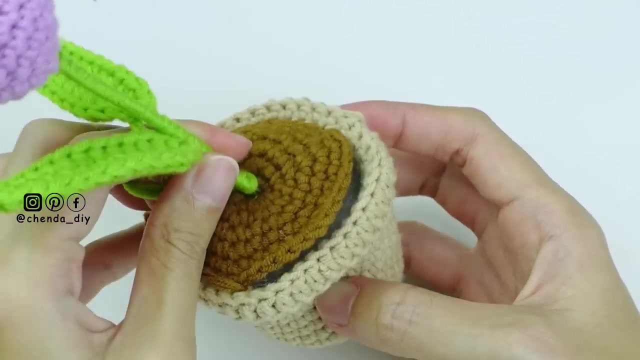 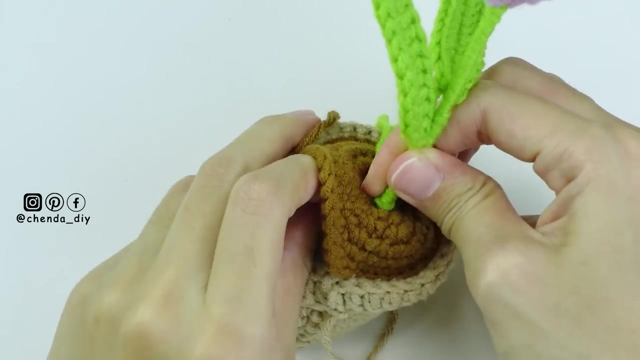 So here is how it looks like, Thank you. Next, we are going to insert the wire into the middle part of the pot and, when the wire get inside the pot, and then stretch the wire to secure it. Next, we are going to insert the wire into the middle part of the pot and, when the wire get inside the pot, and then stretch the wire to secure it. 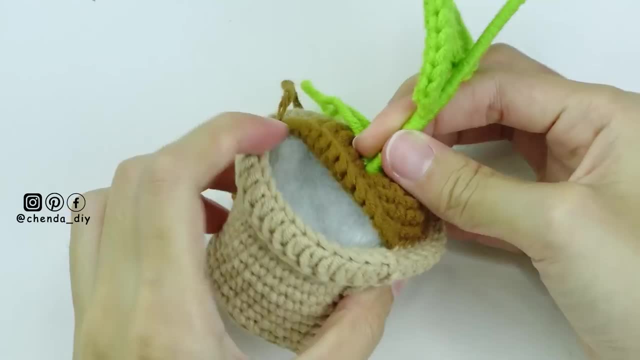 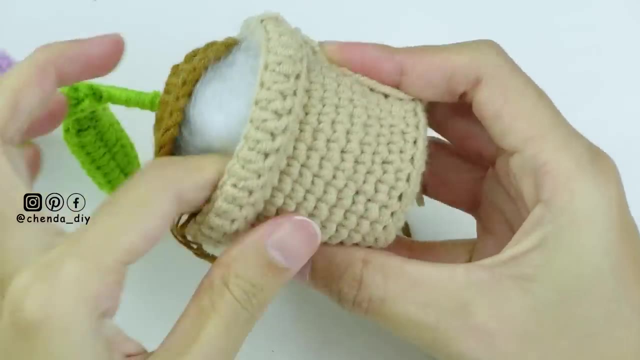 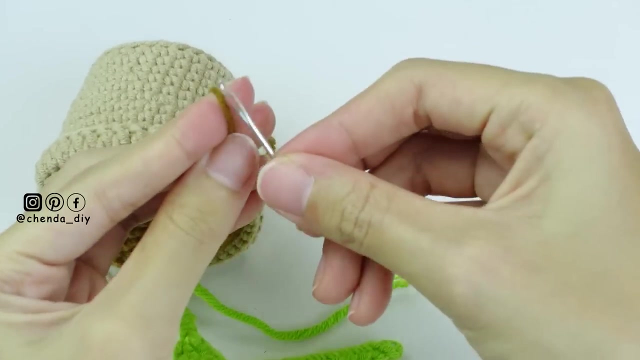 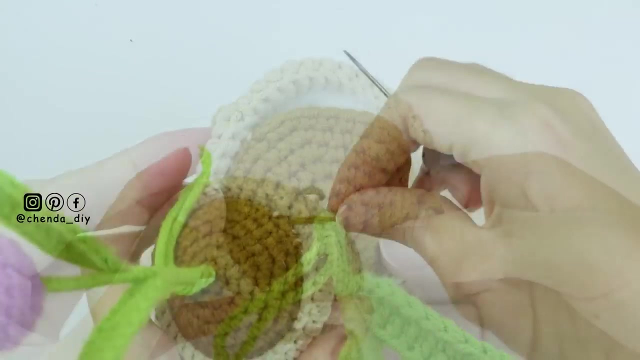 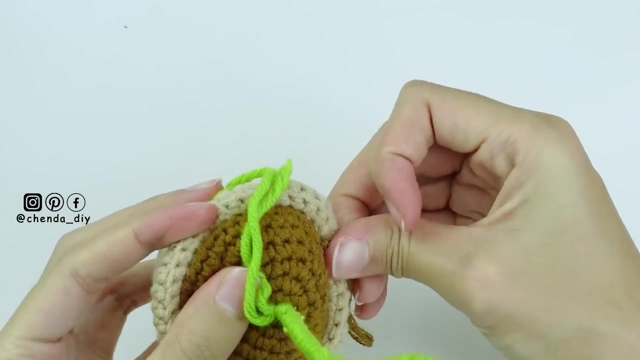 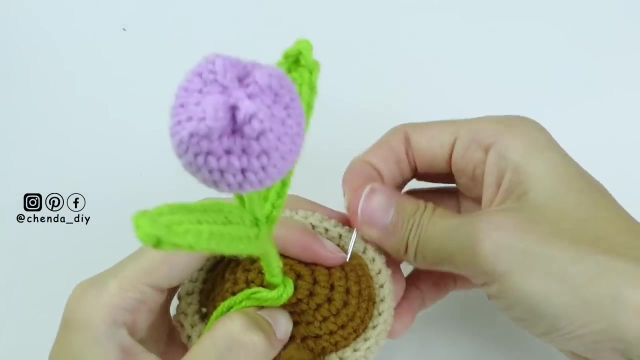 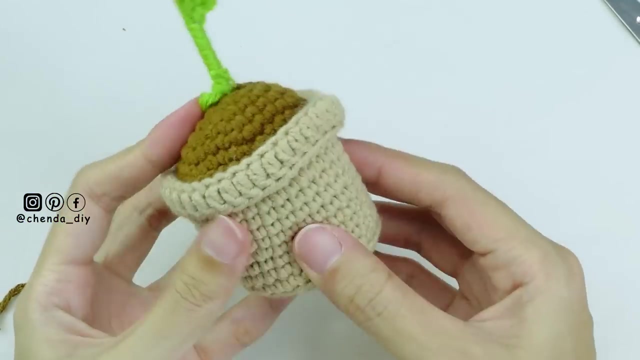 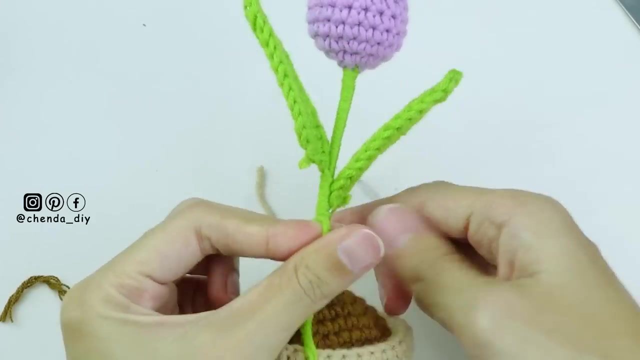 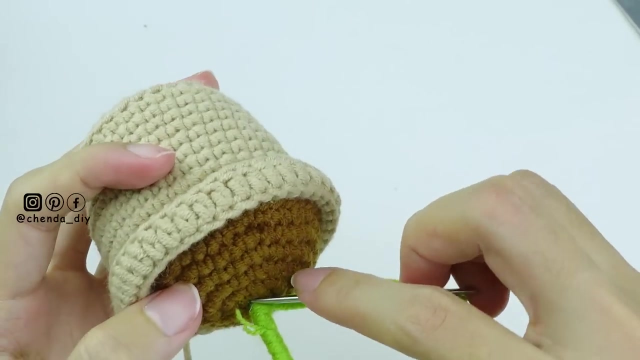 Next, we are going to insert the wire into the middle part of the pot and when the wire get inside the pot and then stretch the wire to secure it. Next, we are going to continue sewing the cover of the pot to close it. Next, we are going to continue sewing the cover of the pot to close it. 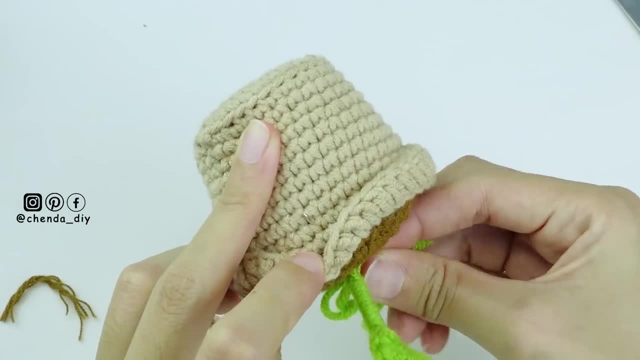 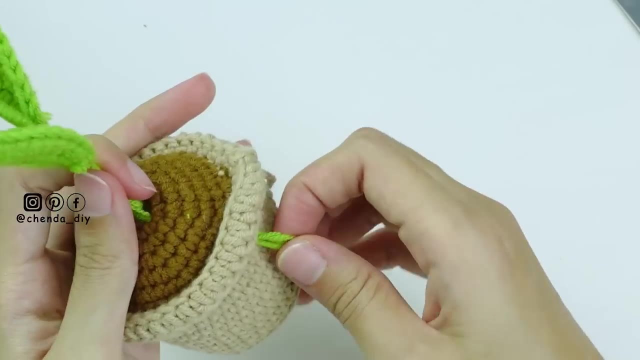 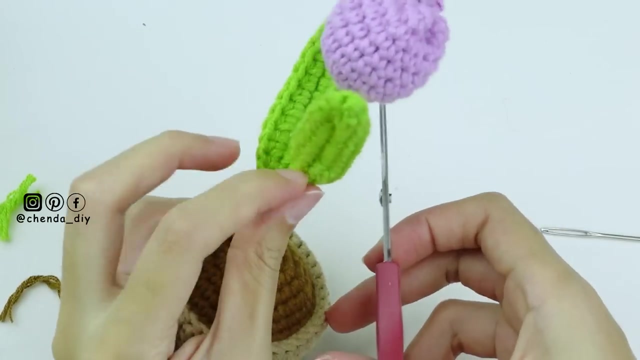 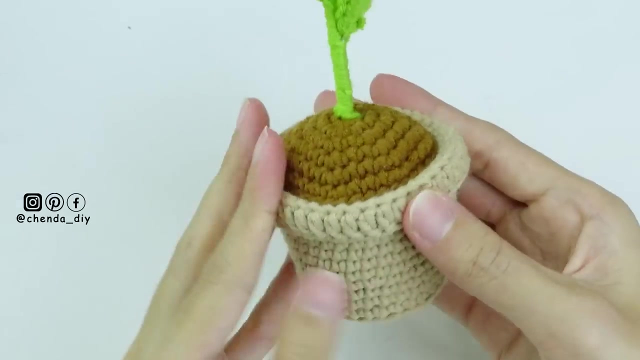 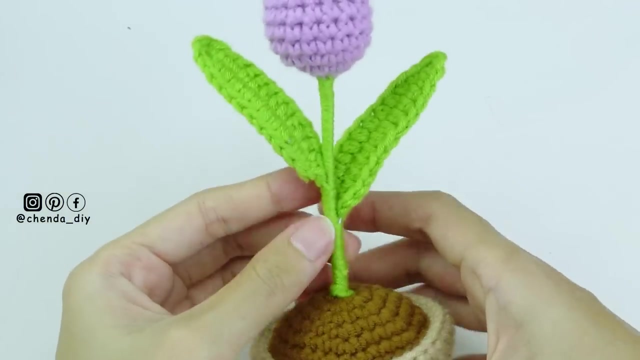 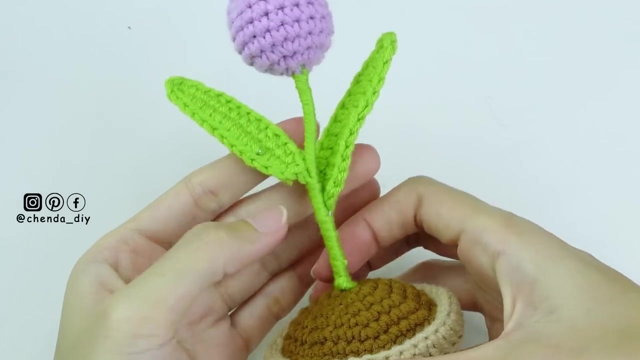 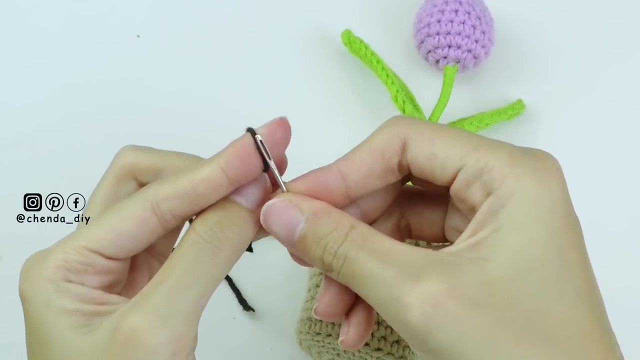 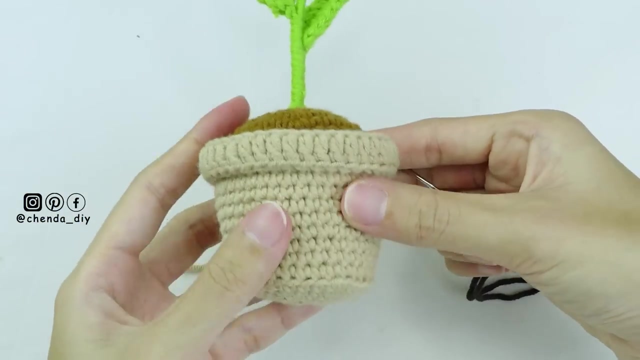 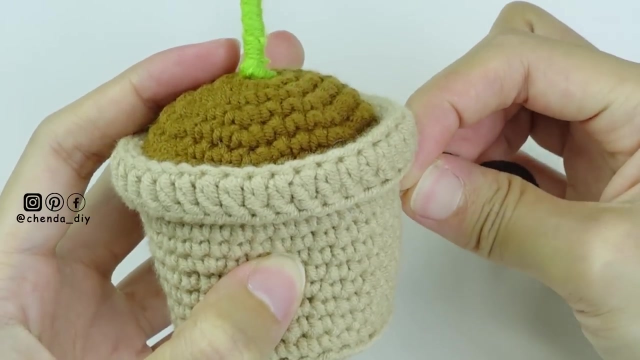 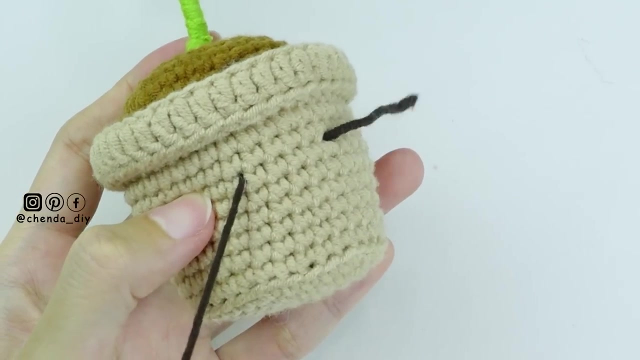 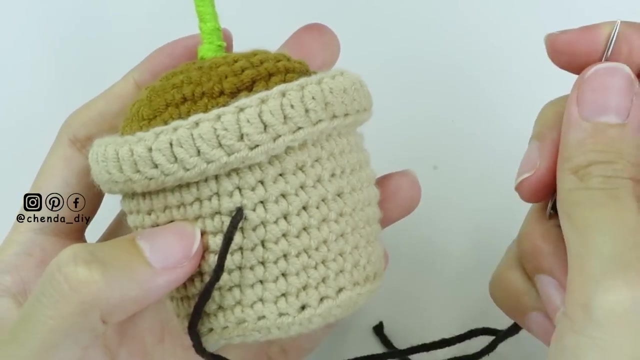 Next, we are going to continue sewing the cover of the pot to close it. And now we are done attaching the flower into the pot. Next, we are going to sewing smile emoji on the pot. Next, we are going to continue sewing the flower into the pot. 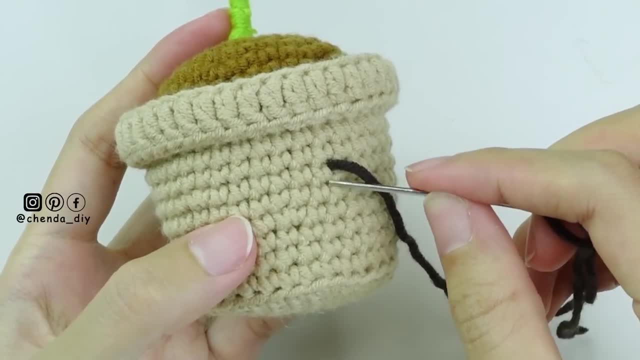 Skip one row and insert the needle into the second row at the row below, And then count two stitches at the front and insert the needle into the middle part of these two rows. And then count two stitches at the front and insert the needle into the middle part of these two rows. 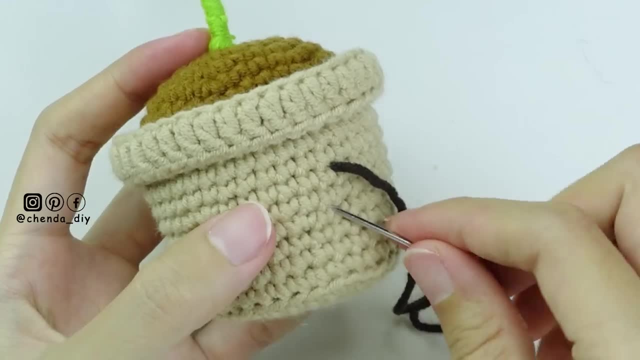 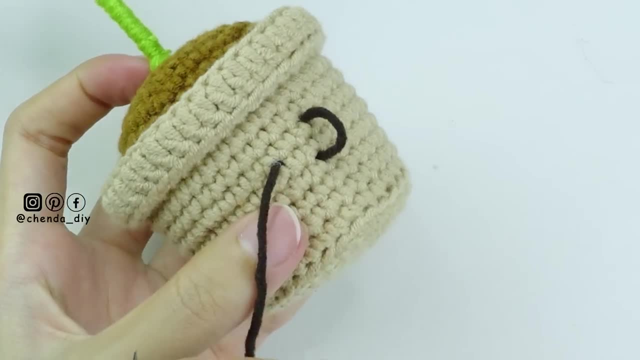 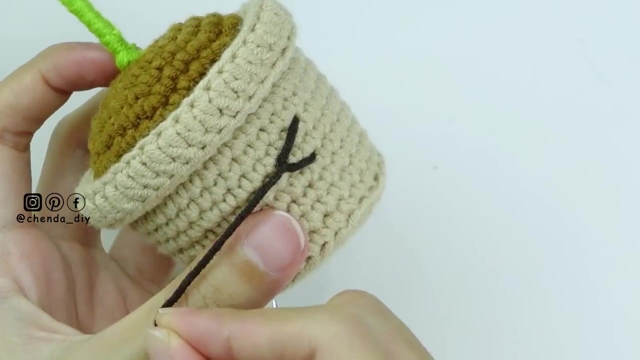 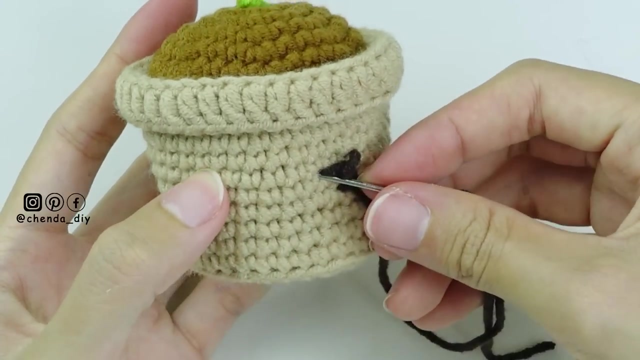 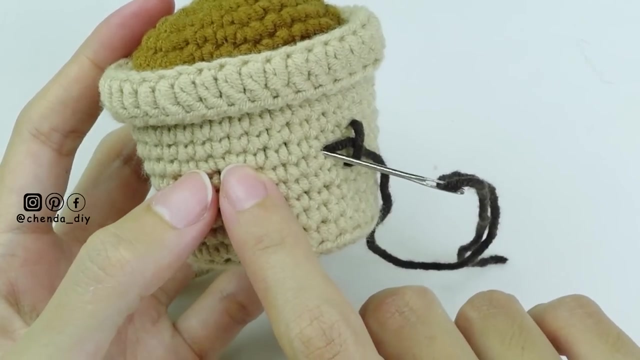 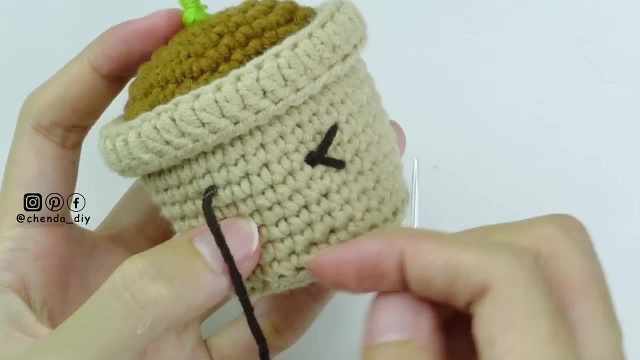 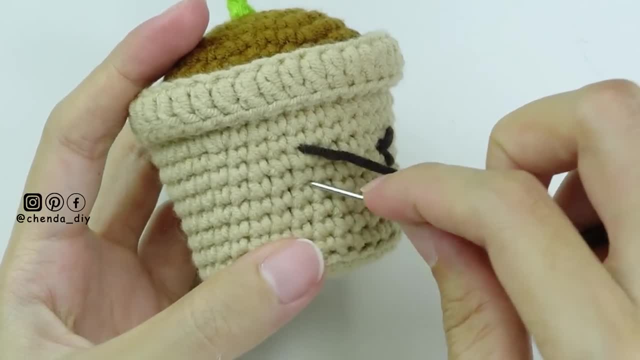